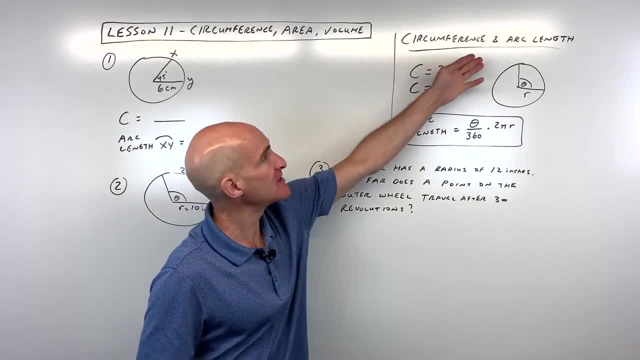 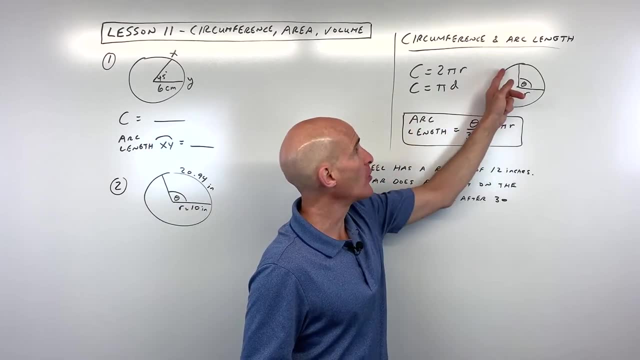 you've learned already. So first thing we're going to start off with is circumference and arc length. So remember, circumference is kind of like a fancy name for perimeter of a circle, So it's the distance all the way around that outer edge of the circle, And you probably remember circumference is. 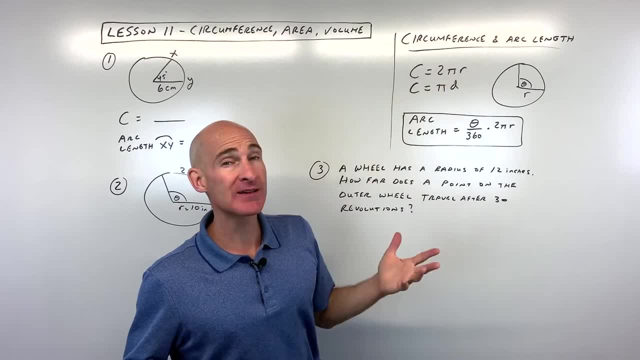 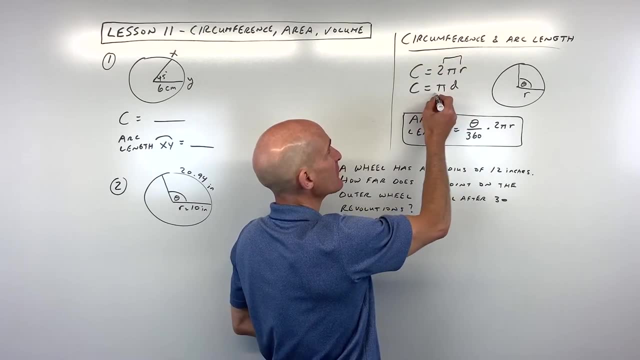 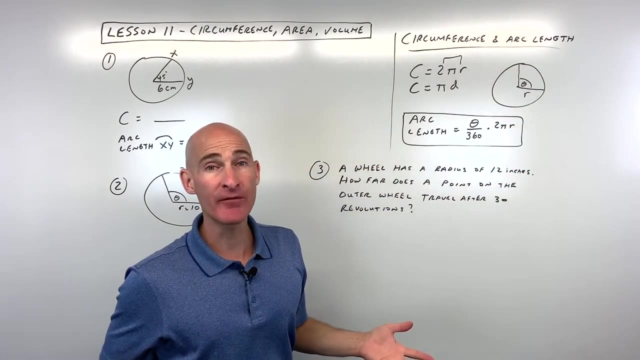 two times pi times r. Remember pi is 3.14 approximately. Or you could do see two times the radius. That's the diameter. So you could just say circumference is pi times d. Now the arc length is just a portion of the length of the circumference, right? So what you can do is you can. 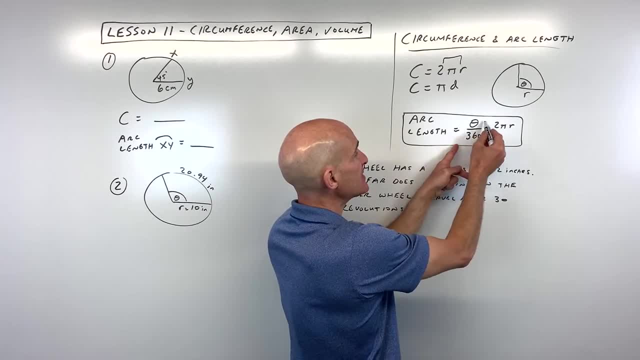 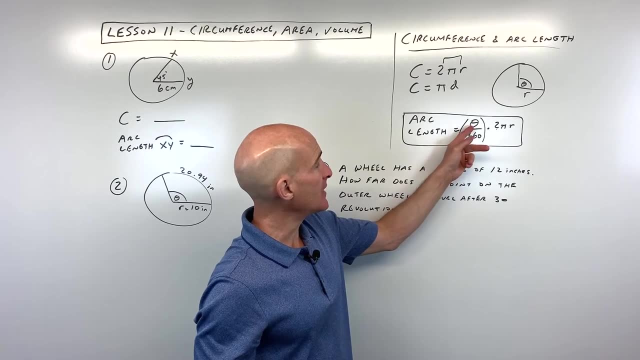 take this central angle, theta, divided by 360. And what this gives you is the fraction of the whole circumference, which is two pi r. So pretty simple. You just take whatever the angle is like. say, if this was 90, 90 divided by 360, that's actually one-fourth. 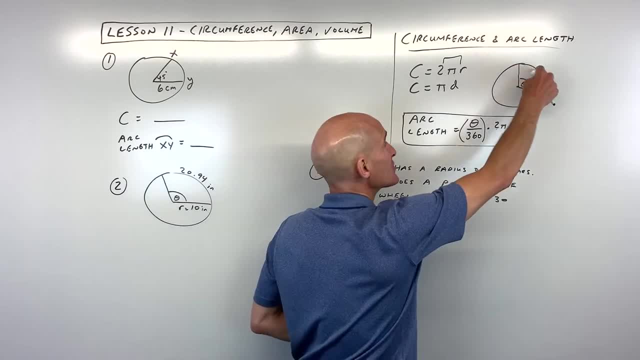 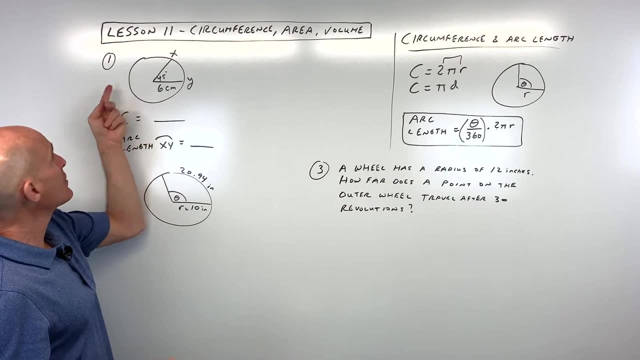 times two pi r, So one-fourth of the circumference, will give you just that portion of the circumference. That's the arc length. So let's go through some examples just to kind of illustrate. So for number one, you want to find the circumference of this circle, So we're just going to use this formula. 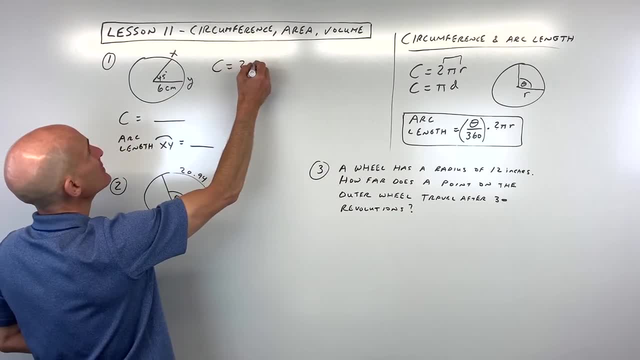 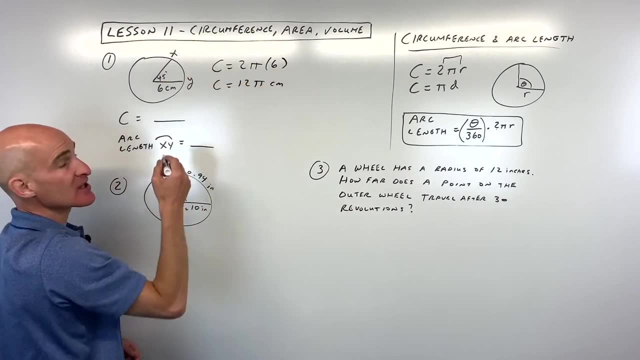 two pi r. So this is going to be two times pi, times the radius, which is six, And you can say that's going to be 12 pi centimeters. It's just centimeters to the first power. That's just length. It's just one dimensional, You can. 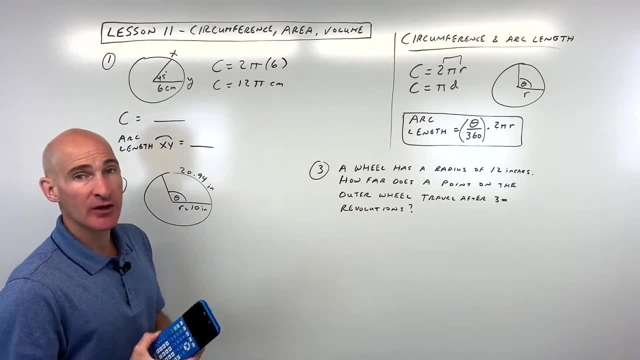 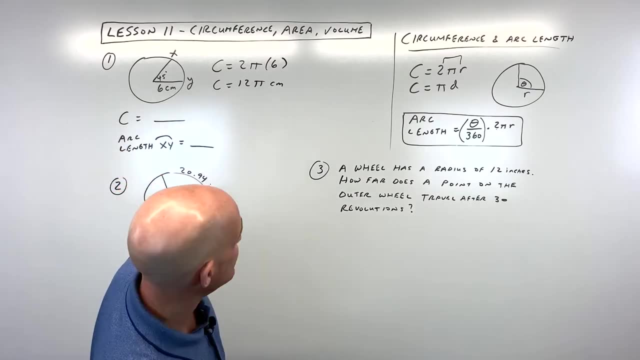 also put 3.14 in for pi, if you want to. you know, get an approximation, But this is like an exact answer, So I'll just do 12 times 3.14.. It's about 37.68 centimeters. Okay, now for the more. 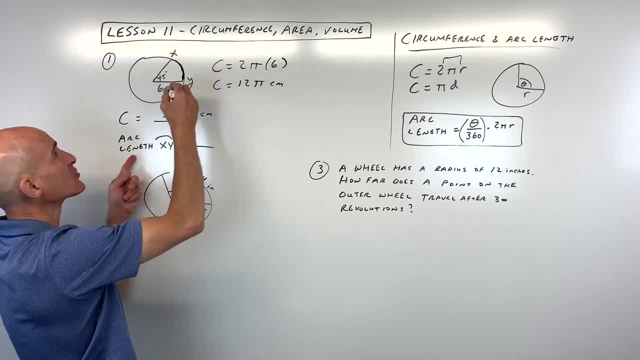 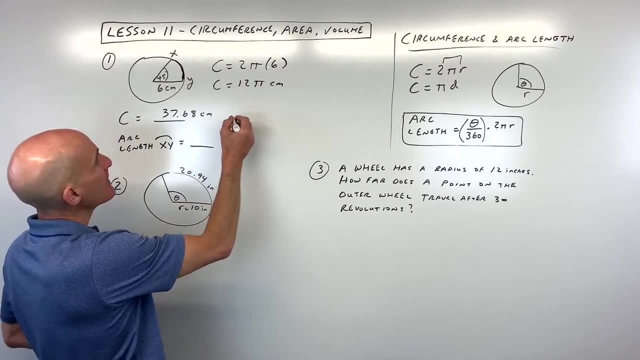 interesting one here: the arc length. What's this length right here, this curved portion of the circle? If we were to straighten it out, how long would it be? Well, you can see, this central angle here is 45 degrees. So what we have is 45 divided by 360 times the whole circumference which we 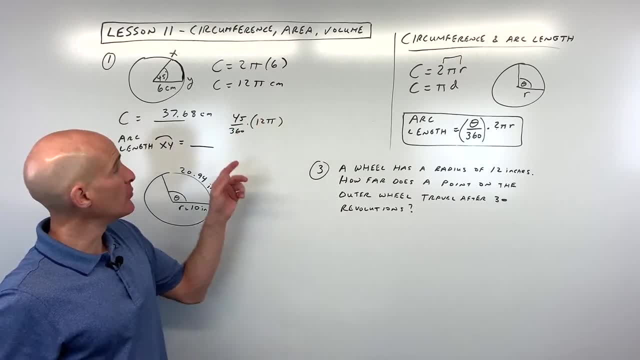 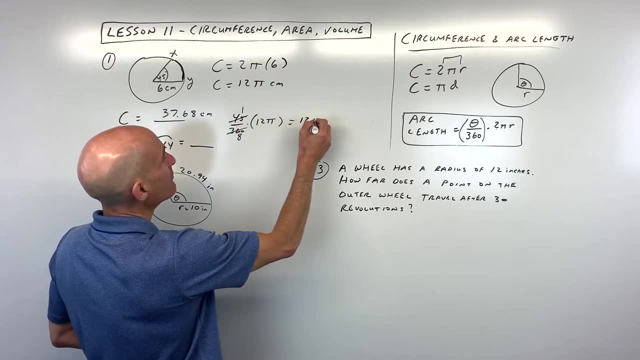 figured out was 12 pi. Now you can reduce this a little bit. 45 goes in here once. 45 goes in here eight times. So this is really like 12 pi over 8, and 4 goes in here three times. 4 goes in here. 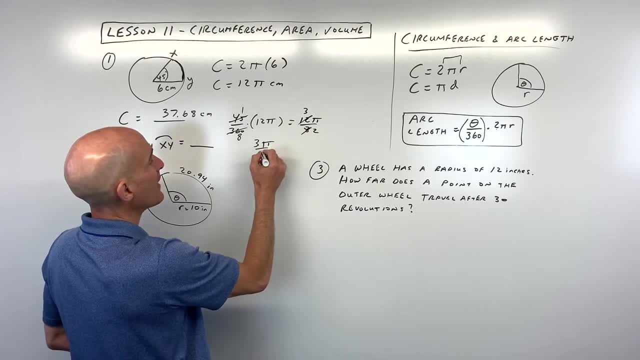 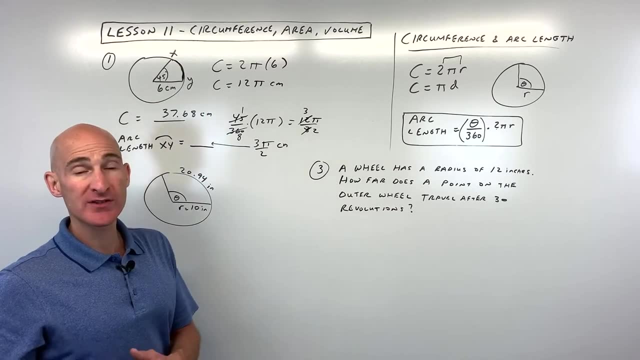 two times. So this is like an exact answer: 3 pi over 2 centimeters, and that would be just the length of the arc there. Now, if you want, you can put 3.14 whenever you see pi and get a decimal approximation. Let's go to number two now. So this one is a little bit different. 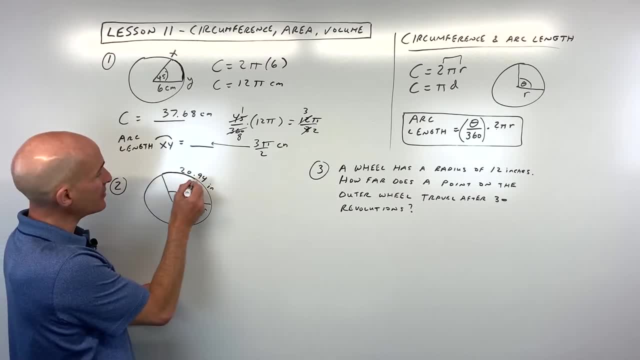 because we're working backwards. So they give us the arc length, see right here, 20.94.. But how do we find that central angle? Is it 90 degrees? Is it, you know, 60 degrees? Is it 65 degrees? So, 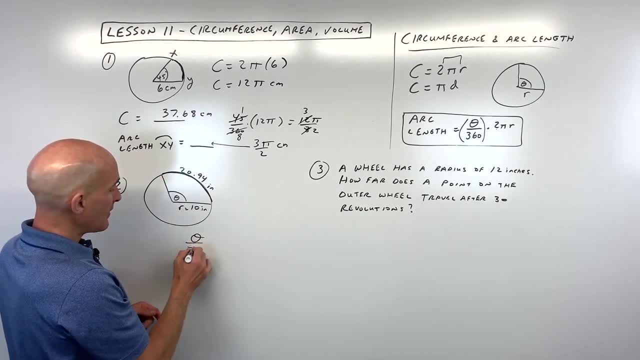 again. let's use our formula here. We have theta divided by 360 times the circumference, 2 pi r r is 10 centimeters. So we have theta divided by 360 times the circumference, 2 pi r r is 10. 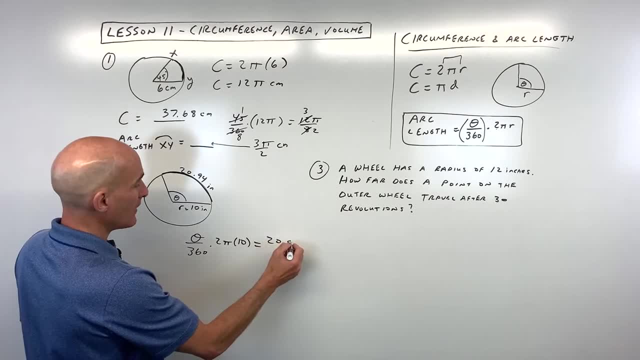 centimeters. So we have theta divided by 360 times the circumference, 2 pi r, r is 10 centimeters. So that's going to give us our arc length, which is 20.94.. Okay, so now let's see what we can do here. 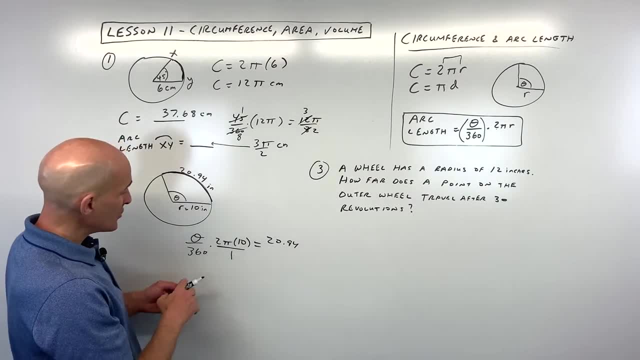 This is like over 1, anything divided by 1 is itself. So what I'm going to do is- I'm going to simplify a little bit here- I'm going to multiply the numerators together, the denominators together, and I'm going to divide. So 2 times pi times 10, and you can use the pi key on your calculator. 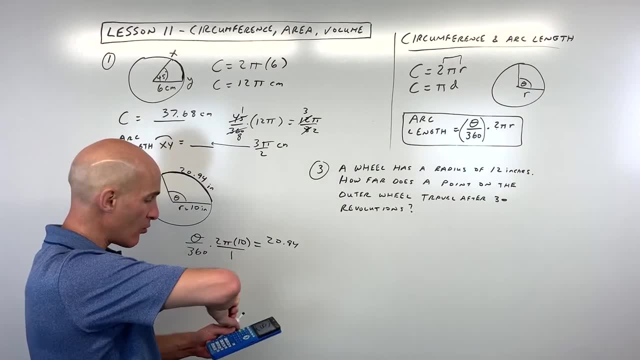 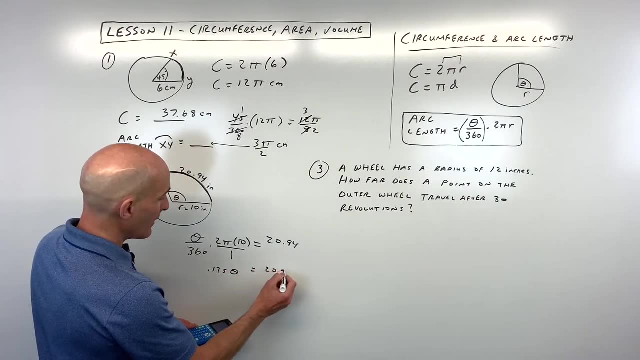 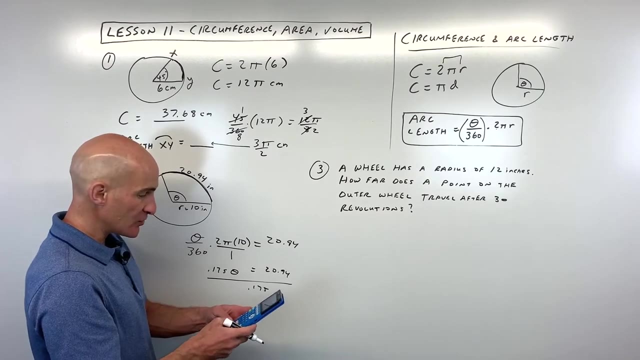 I'm going to divide that by 360, and this comes out to 0.175 approximately times theta, which is equal to 20.94.. Now if we divide both sides by 0.175, you know we can get theta by itself. So let's go ahead and do that. So I'm. 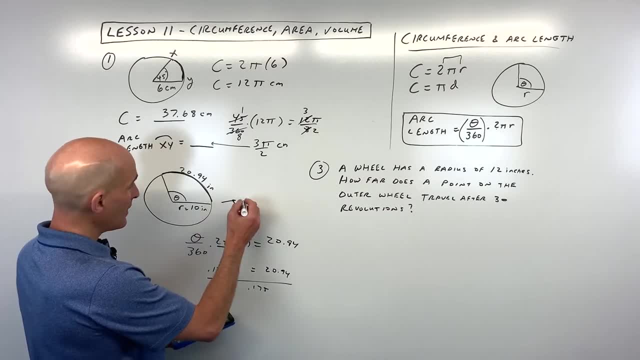 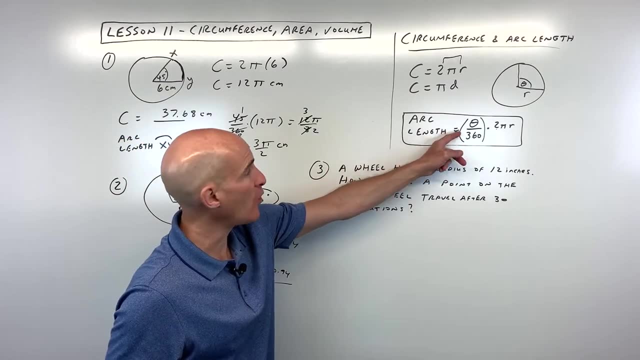 getting about. I'm just going to round to the nearest degree. it's about 120 degrees And you can double check your work on this. just go back and put 120 over 360. that's 1 third of the circumference, 2 pi times 10.. Okay, let's. 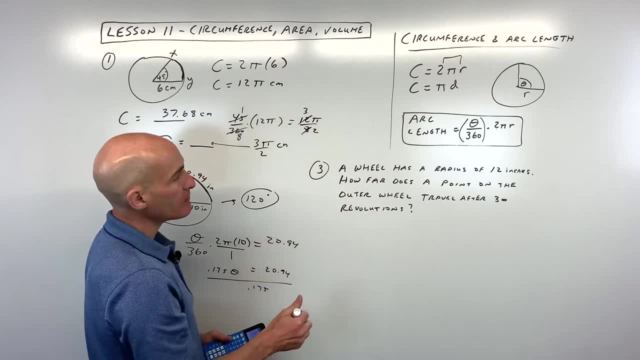 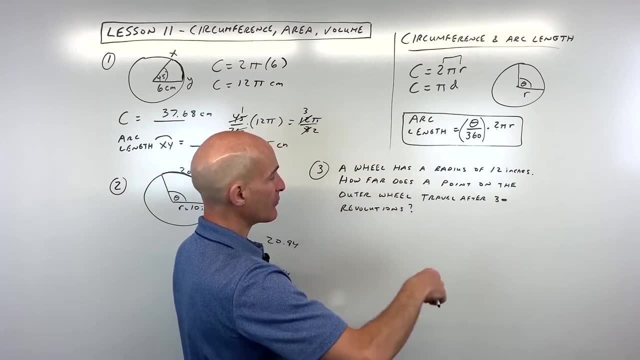 go to number three. now, this one's a little bit different, kind of like a word problem. It says a wheel has a radius of 12 inches. how far does a point on the outer wheel travel after 30 revolutions? So just this is kind of. 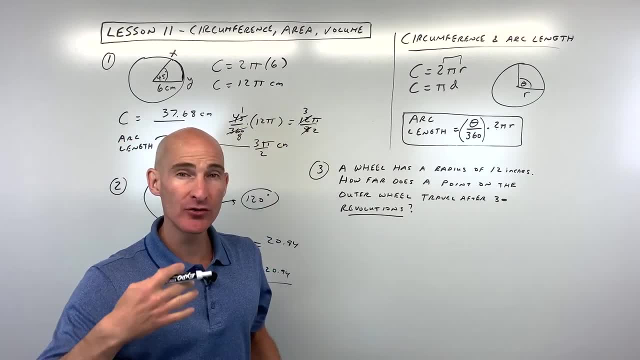 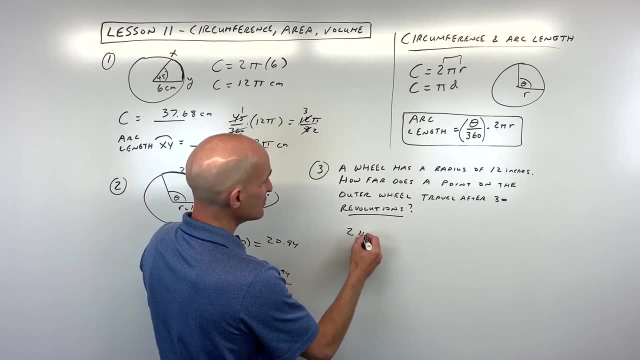 interesting because when they say revolution, sometimes that throws students off. Revolution is just like one circumference, one distance around that outer edge. So really what we're doing is we're really doing the circumference 2 pi times the radius 12. that's one revolution or one rotation, but we're 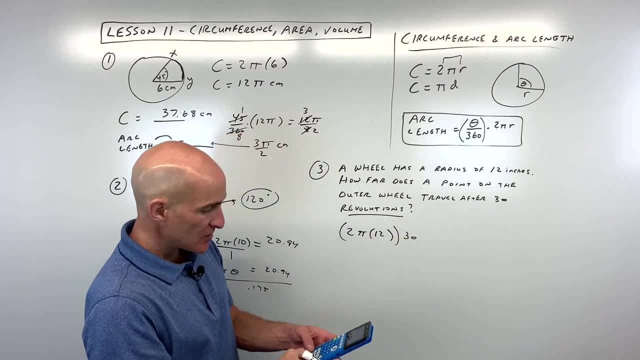 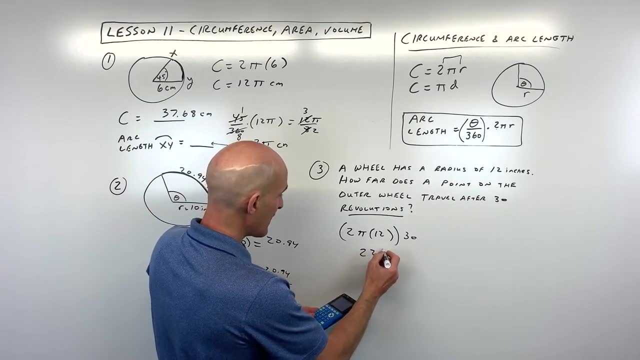 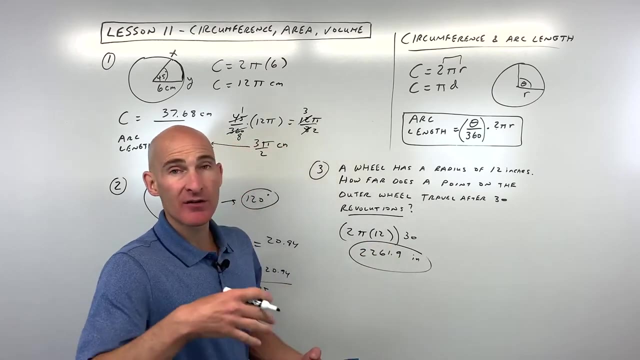 going to multiply that by 30. Since we have 30 revolutions, So let's do that on the calculator. I'm using the pi key here to get a little bit more accurate. So it's coming out to 2261.9. let's see, that's inches, And sometimes we'll ask you to convert it to feet, or 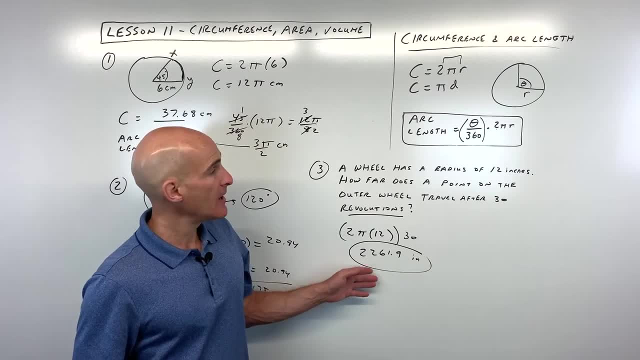 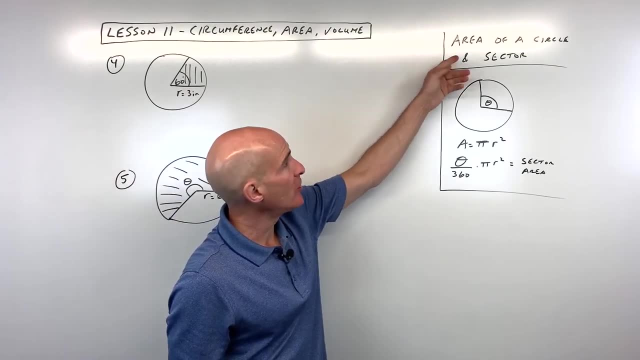 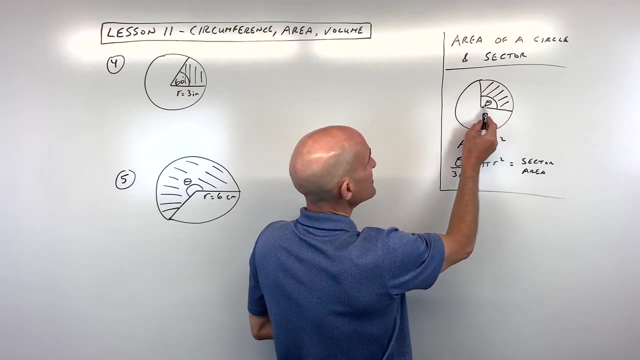 to miles or that sort of thing. that's more of like a dimensional analysis. but again, here we're just working with circumference and multiples of those. Okay, now let's talk about the area of a circle and the area of a sector. A sector is like a section of the circle, so, for example, like here you can see, this is: 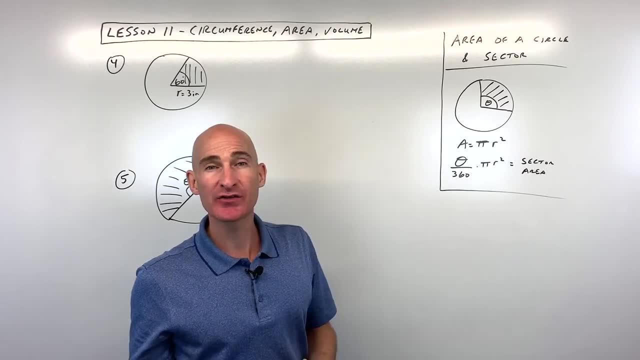 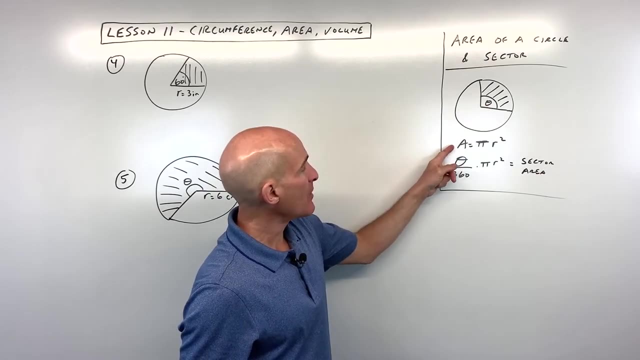 our central angle, theta, and by the way you know, you can use Greek letters for these angles, like alpha, beta, gamma, theta. So here I'm just using theta. You can call it X if you want, but you probably remember from a previous course the area. 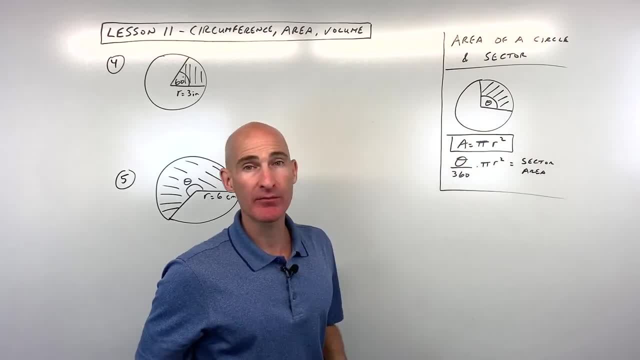 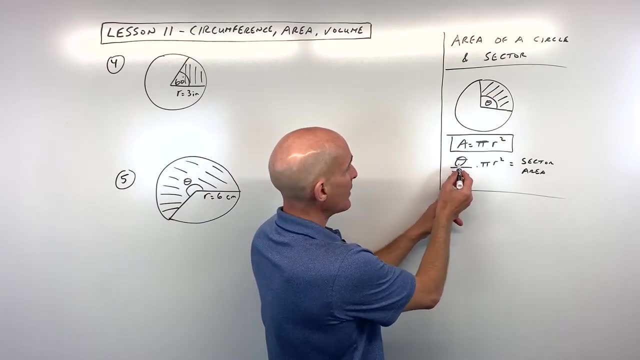 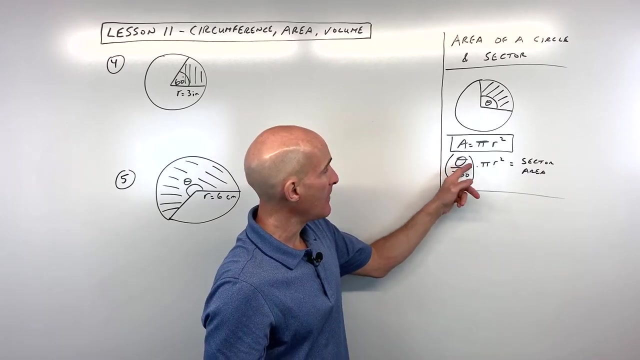 of the whole circle is pi times the radius squared. So pi r squared. But when you want to find just the area of that section or that sector of the circle, you take the central angle, theta divided by 360.. that gives you the fraction of the whole circle pi r squared. So it's just pi r squared, but you're 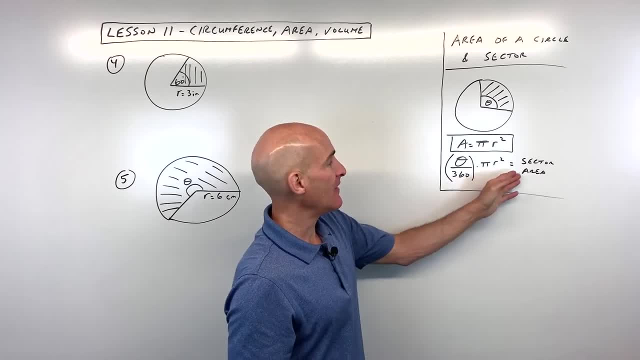 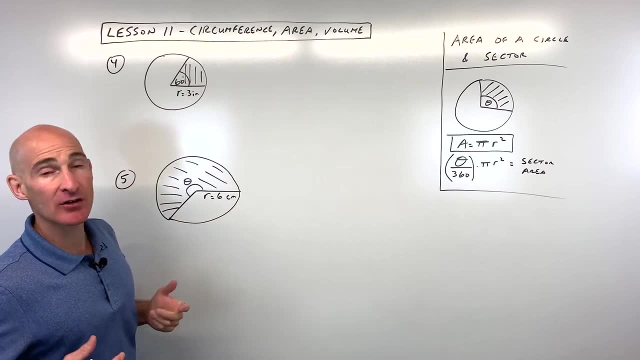 taking that fraction of of usually means times, and that'll give you just the portion of the circle that you want. So let's look at a couple examples. For number four, if you want to find the area of that sector, how would you do that one? Well, let's see, our central angle is 60, so we have 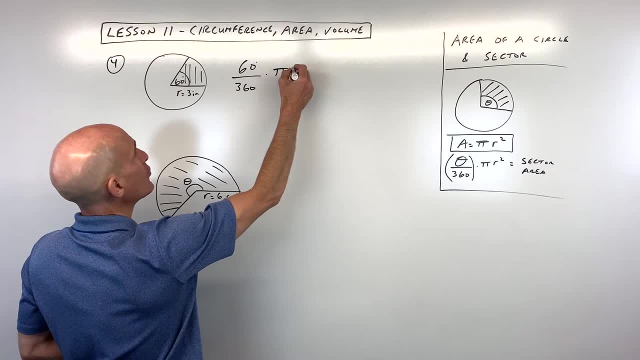 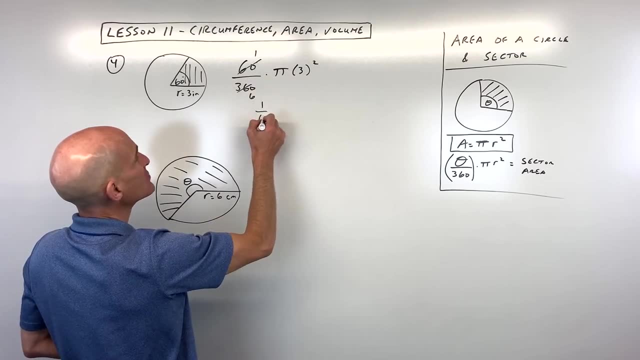 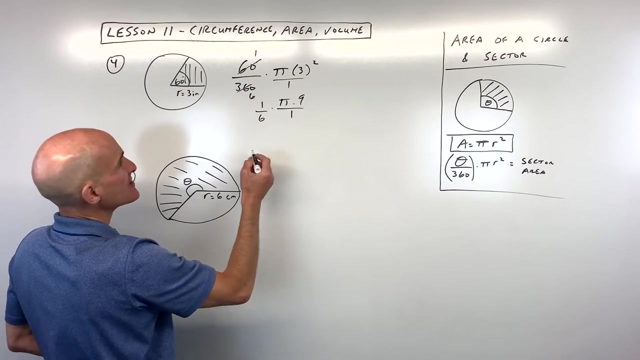 60 divided by 360 times the area of the whole circle, which is pi times three squared. This you can reduce a little bit. 60 goes in here one, 60 goes in here six times. so we have one. six times three squared is nine. so pi times nine, Anything divided by one is itself. so you can always make 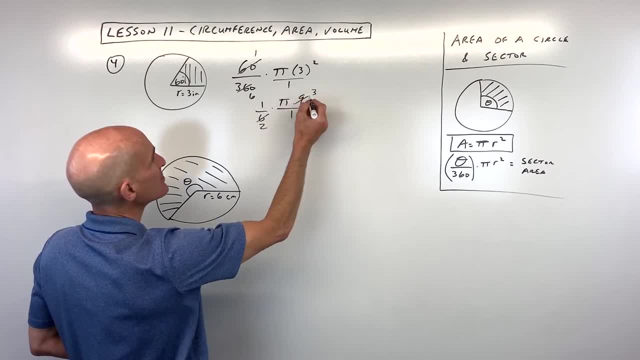 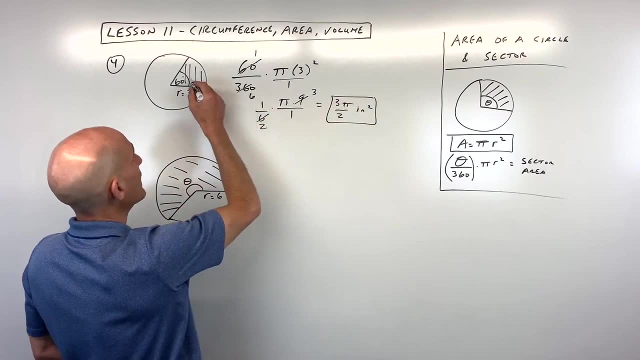 it into a fraction and let's reduce a little bit. three goes in here two times, three goes in here three times, so it's going to be three pi over two inches squared. Remember, with area it's two dimensional right, like length and width, and this is an exact answer. again, you can put 3.14 in for 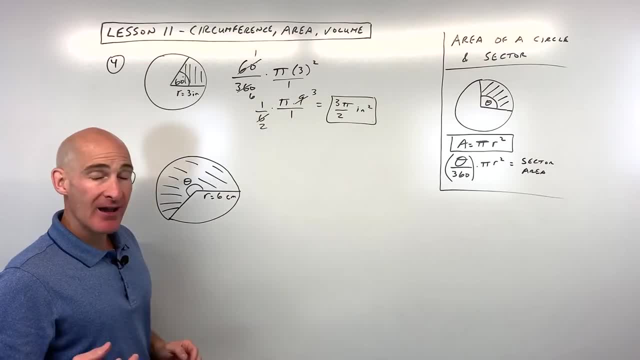 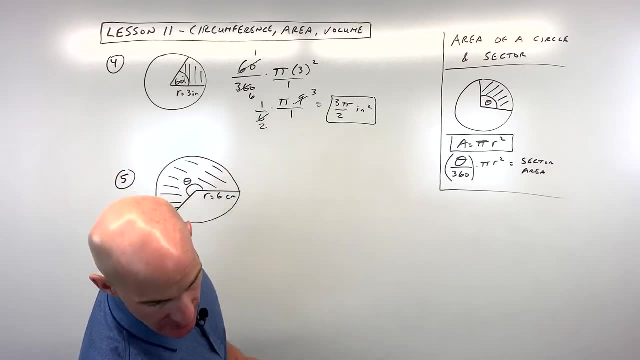 pi if you want to get a decimal approximation, Number five. this one's a little bit more challenging because we're working backwards. we want to find out what is that central angle. The area of the sector here is 70.69 centimeters squared. So let's go ahead and use our formula and let's put in what we know. So we have theta divided. 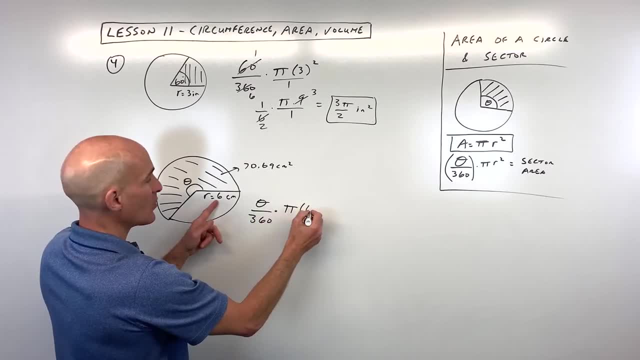 by 360 times pi, times the radius squared, that's going to be six. squared equals the area of our sector. seventy point six, nine, Okay. so now we're going to look at the area of our sector and we're going to use our formula and let's put in what we know. so we have theta divided by 360 times pi, times the radius squared, that's going to be six. squared equals the area of our sector. seventy point six, nine, okay. so 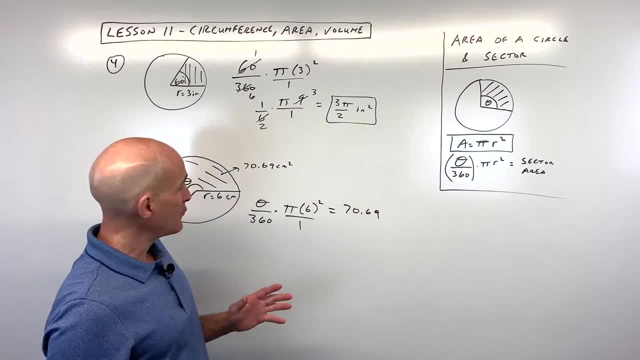 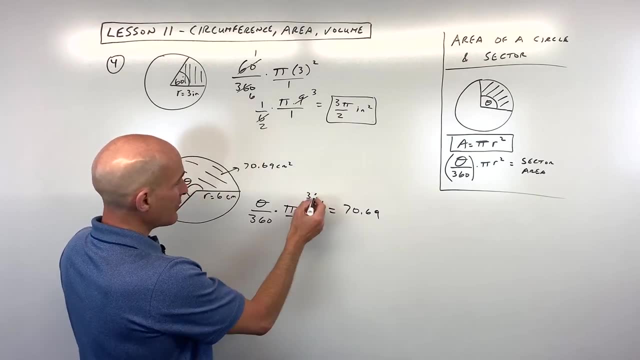 now again, we can think of this as being over one. you can do this in steps if you want, but here what I'm going to do is I'm going to say: six squared is thirty-six, so let's just do that. so that's thirty-six, and thirty-six goes in here once, thirty-six goes in here ten times. so what we have 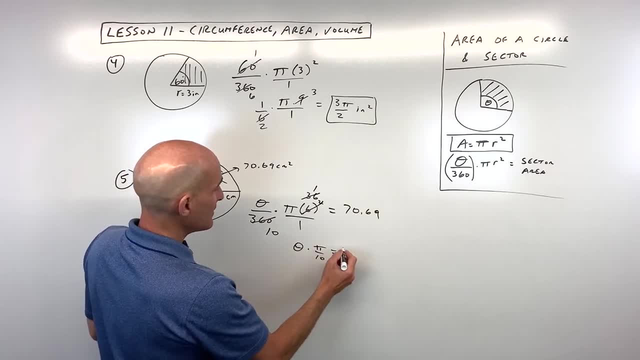 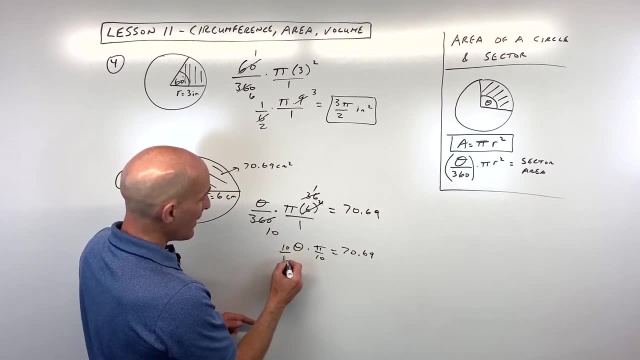 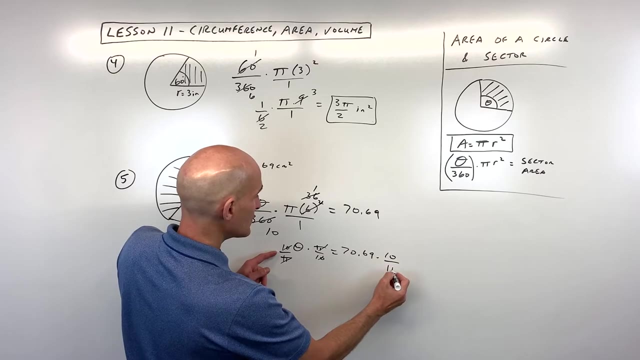 is theta times. pi over ten equals seventy point six, nine. To get theta by itself, we can divide by pi over ten or multiply by the reciprocal ten over pi. that way the numerators and denominators can't. but whatever you do to the left, you have to do to the right. So let's go ahead and see what that. 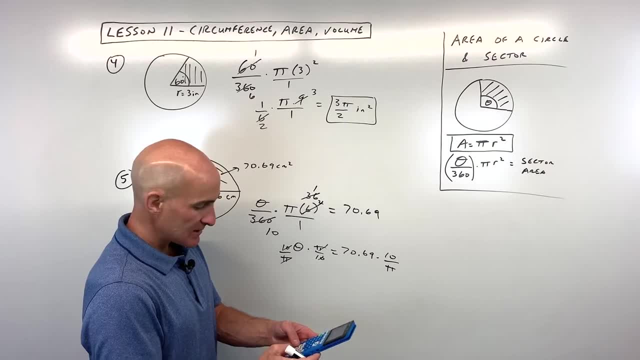 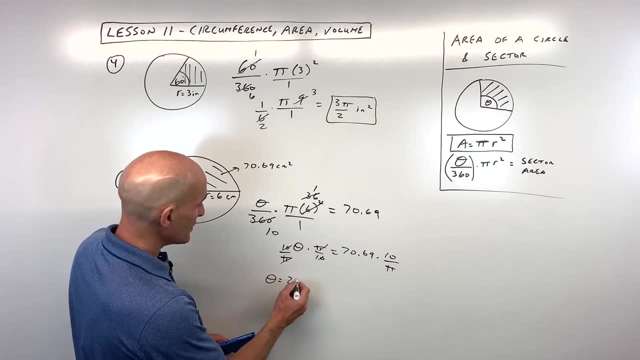 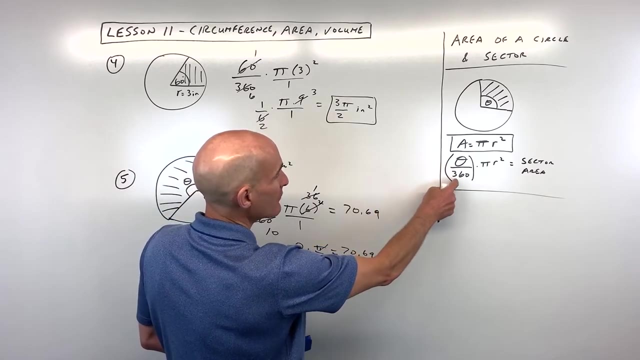 comes out to, We have 70.69 times 10 divided by pi, So it looks like it's approximately- I'm rounding here to the nearest degree- 225 degrees, And again you can check your work by just putting it back in: 225 over 360 times pi, times 6 squared, and you should get the sector. 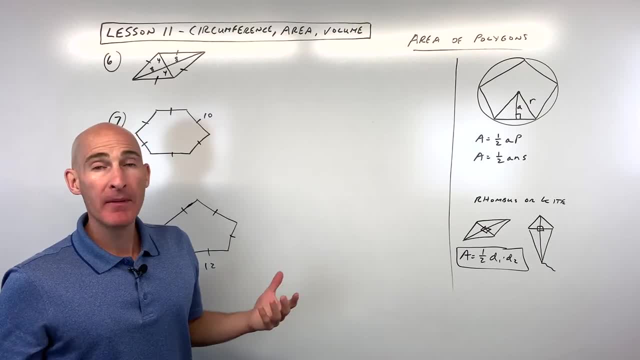 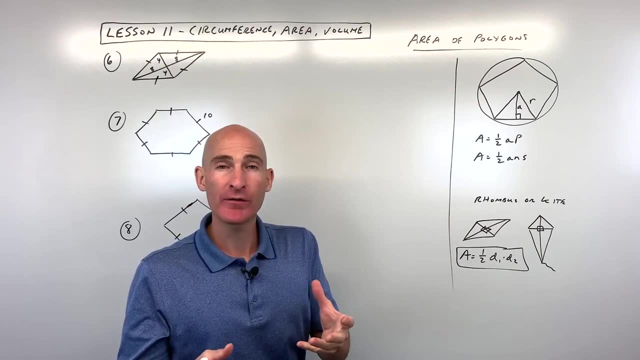 area of 70.. Okay, now let's talk about area of polygons and, specifically, area of regular polygons. And when you talk about a regular polygon, what you're referring to is that all the sides are the same length, all the angles are the same measure, and there's a nice formula that we can. 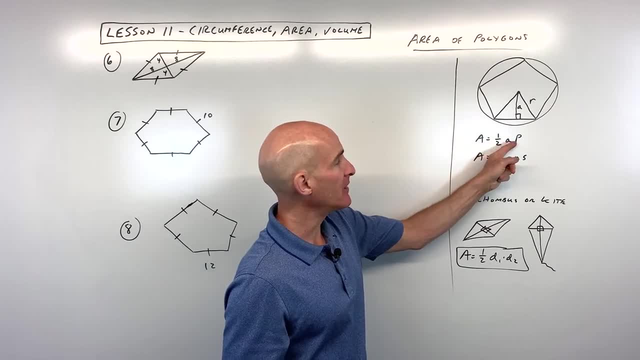 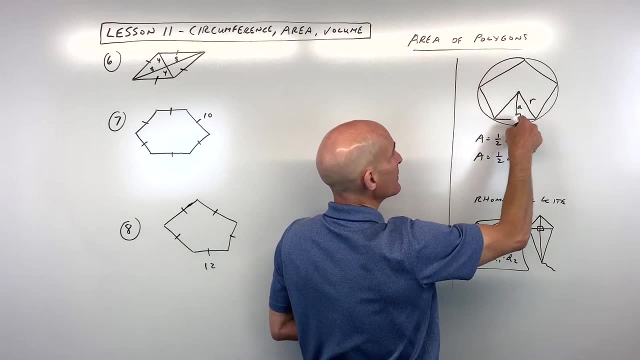 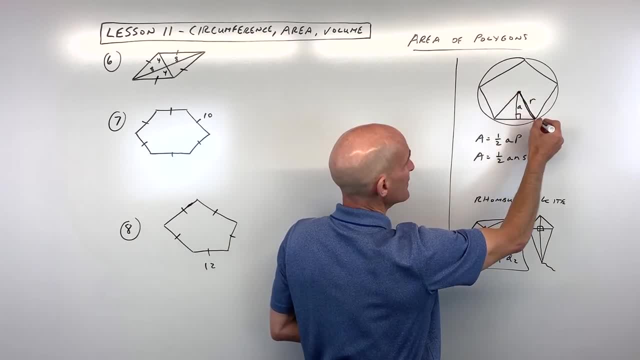 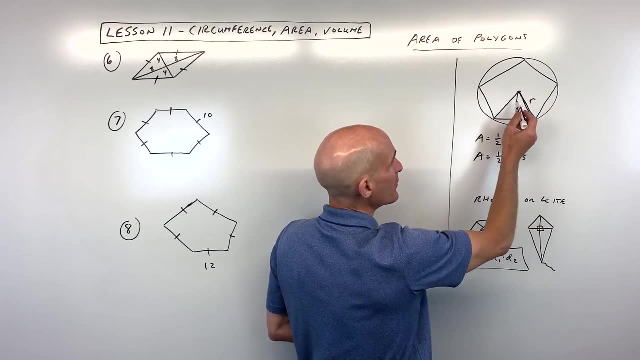 circle is That's going to be from the center of the circle to the edge of the circle. But you'll also notice that these vertices, they lie right on the the circle, So there's your radius there. Now the apothem is the perpendicular distance, or the shortest distance from the center of that circle. 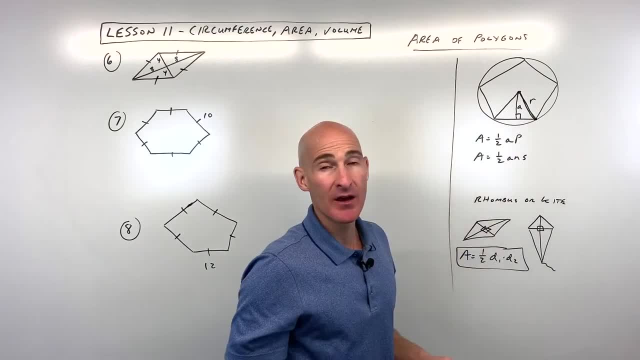 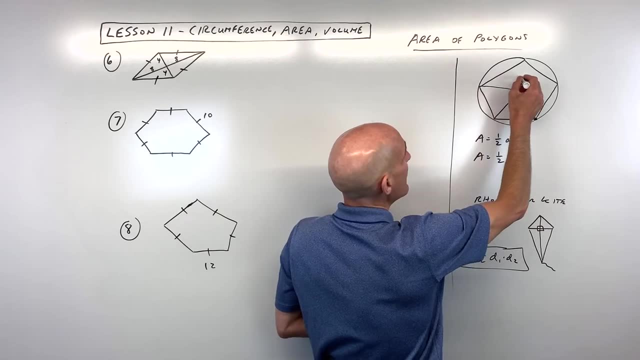 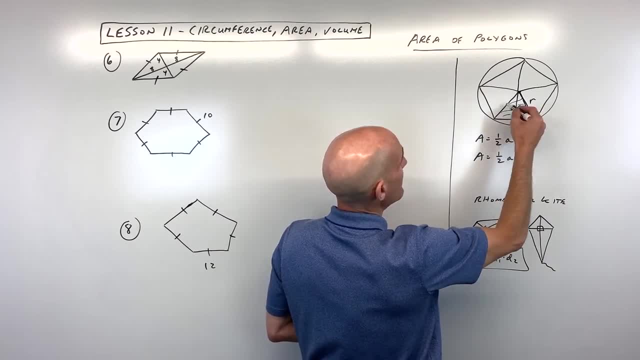 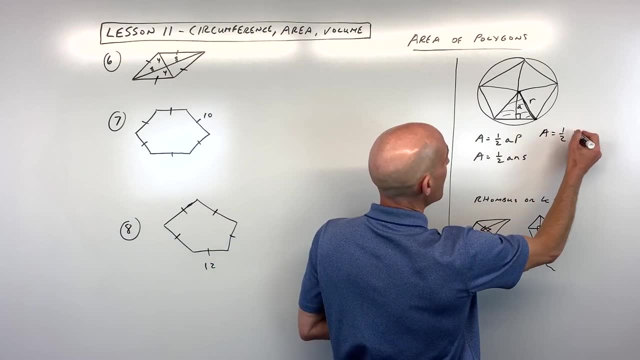 area of one of these triangles, okay, and then multiply by how many you have. In this case you have five. So when you think of the area of a triangle, remember the formula for area of a triangle: one half base times height. right, This is the base here. Now, if you were to take that area, 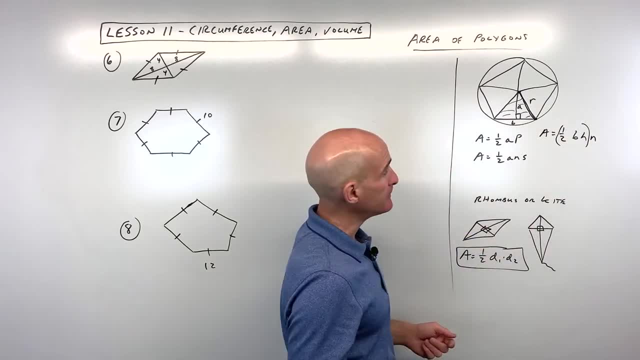 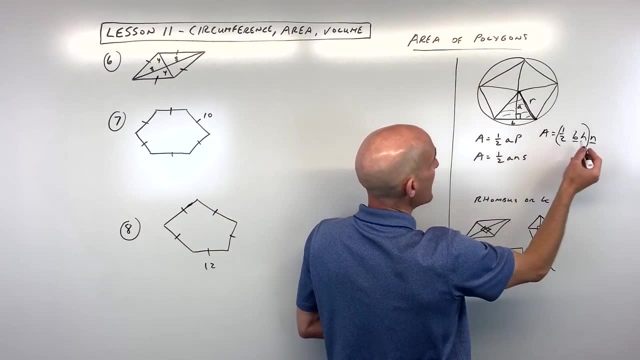 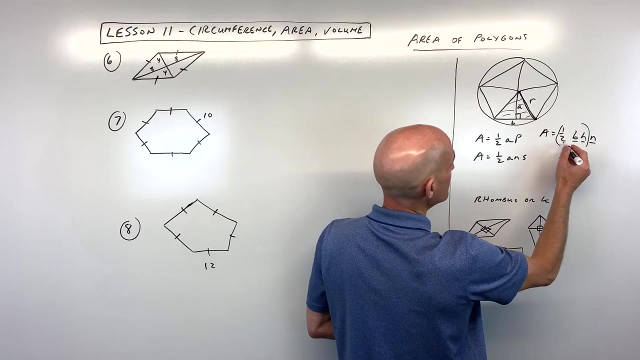 that triangle multiply by how many you have. let's just call that n. You can see this base b times the number of triangles. that's going to be like the number of sides. b times n is actually the perimeter, The height of the triangle. we said that's a, that's the apothem, and then here's your. 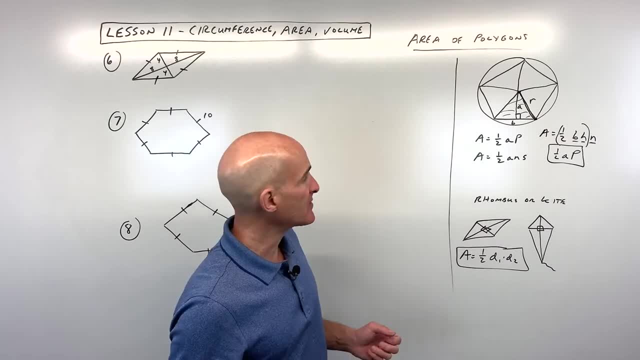 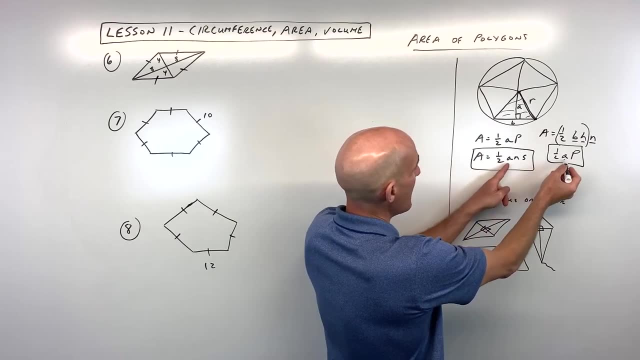 one half. So that's where the formula comes from: one half apothem times perimeter. Now another way to do this is to use this formula. Some students like this: one half a and s. Here's your apothem, but the number of sides times the length of a side is your perimeter. So either one you can. 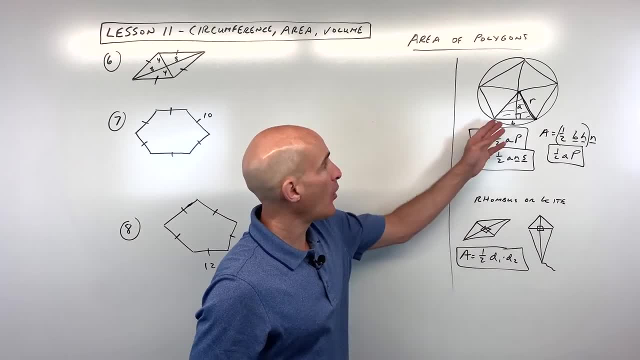 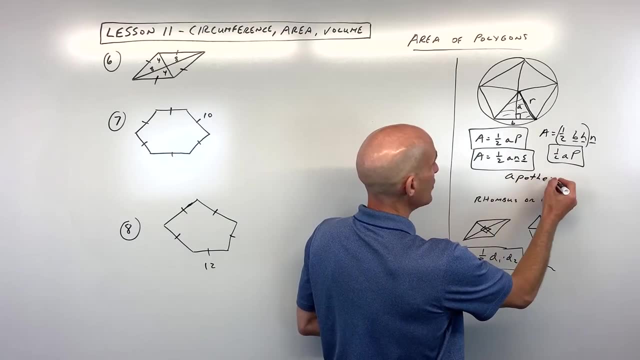 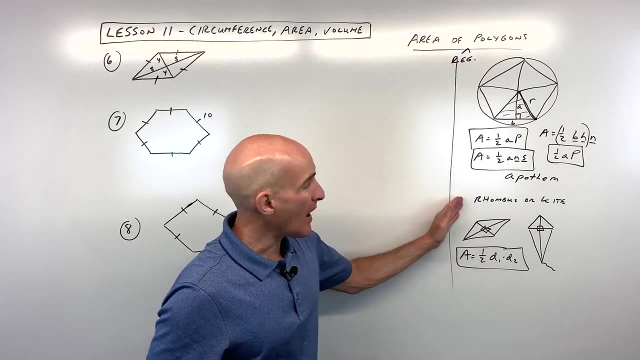 either do one half apothem times perimeter, or one half a and s, or you can just find the area of one half base times height, right? And the word I was mentioning, apothem, is spelled a-p-o-t-h-e-m, and this is for regular polygons. Okay, now for rhombuses and kites, or I should say rhombi is plural of rhombus. 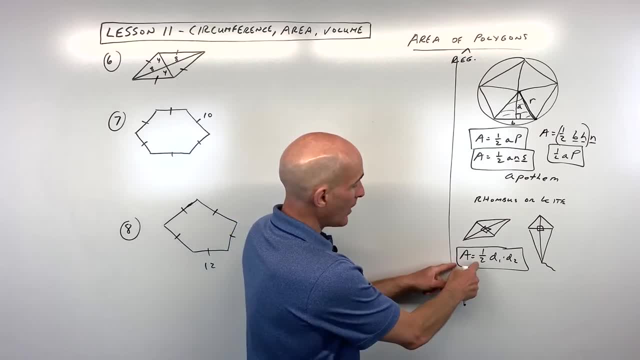 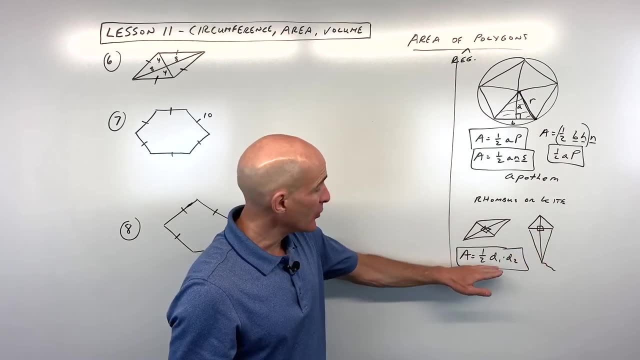 or kite. the area formula is the same. It's one half diagonal one times diagonal two. or here you can see in the kite: diagonal one diagonal two times a half. It looks a lot like the formula one half base times height. right, and that makes sense because what it is is, you can see it's actually. 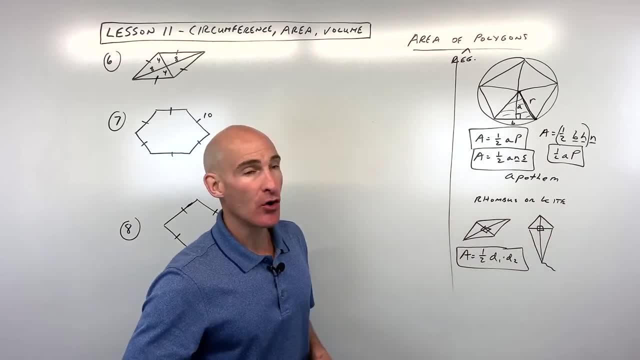 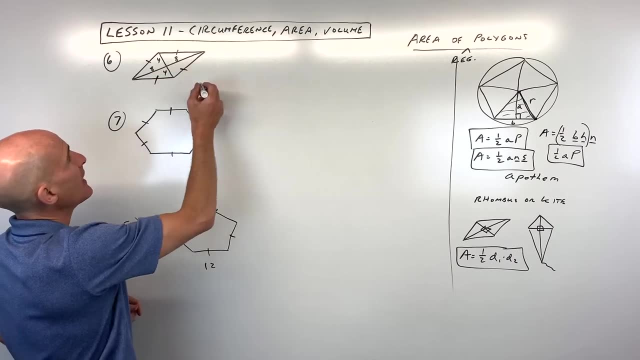 you can divide this into like two triangles. So let's just go into some examples. I'll show you how to work with these Number six. we have a rhombus Notice. all the sides are congruent and we're going to figure out the area using our formula one: half diagonal, one times diagonal two. 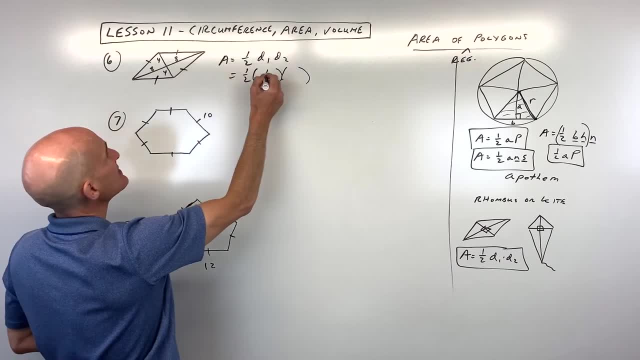 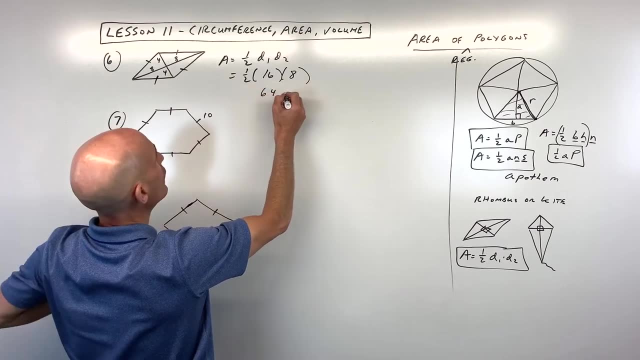 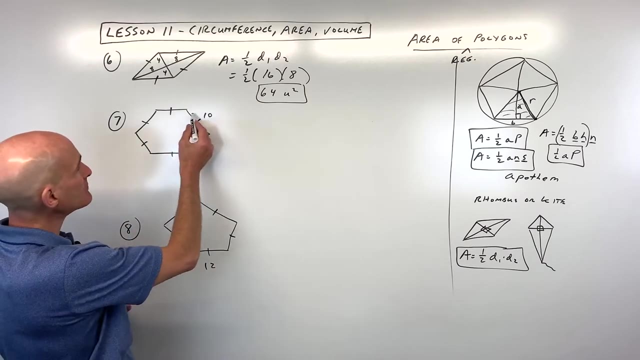 Diagonal one is going to be eight plus eight, that's sixteen. This diagonal is four plus four, which is eight. One half times sixteen is eight times eight is sixty-four units squared, since it's area. Okay for number seven. We have a regular hexagon. Notice there's six sides. We can see that all the sides are congruent. 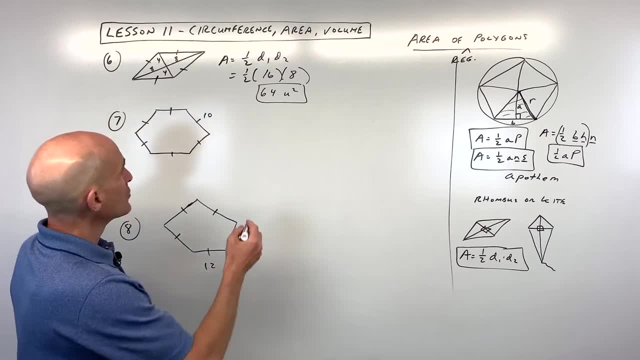 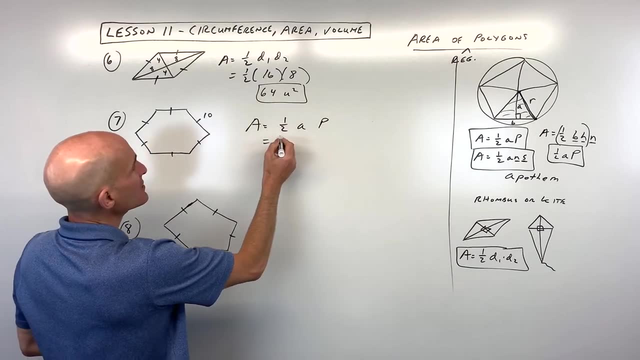 We know it's regular and the length of a side is ten. So let's, I like to write down the formula first and then kind of look for what I'm missing. So let's use the one half apothem times perimeter. So we don't know the apothem yet, but we do know the perimeter. that's going to be ten times six. 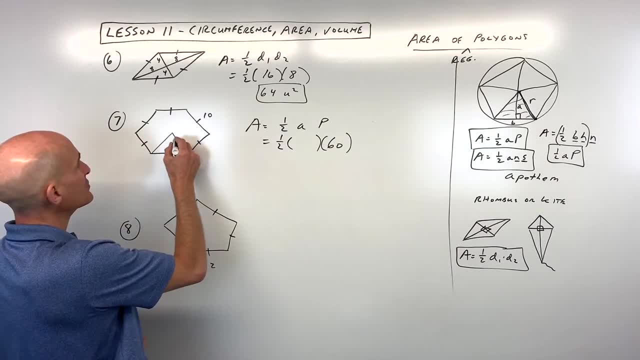 which is sixty. Okay, so now let's go ahead and divide this up into triangles. Okay, and all these triangles are congruent, And this side is ten, But let's look at that central angle there. We know, in a circle there is 360 degrees, right? 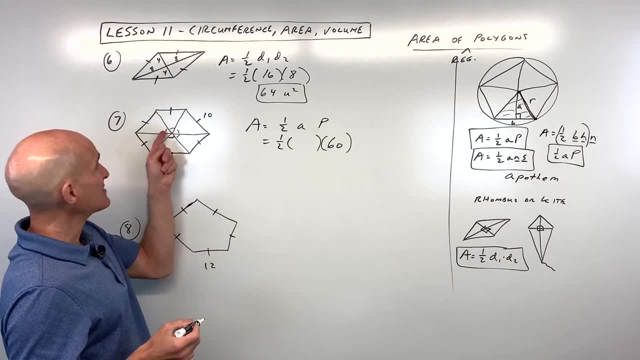 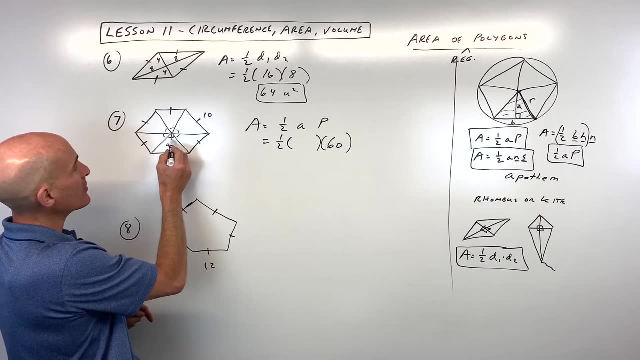 So if we do 360 divided by six, We have six of these angles. That's going to give us sixty degrees for the central angle. Now if we drop in altitude- that's our apothem right here- that's going to bisect this angle. 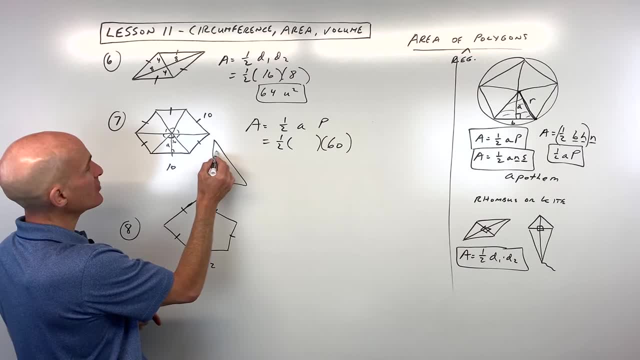 Let's draw it a little bit larger. This angle here is going to be thirty degrees, This is going to be ninety and this is going to be sixty. You can see it's a special right triangle of thirty, sixty, ninety. Also, when you start drawing this in, you're going to get this will be the angle of one half. 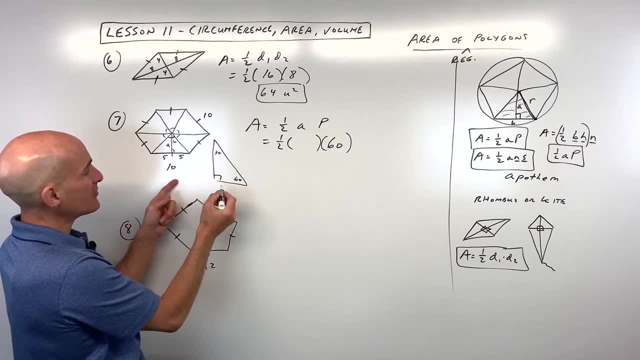 So we're going to start drawing this in. This is going to be one half. this is going to be the angle of one half. Also, when you drop in altitude, it's going to bisect the base or cut the base in half. 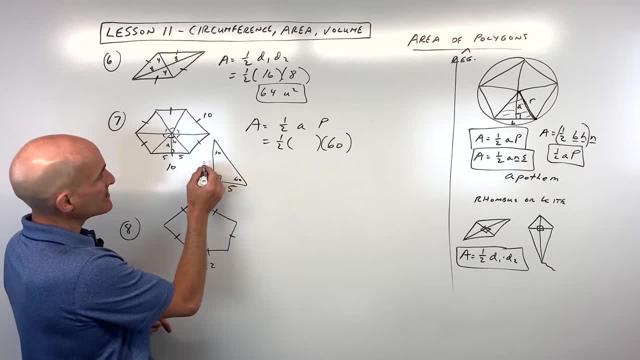 So now this is going to be 5.. And now we know this is x, x, root 3, and 2x. So we know this is going to be 5 root 3 for the height of this triangle, this apothem. 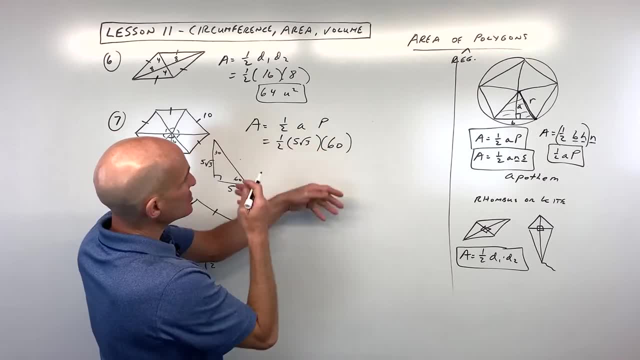 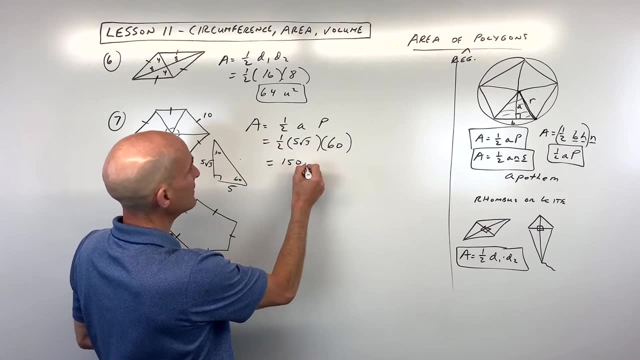 So that's from the special right triangle. So let's see, Multiplication is commutative. We can multiply this in any order. So I'm going to do a half times 60.. That's 30 times 5 is 150 squared of 3 units squared, since it's area. 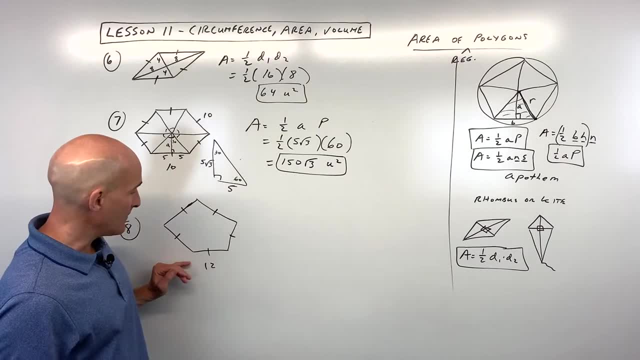 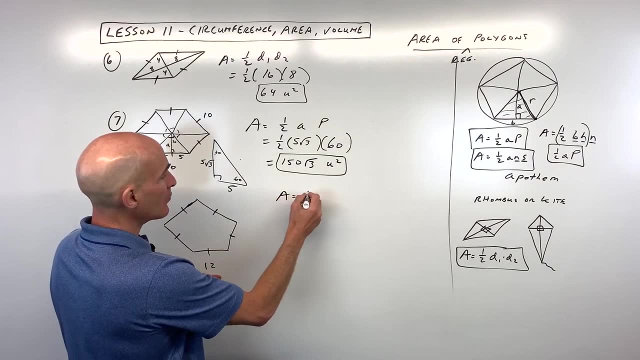 Okay, now let's look at a little bit more challenging one, number 8.. We're going to find the area of this regular pentagon. Notice there's 5 sides. The length of the side is 12.. So again, let's go ahead and write down our formula 1: half apothem times perimeter. 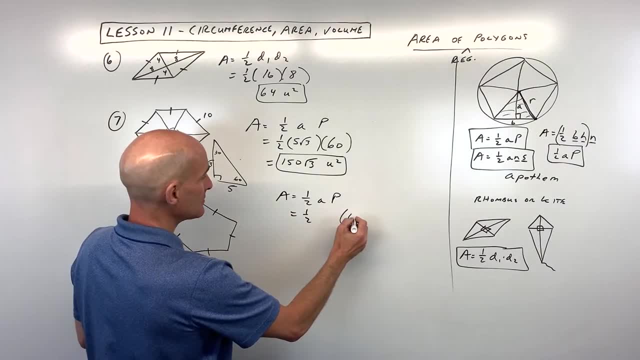 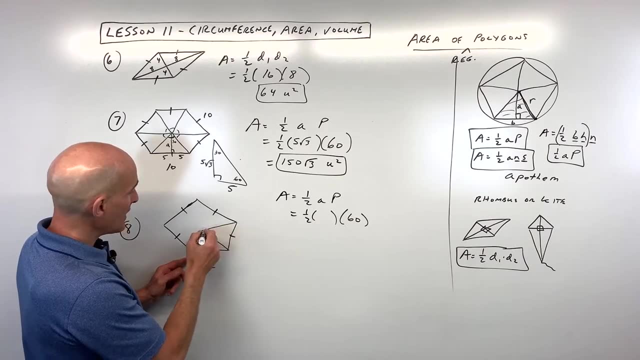 We know the perimeter is 12 times 5,, which is 60. But the apothem we don't know yet. So what we're going to do is we're going to again divide it up into triangles And again, if you forget the formula, no problem. 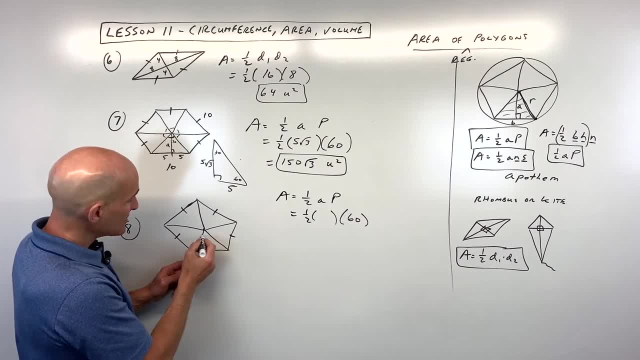 Just find the area of one triangle, multiply it by 5.. But notice this central. See how there's 5 of these central angles. 360 divided by 5 is 72 degrees. But if I drop an altitude it's going to bisect the base. 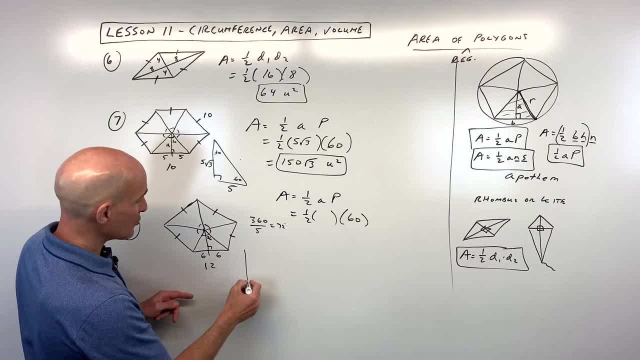 It's also going to bisect this central angle. That's going to make this 36 degrees. So here we have 36 degrees, We have this side here, which is 6.. But we're looking for that apothem. So let me ask you a question. 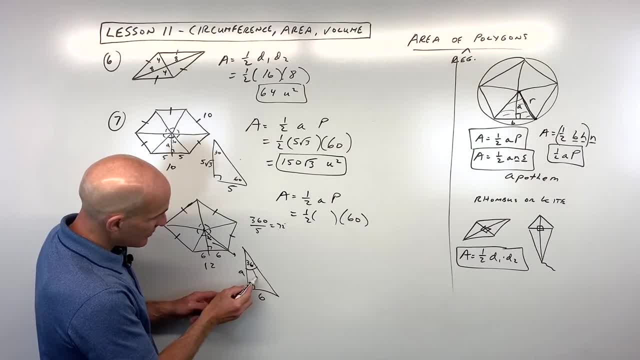 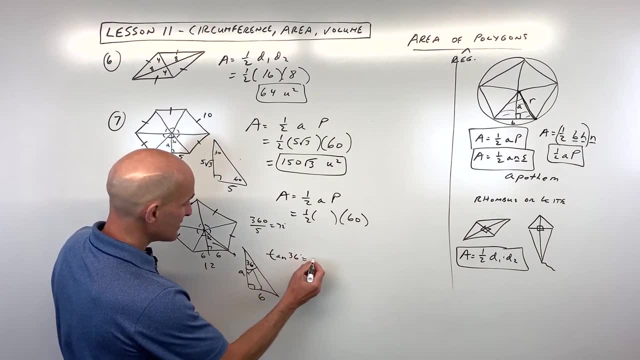 What trig function sine cosine or tangent ties together the opposite side and the adjacent side? Well, that's TOA. So the tangent of 36 equals opposite over adjacent. We can cross, multiply and solve, So let's go ahead and do that. 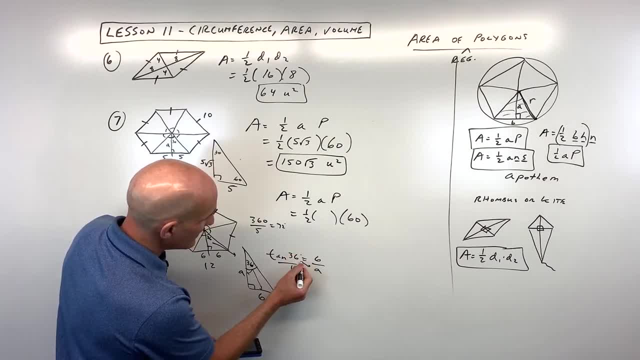 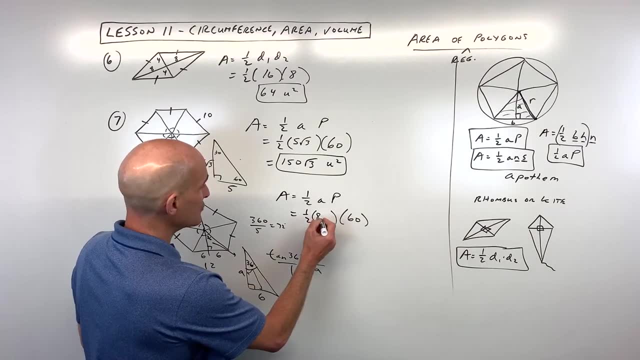 Remember, one of the properties of proportions is you can switch these on the diagonal. So a over 1 is just a. So I just have to do 6 divided by the tangent of 36, which gives us about 8.26.. 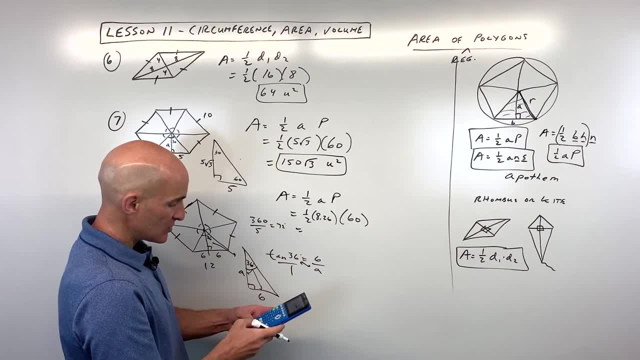 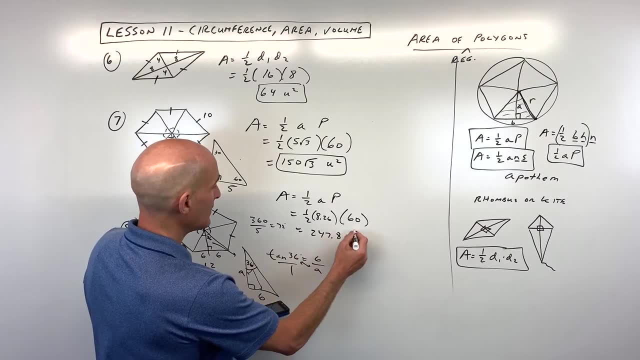 Okay. so now, if we multiply all that out, we've got 8.26 times 1, half times 60.. We're looking at 2.26.. So we're looking at 247.8 units squared for the area of this regular pentagon. 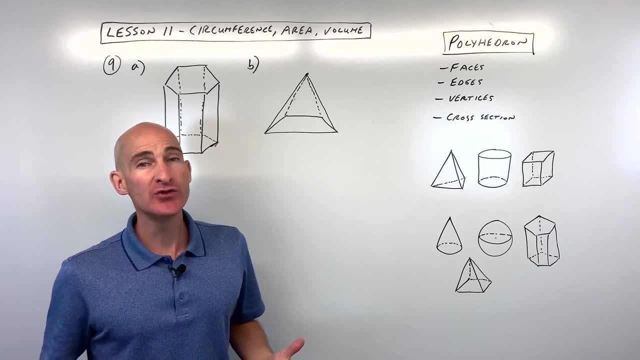 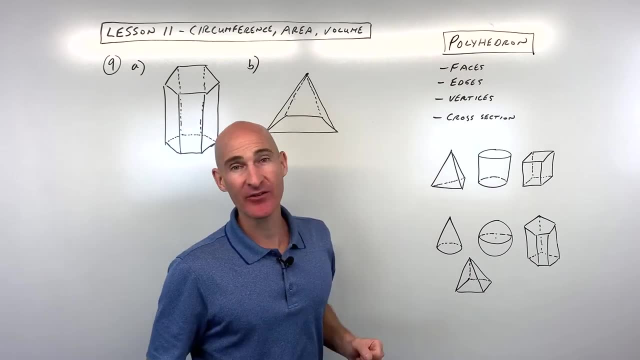 Okay, we're getting ready to get into surface area and volume, But before we do that, we want to talk about polyhedron. So what exactly are polyhedron? Well, poly means many right. Hedron is like sides. 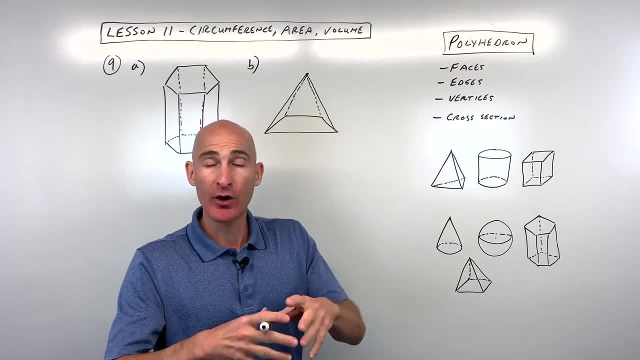 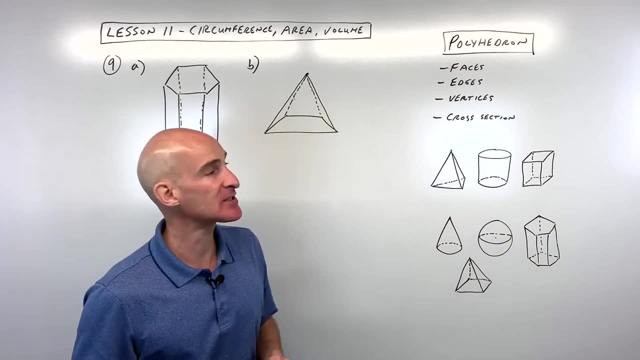 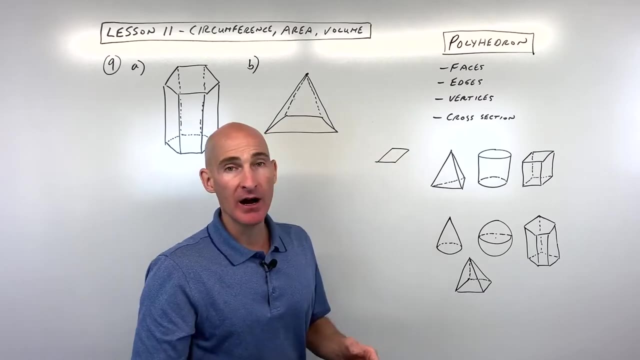 So it's like a many-sided figure, but it's more than that. It's actually a three-dimensional solid that the faces or the sides are made up of polygons. Now remember from an earlier lesson we talked about a polygon. A polygon encloses a single region and its sides are made up of line segments. 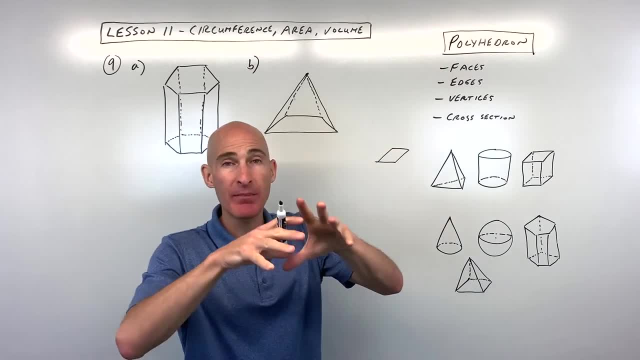 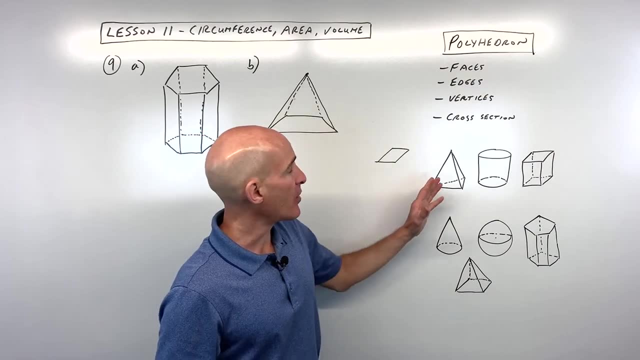 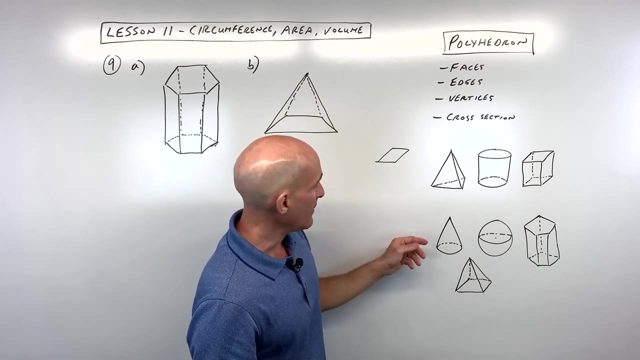 So when you talk about a polyhedron, it has to be made up of those polygons as the outer faces. So that's what a face is. It's a two-dimensional part of the figure that makes up the side, Where an edge is where two faces come together and they're going to form a line. 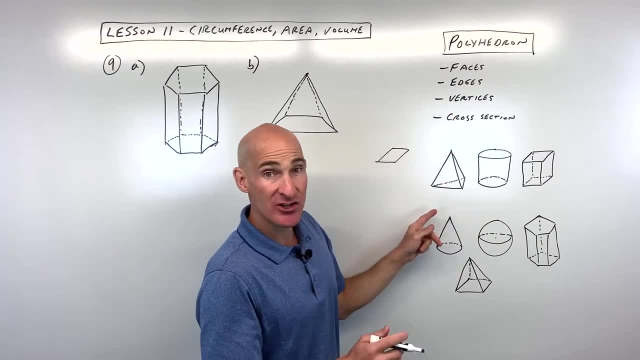 It's basically like this: here And a vertice is where two edges And when the edges come together they're going to form like a point, that's like a vertice, And then we'll talk about cross-section in just a second. 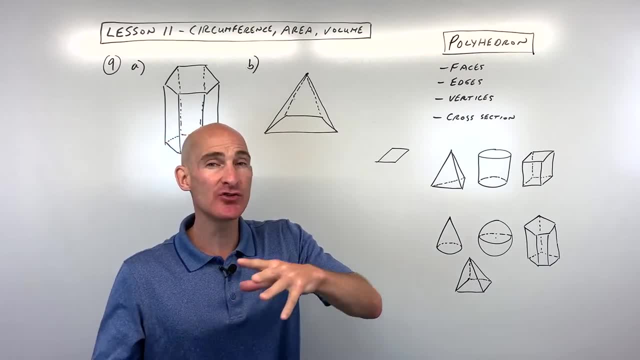 But first of all let's look at some examples. Which one of these are polyhedron and which are not polyhedron. So when you look at this one here, is this a polyhedron? Are all the faces made up of polygons? 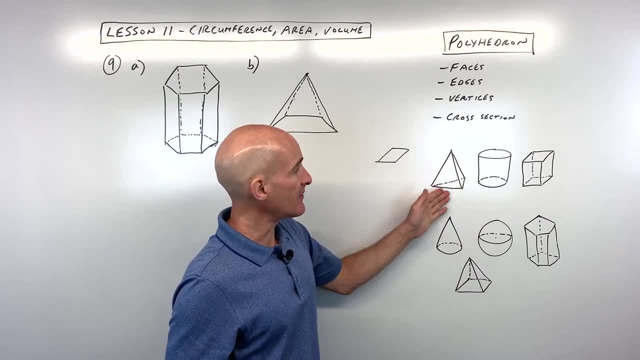 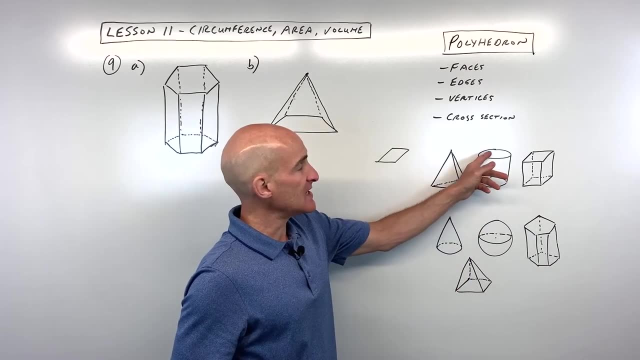 Well, yes, In this case they're all made up of triangles, So this is definitely a polyhedron. So let's just write yes for this one. How about for this one? Is this a polyhedron? Well, you can see, this is a cylinder. 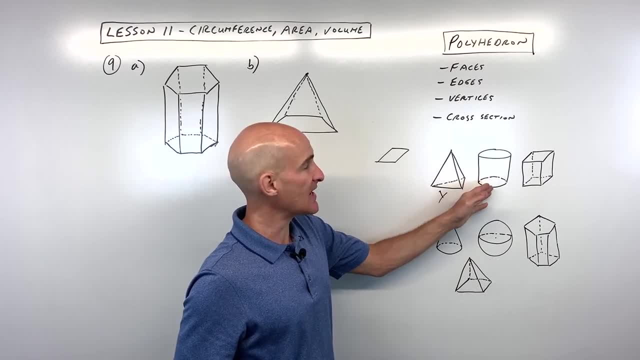 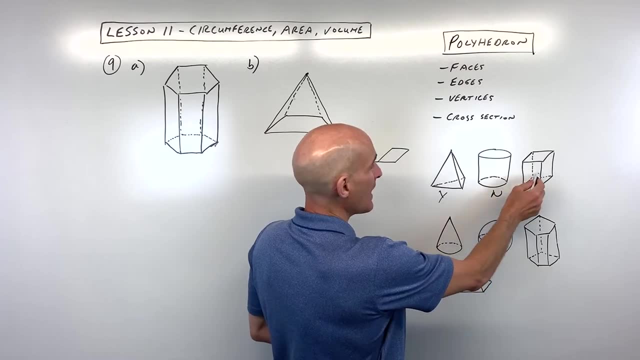 These are made up of circles. right for the two bases. This is not a circle, is not made up of line segments. it's not a polygon, so this is not a polyhedron. We'll say no. How about for that one there? 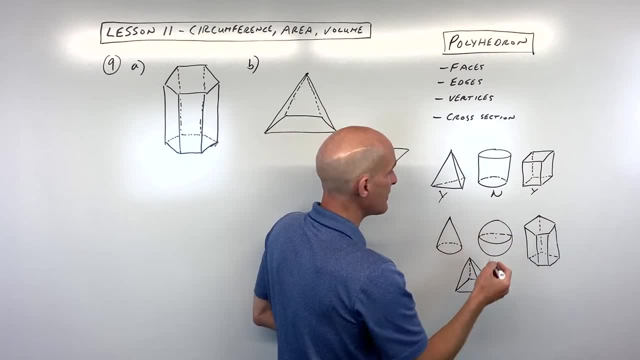 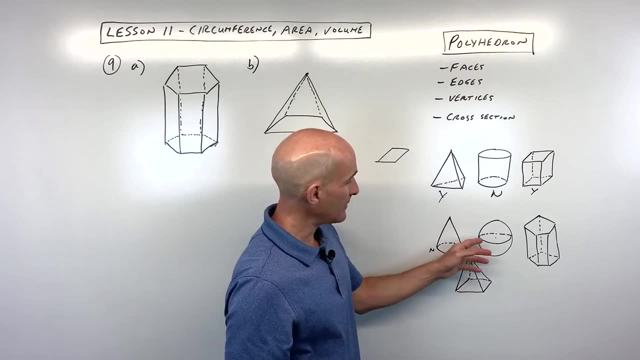 Looks like it's made up of squares and rectangles. those are all polygons. so this is a polyhedron. How about this one here? This one? you can see the base is a circle, so this would be. no, that's not a polygon. 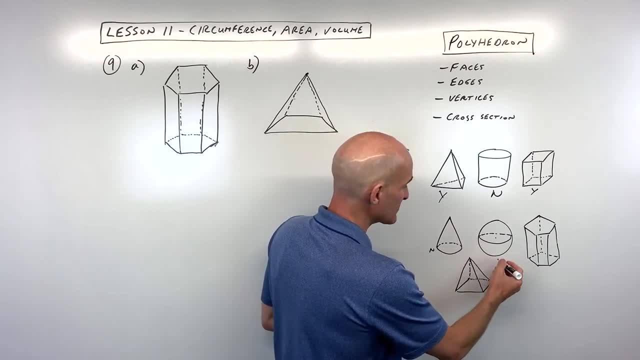 This one is like a ball, and we're going to talk about the more specific names in just a minute, but this is not a polyhedron. This one looks like it's made up of pentagons and it's also rectangles. so yeah, this one's. 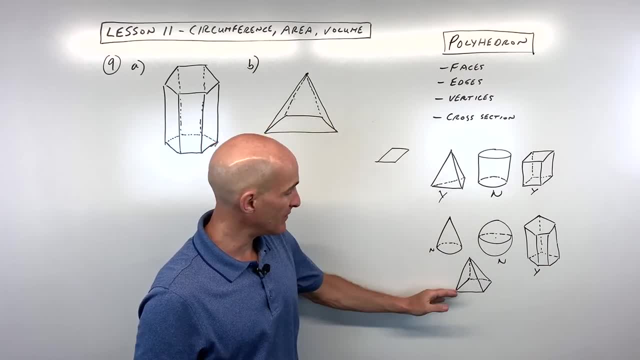 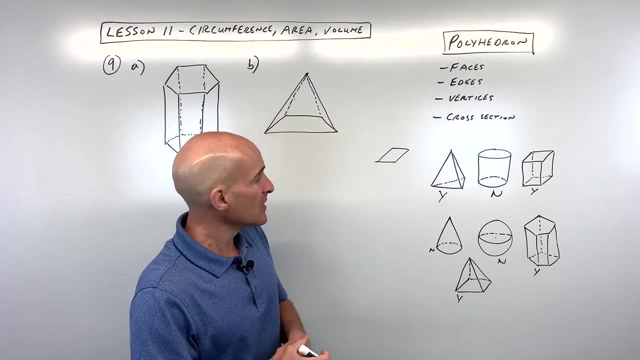 made up of all polygons as faces. that's a polyhedron, and this one looks like a square and some triangles. so yes, this is a polyhedron. Now let's get a little bit more specific now. So notice the difference between like this shape and this shape. 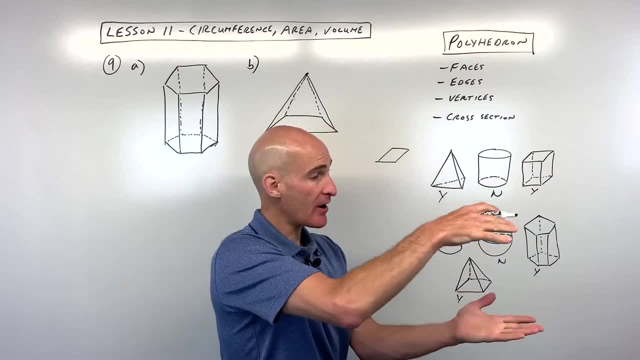 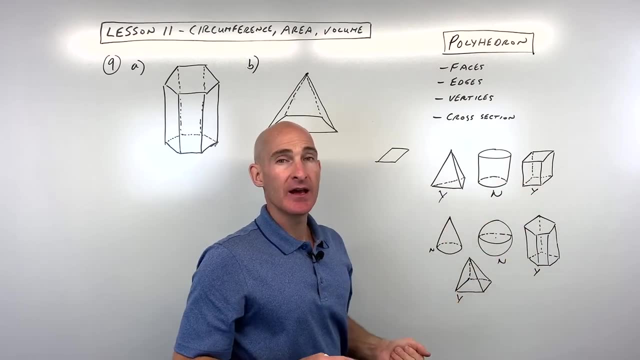 See this shape: you have two squares that are parallel and congruent to one another, These are referred to as the bases, and when you have two bases that are parallel and congruent like that, this is referred to as a prism and we name it by the base. so this is like: 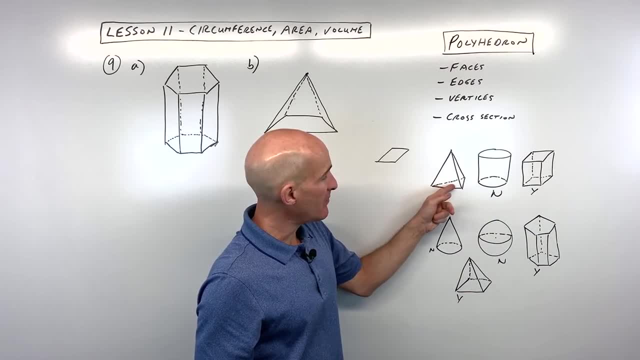 a square prism, whereas this one, you see, the bottom is a triangle, but the top is not a triangle. It comes to a point, It comes to a vertex. This is what we refer to as a pyramid, and we name it by the base. 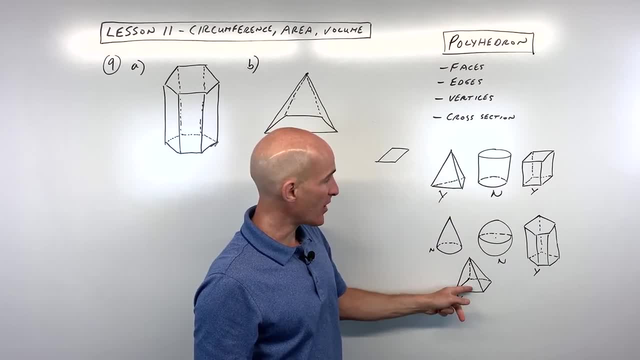 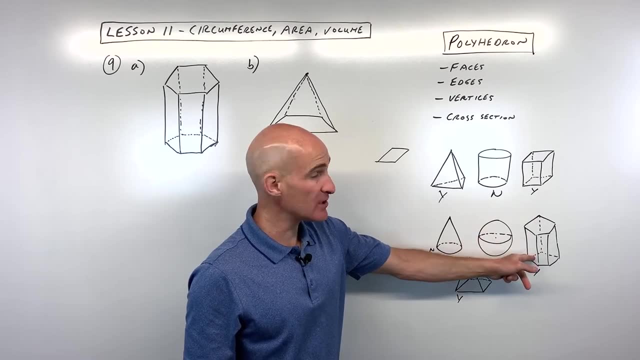 We say this is a triangular pyramid. Over here, this is like a square pyramid. This one here, notice, you have two pentagons that are parallel and congruent, separated by the height. This is a prism, but more specifically, a pentagonal prism. 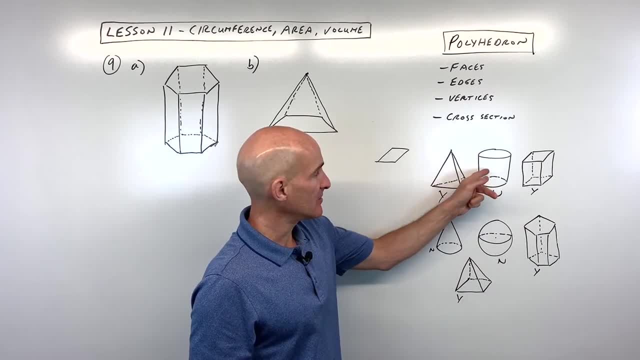 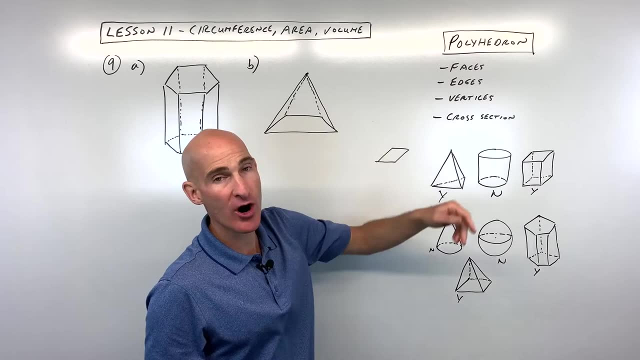 Two pentagons. This is a cylinder, This is a cone, This is a sphere. Okay, let's look at some examples, but before we do that, let's talk about the cross-section. So cross-section is like if you were to take a plane like a flat surface and you were 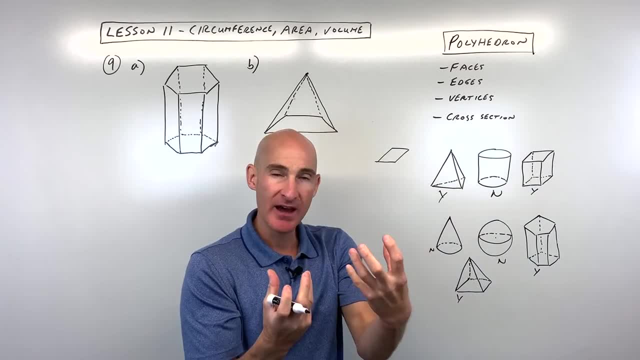 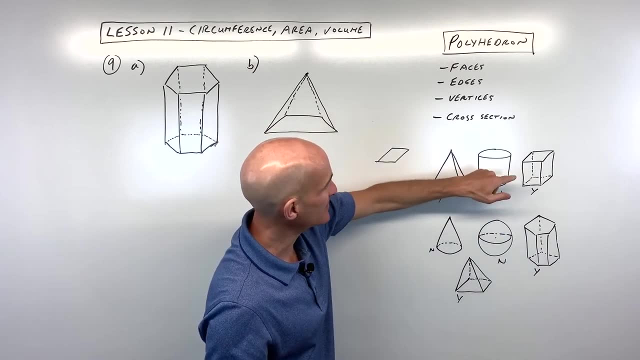 to cut through that figure and you were to look at that, like when you split it and you look at that exposed part, you say, hmm, what kind of a shape is that? That's your cross-section. So if I was to cut this cylinder like this, what kind of a shape is that? 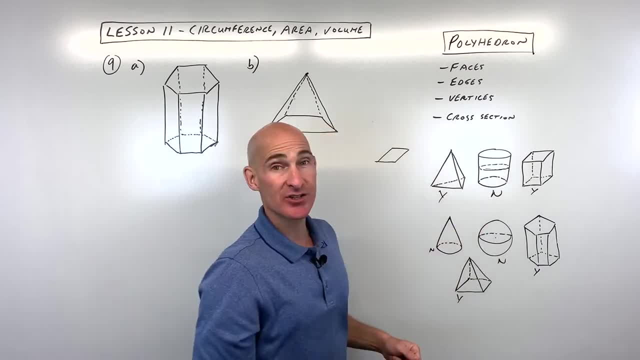 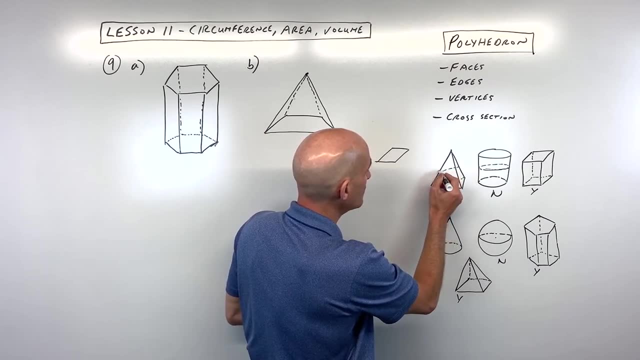 Okay, What would we be looking at right there? A circle right, So that's your cross-section. If I was to cut this, what would I end up with? Well, depending on the angle, it's very important the angle. 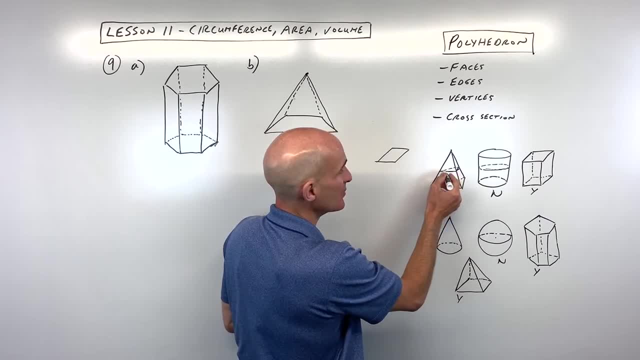 See if it's parallel to the base, it's going to be the same shape as the base. In this case, it's just going to be a little bit smaller. It's still a triangle, This one. if it's parallel to the base, it would be a square. 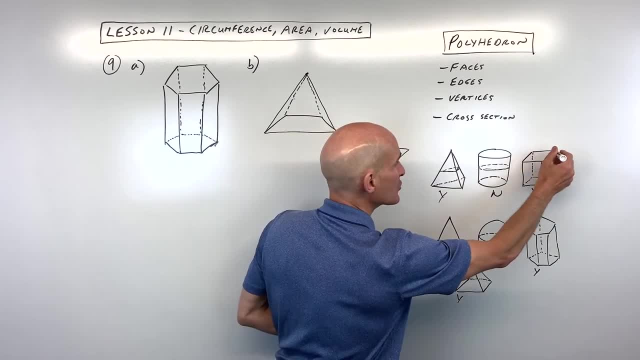 If it was like this, you know, you may get a rectangle. If you go on a diagonal, you could even get a triangle. So those are what are called cross-sections. but let's look at a couple examples. So what do you think for A here? 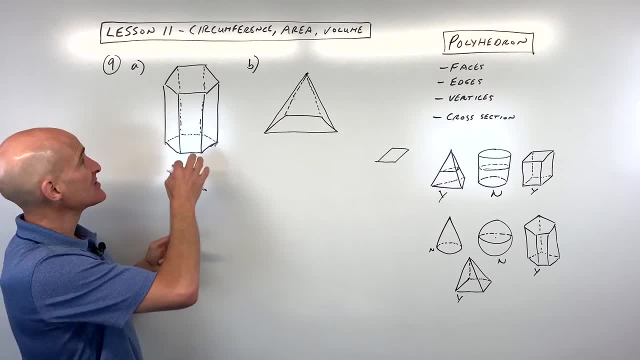 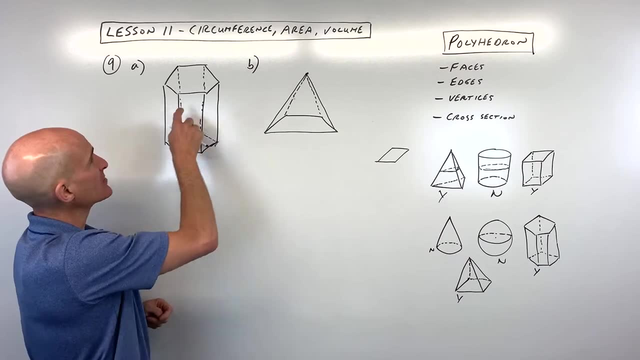 Is this a point? Is this a polyhedron? Yes, We can see all the sides are made up of polygons. right, And let's see what's the name of this shape? Well, it looks like the top and the bottom are hexagons, and you can see they're parallel. 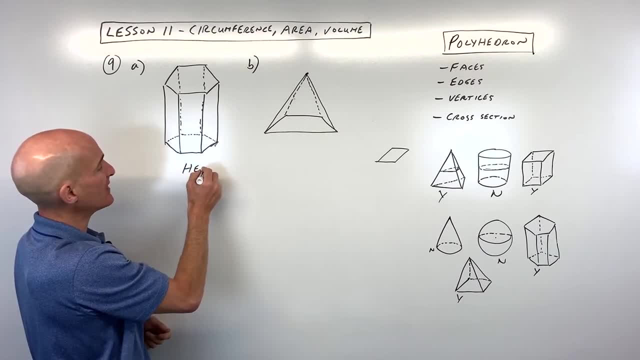 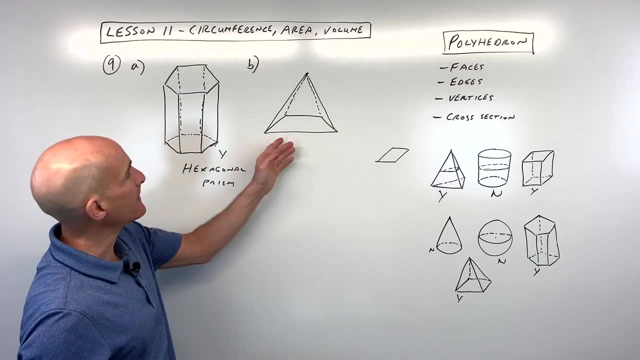 and congruent. So this is a hexagonal prism. So let's write that down: hexagonal prism. and it is a polyhedron. so we'll say yes. How about for letter B here? Is this a polyhedron? 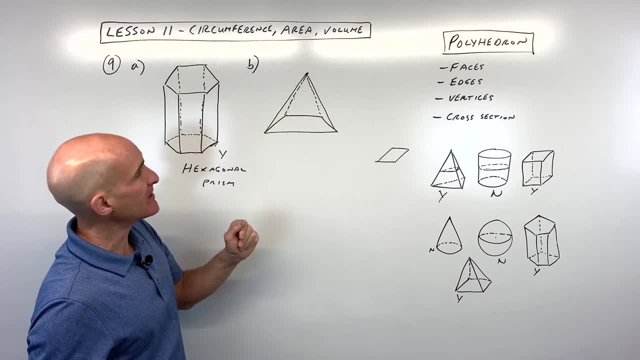 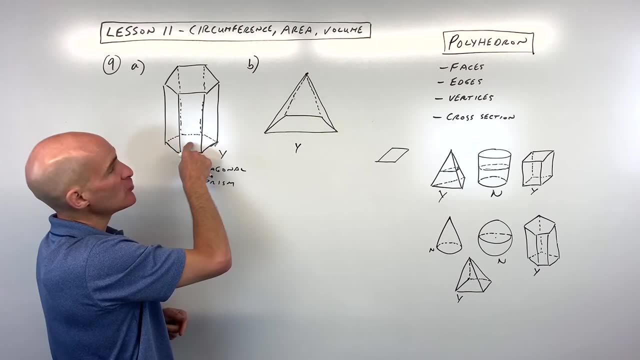 Yeah, it looks like all the sides, all the faces, are made up of polygons. so I would say, yes, this is a polyhedron. but, more specifically, what's the name here? Well, it's not like this one where we have two parallel and congruent bases, so it's. 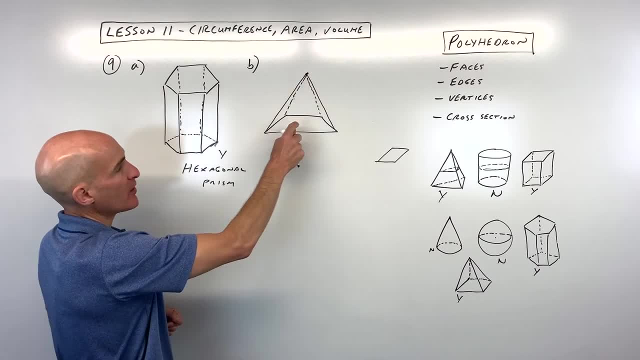 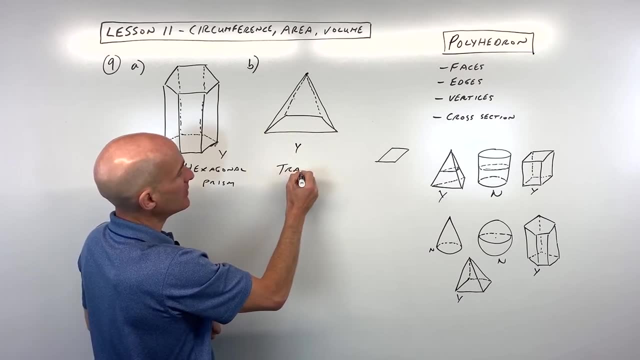 not going to be a prism. Looks like it comes to a vertex, a point here. This is a pyramid, but what type of a base is that? Well, I tried to illustrate as best I could here. It's actually a trapezoid, so we're going to call this a trapezoidal pyramid and we're 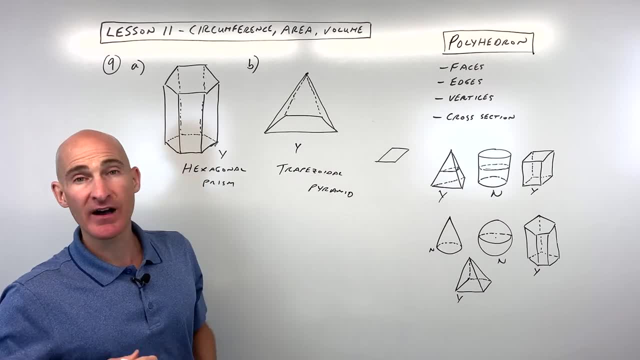 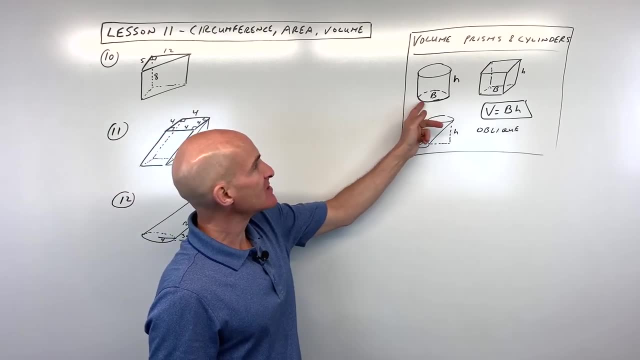 going to talk about how to find the areas of the surface areas, volumes of these shapes. in just a moment We'll start off by talking about the volume of prisms and cylinders. So in a sense you could almost think of a cylinder as like a circular prism, like the 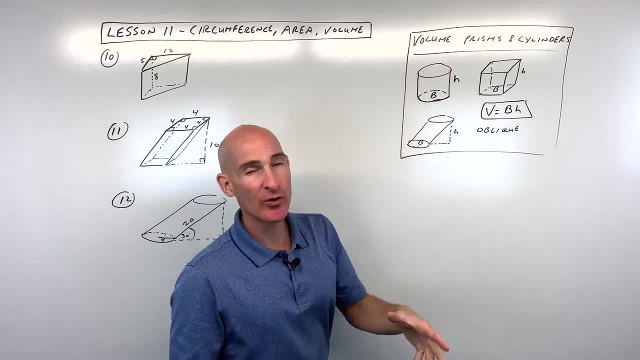 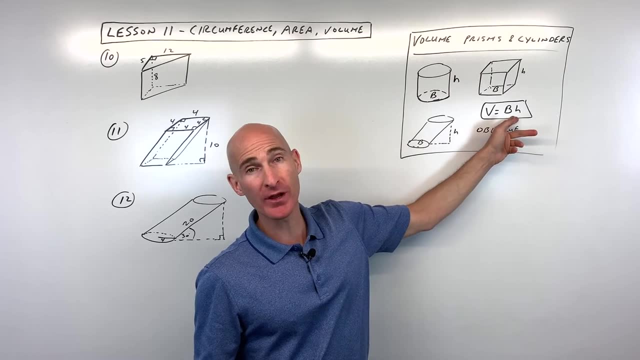 top and the bottom are circles. they're separated by the height. We don't call it a circular prism, but you can kind of think of it like that, because these two formulas, I mean these two figures- they have the same formula. The volume is the area of the base. that's what the capital B represents times the height. 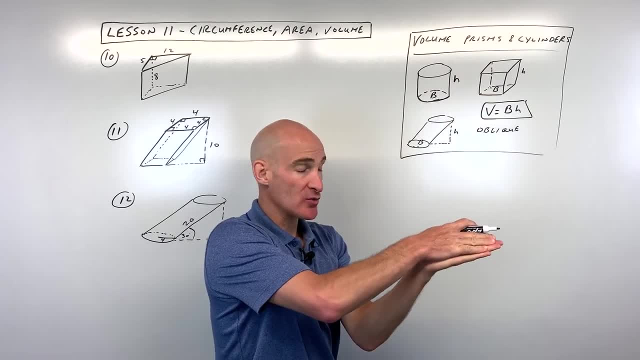 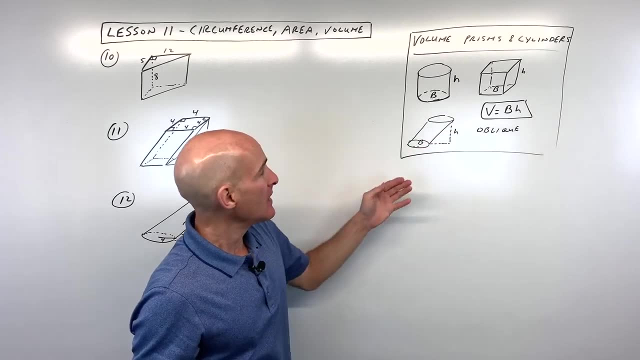 And so it's kind of like, if you look at this example here, it's kind of like taking these squares, which are two-dimensional, stacking them up, You know, in the third dimension, and that gives you the three-dimensional volume. 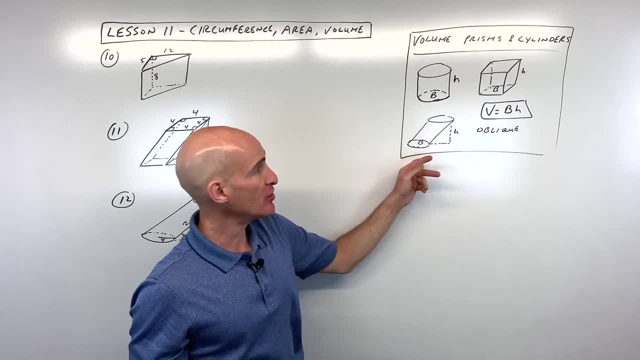 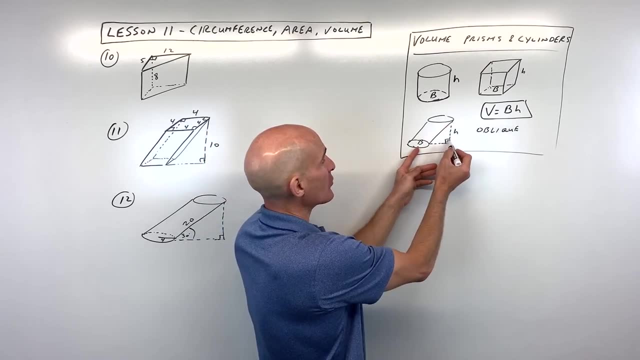 Now over here, what we have is an oblique cylinder. you can also have an oblique prism, but again, what you want is you want the area of that base times the perpendicular height. okay, this perpendicular distance between the two bases, not that diagonal height. 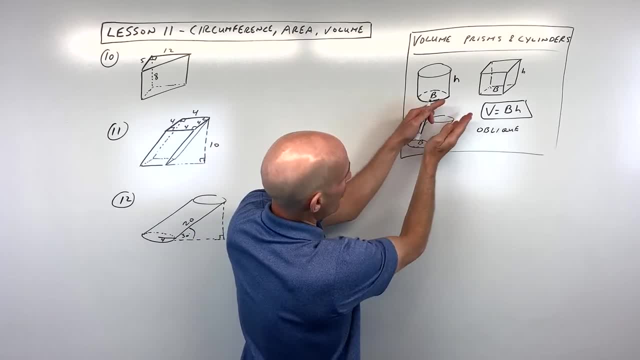 It's kind of like if these were a stack of quarters and you kind of had them a little bit off, a little bit on a little bit of an angle. imagine if I was to straighten them back up. It's not like they would get taller. 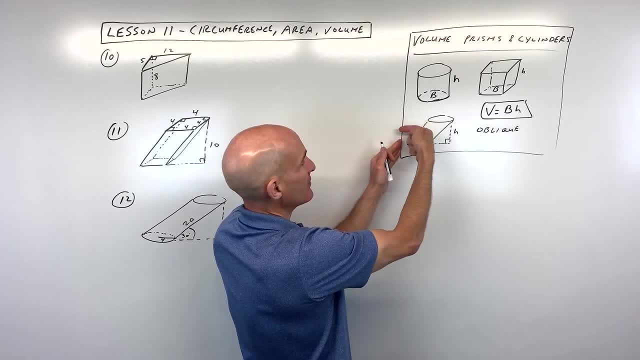 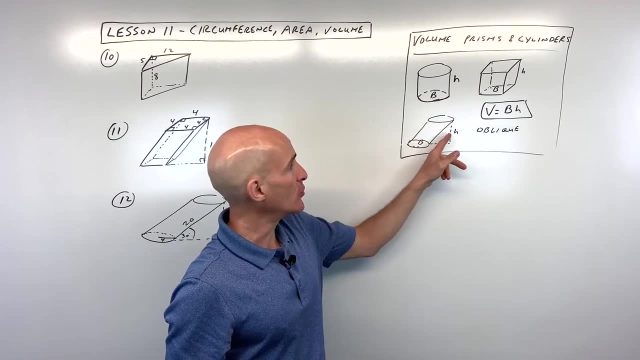 You're just sliding each coin horizontally to the left here, and so it's really going to be the same volume, you know, as a normal right cylinder, with that same height and same base. So let's look at some examples. I'll show you how this works. 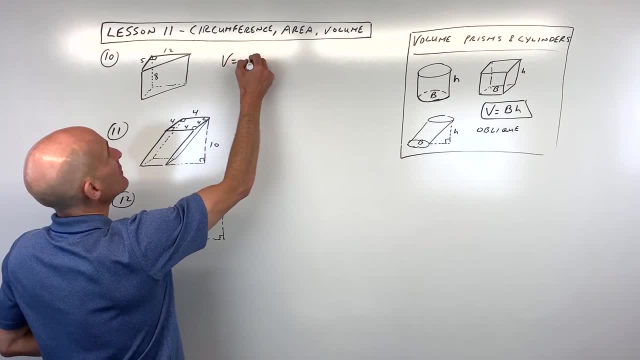 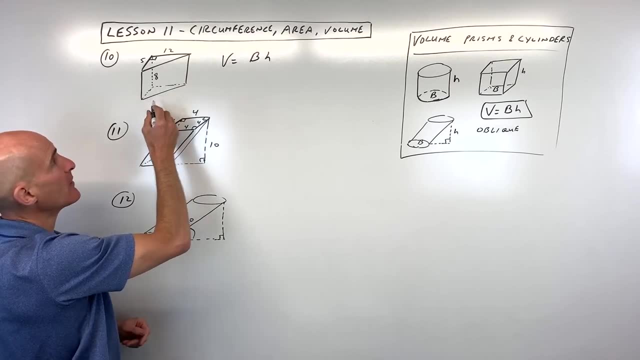 So for number 10, what kind of a shape is this? Well, if you said a triangular prism, you're absolutely right. you can see, the top and bottoms are triangles, they're parallel and congruent and they're separated by that height. 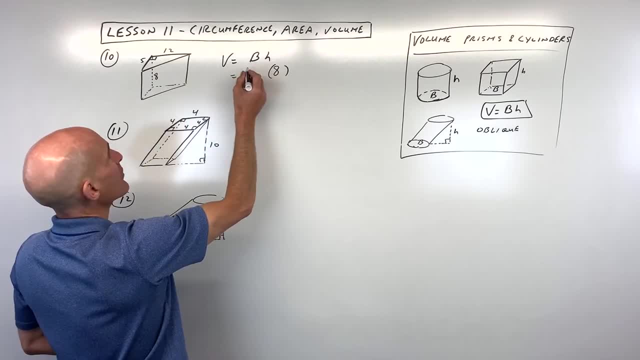 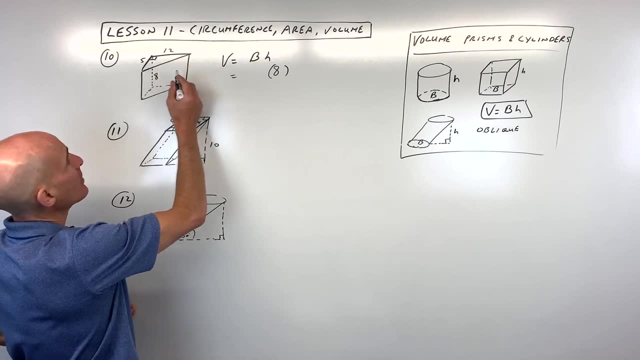 which, in this case you can see is 8 units. so we have 8, but remember the B represents the area of the base capital B. so this is a triangle. so what's the area of a triangle? Well, the area of a triangle is actually 1 half little b times h, 1 half base times height. 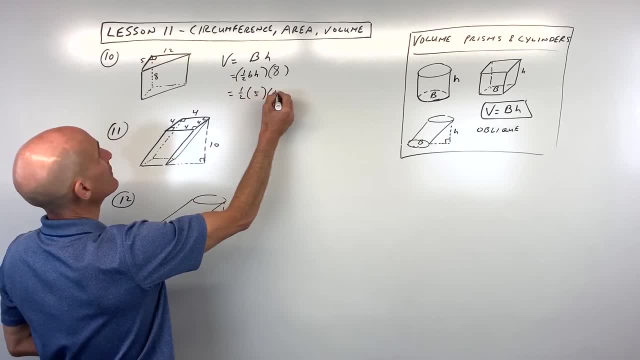 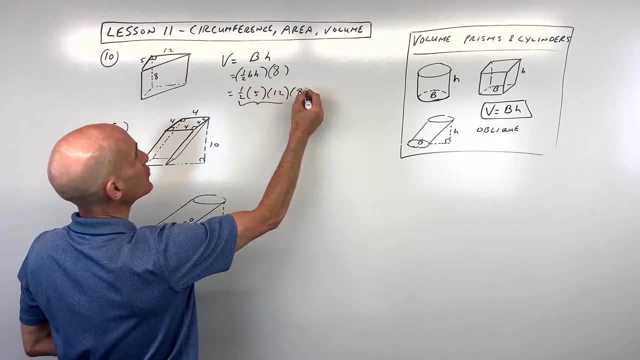 so what we're doing here is we're doing 1 half, 5 times 12, that's the height of the triangle. this gives us the area of the triangle. then times the height, which is the distance between the two triangles, that's 8.. 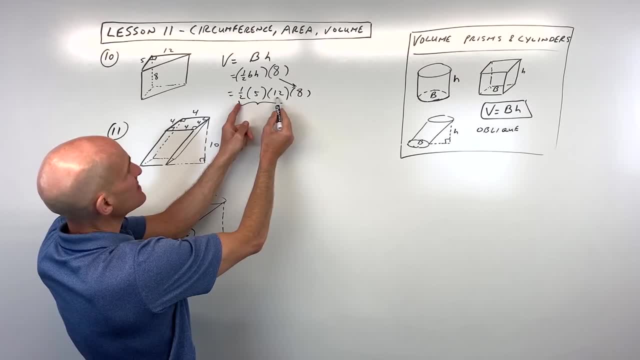 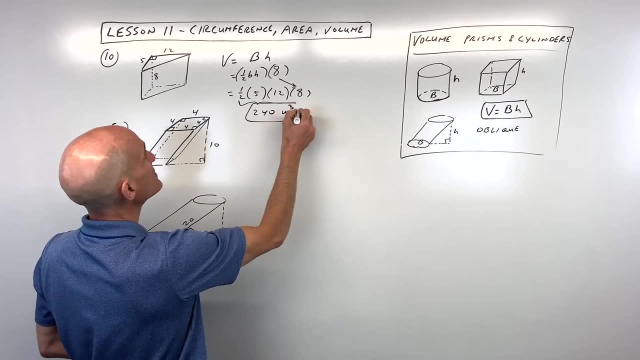 So let's see, You can do this in any order. 1 half times 12 is 6, 6 times 5 is 30,. 30 times 8 is 240 units cubed. it's like you're filling this up with like little ice cubes, like 1 by 1. 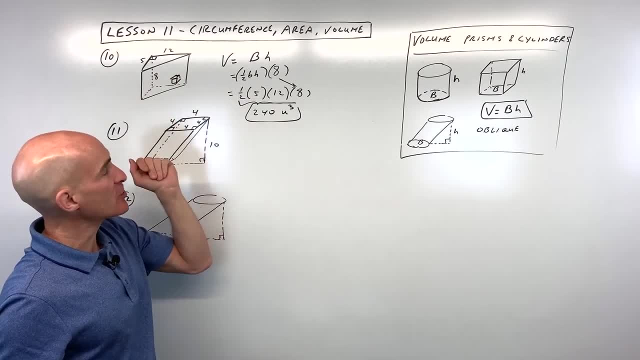 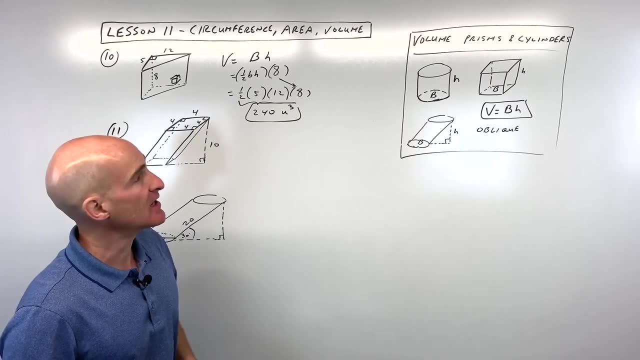 by 1 ice cubes and that's how many we'll fill in the interior. One thing I haven't pointed out yet, but when you get to drawing these figures you want to kind of practice as you do these, but notice the dashed or the dotted lines, what that? 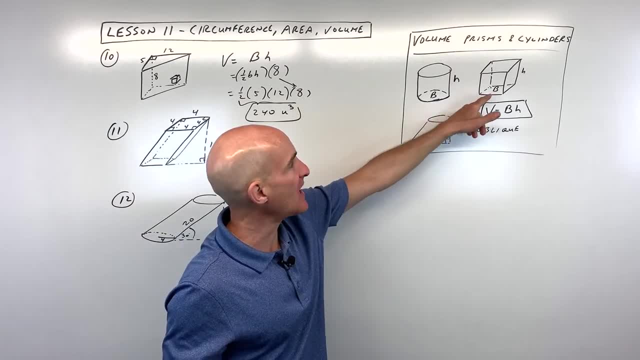 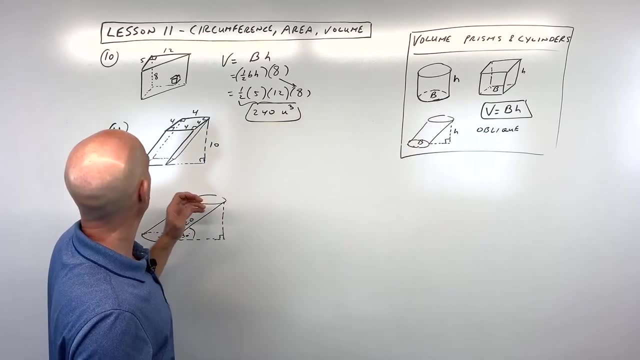 represents is like you're looking through The object to the other side, so it's kind of like hidden. normally you wouldn't see these lines, but it kind of helps us get that 3 dimensional view so we can see what we're looking at. 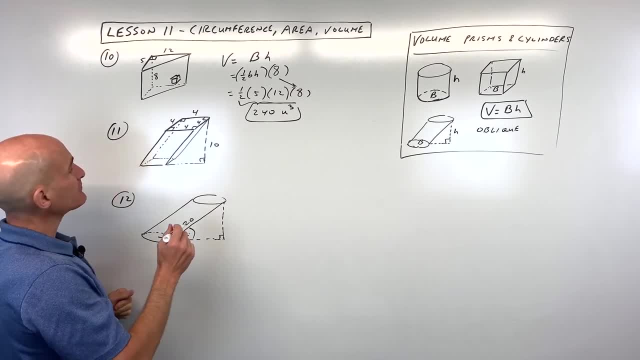 For number 11, what do you think the name of this figure is? Well, you can see the top and bottoms are squares, but you can see it's been tilted a little bit right. So this is going to be an oblique square prism. oblique square prism. the volume formula is: 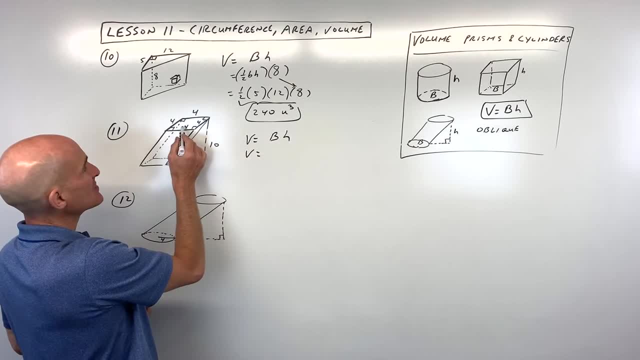 the same, though. area of the base times the height. Okay, the area of the base is the same. the area of the base times the height. Okay, the area of the base is the same. the area of the base times the height. 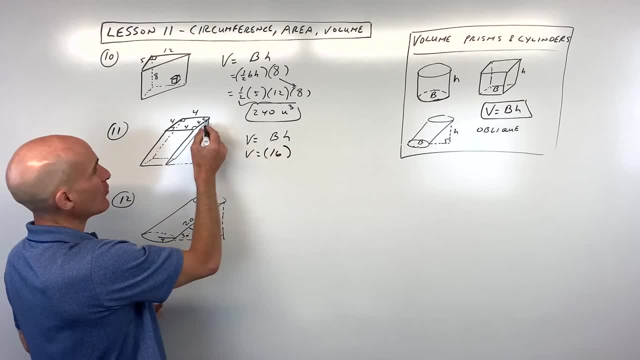 The area of the base is the same. the area of the base times the height. Okay, the area of the base is the same. the area of the base times the height. So 4 times 4 is 16.. The height, though: we want that perpendicular height, which is 10, not this diagonal height. 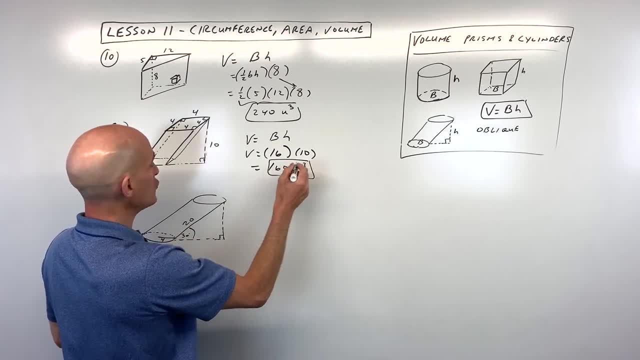 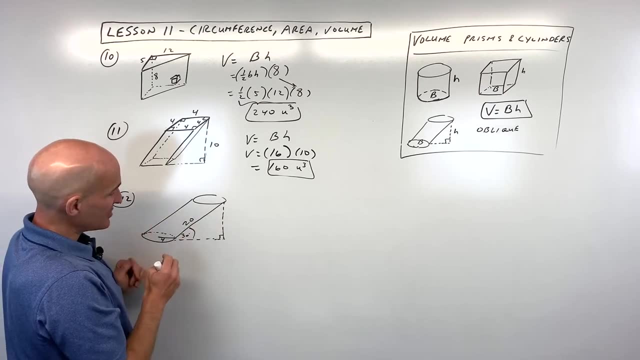 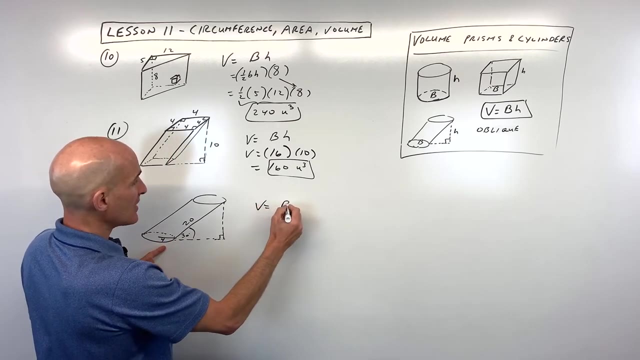 So this is going to give us 160 units cubed. And then the last one here. this is a- what do you think? definitely looks like a cylinder that's been tilted essentially right and it's an oblique cylinder. So we're going to say for this one, volume equals area of the base, times the height. 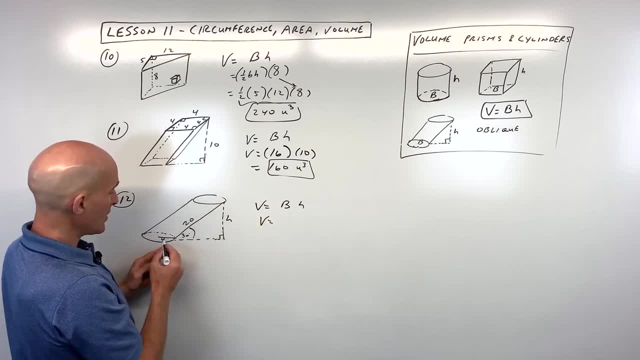 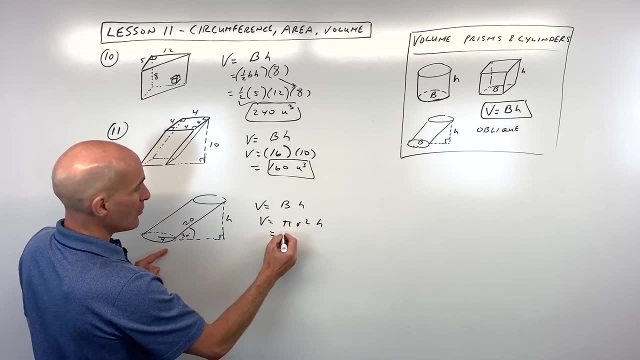 The only thing is, though, they didn't give us the height, so let's figure out what we know here. we know that the base is a circle, so we're going to be using pi? r squared times the height. Okay, so pi r squared, the radius is 4, 4 squared is 16.. The height, though? okay, you see how this. 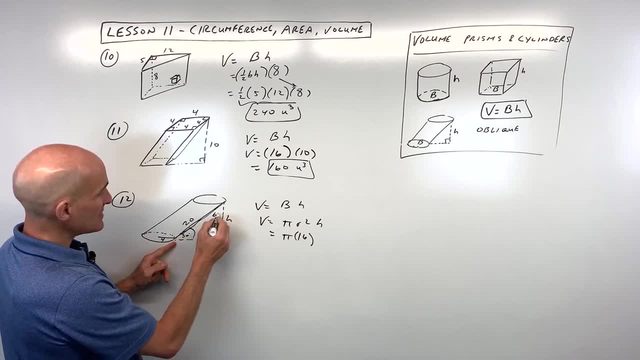 diagonal here is 20 and see how this is 30 degrees. so that means this is a 30, 60, 90 special right triangle: The one that's across from the 30, that's the short leg. the one across from the 60, that's the longer leg. the one across from the right angle, that's the hypotenuse. 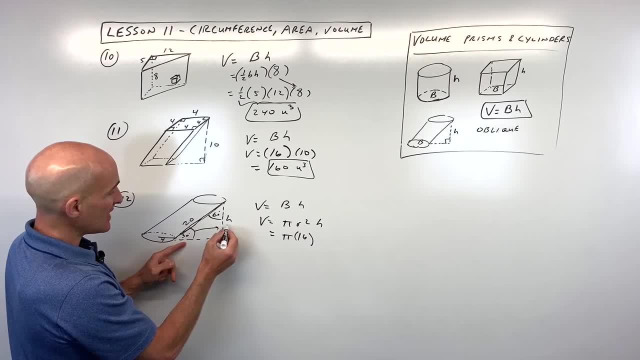 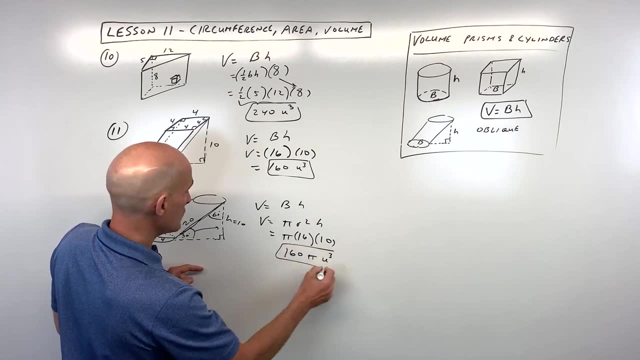 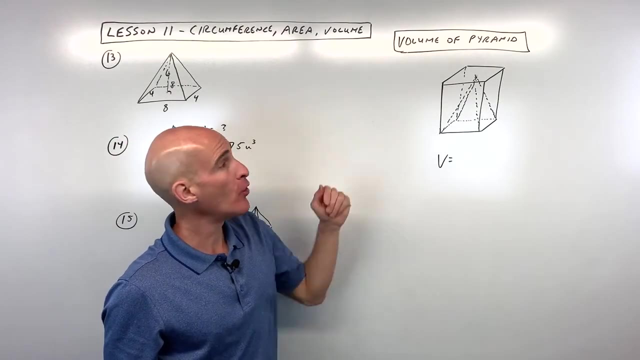 The short leg is half of the hypotenuse, so this is actually going to be 10.. So this is going to be 160 pi units cubed, and that's going to be your volume. Okay, now let's talk about the volume of pyramids. So what I want to show you here is: imagine if you had a square prism and you put a. 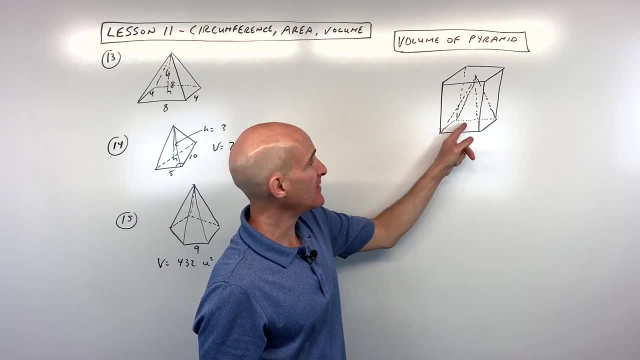 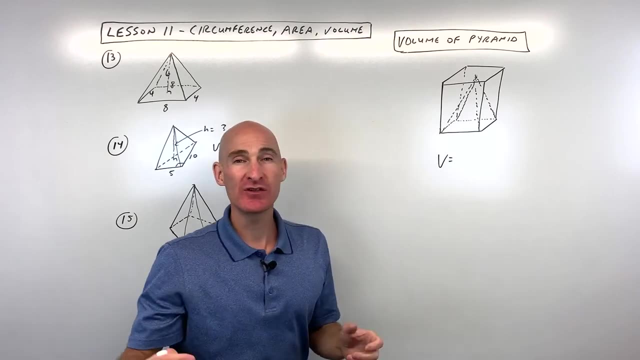 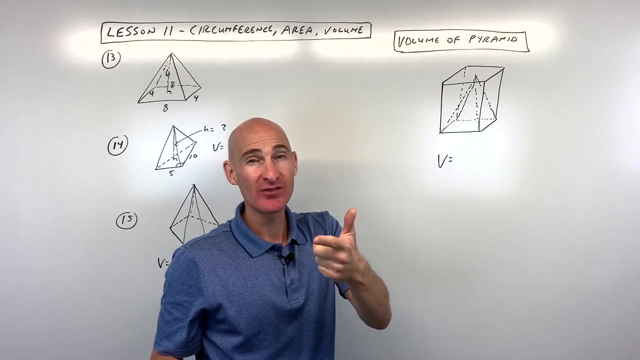 square pyramid inside of that prism and that the pyramid had the same size, base and the same height as the square prism. how many of these pyramids do you think you could put into that square prism, into this box here? one, two, three, four. well, you could actually fit three of these in here. you can. 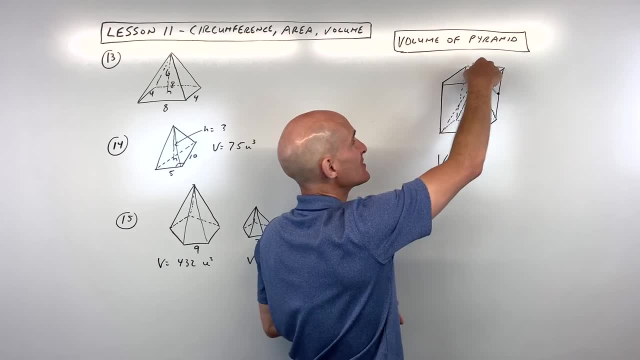 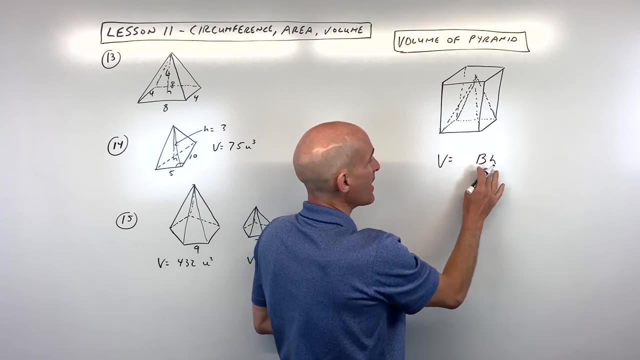 see it's tapered right like this. you could actually fit two more in addition to this one. here you might have to cut them up a little bit, but that's where the formula you can see. it kind of is the same as the volume of a prism, but because this only takes up one-third of the volume, you can divide by three. 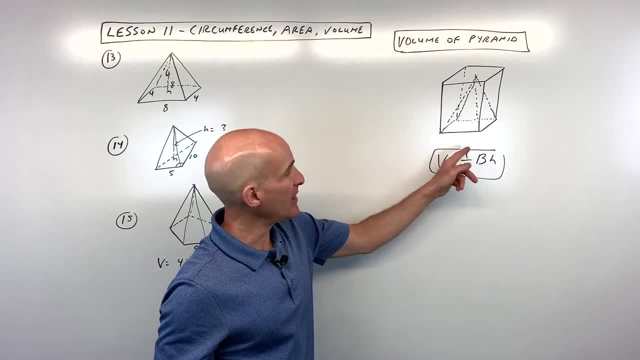 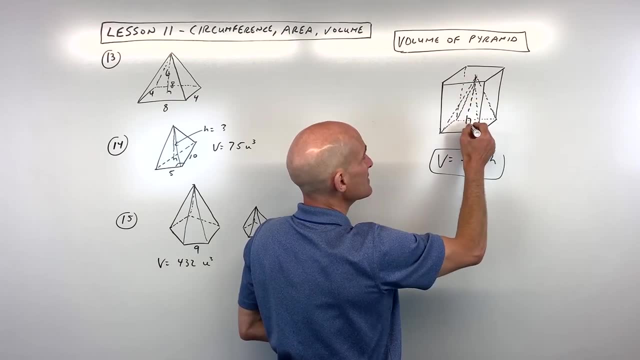 or multiply by one-third. so that's the idea area, the base, whatever shape the base is, times the height, and you want that perpendicular height, that shortest distance from the vertex to the, to the base, and then divided by three or times one-third, so say, for example, number 13. we have 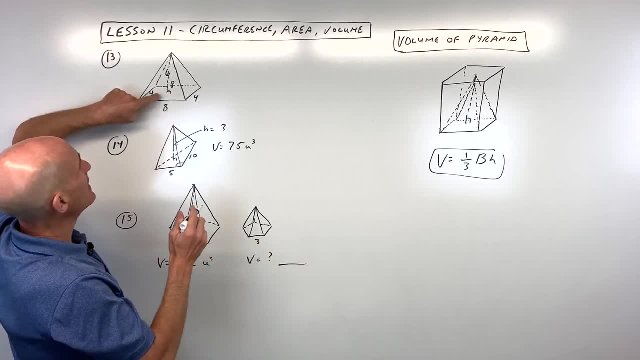 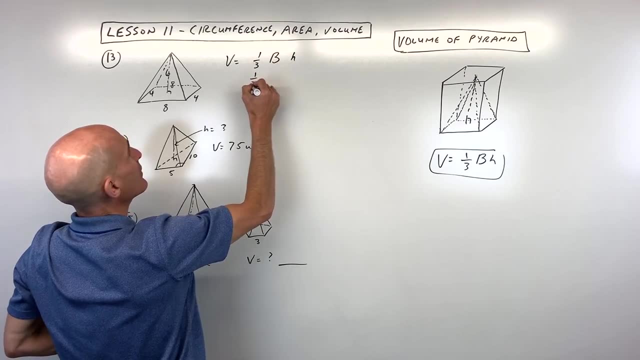 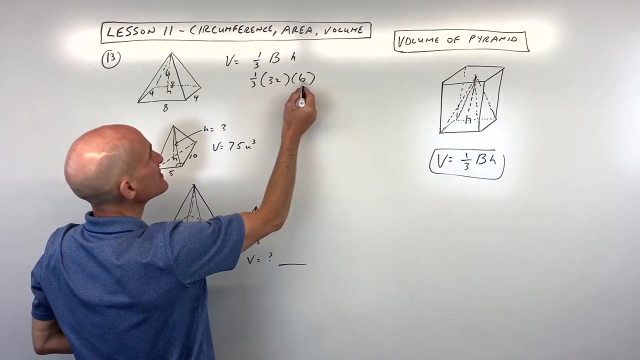 a rectangular pyramid. see, it's a rectangle for the base and the height. so let's go ahead and do that. volume equals one-third area, the base times the height. the area of the base. it's a rectangle. so eight times four, that's 32. the height, that's six. one-third times six is two. two times 32 is 64 units cubed, since it's. 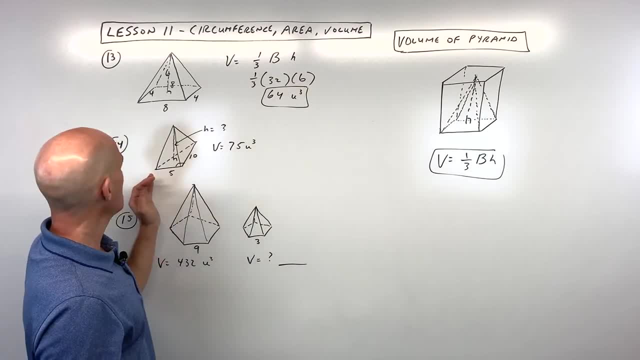 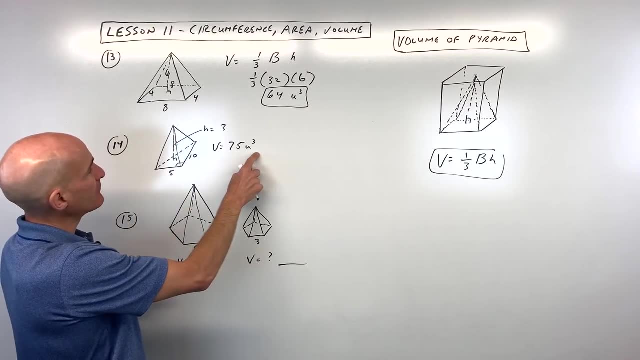 volume. remember, multiplication is commutative. you can do it in any order. for number 14 looks like we have a triangular pyramid. they're giving us the volume but we don't know the height. so what i always like to do is start off by writing my formula down and substitute in what i know, so the volume 75. let's put that in. 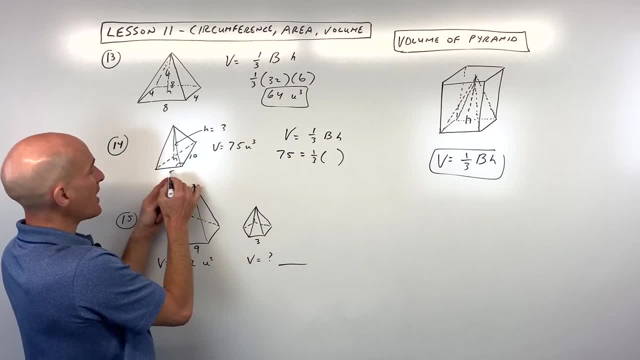 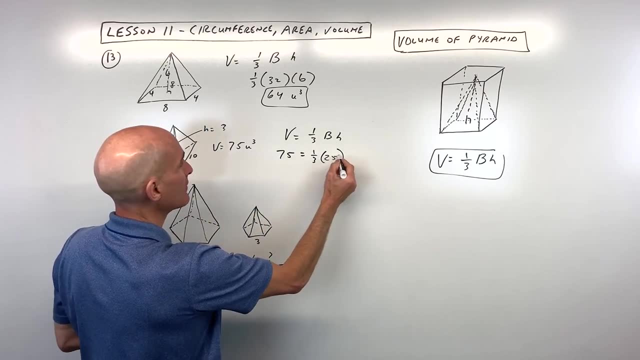 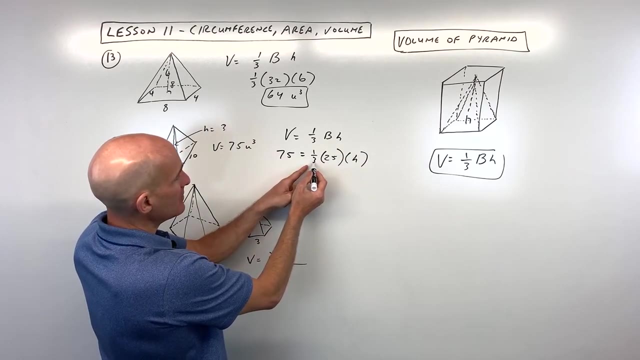 for v, we've got one-third. the base is a triangle, so it's five times ten times a half, remember. one-half base times height. so that's 50 times a half is 25, and then the height we don't know. so let's just leave that as h. so if we multiply both sides by three, that's going to give us 225 equals 25 h i. 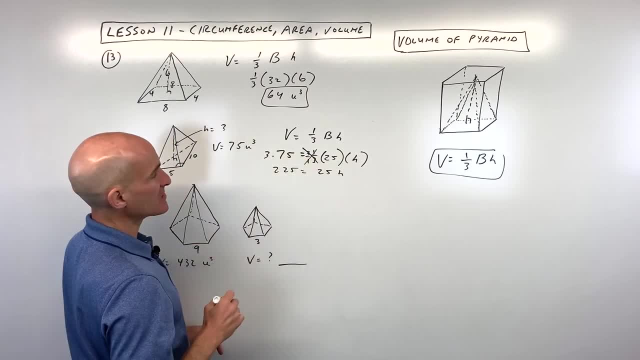 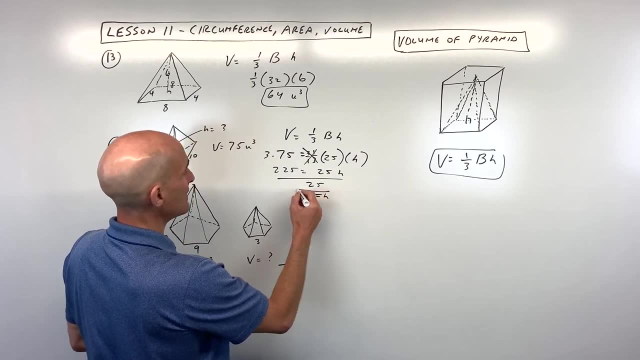 just multiply by three, because these are going to cancel out. and now, if we divide both sides by 25, you can see that goes in nine times. so our height is going to be nine units, and then for the next one number, 15. this is interesting, these two. 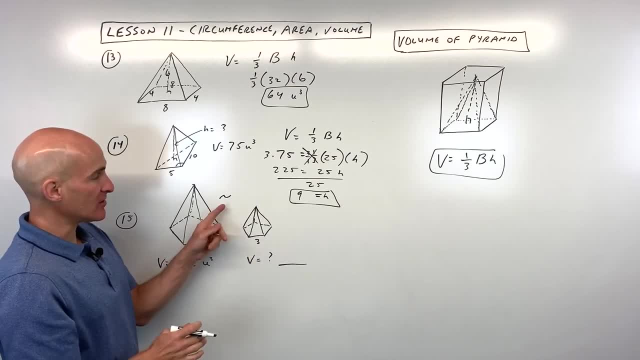 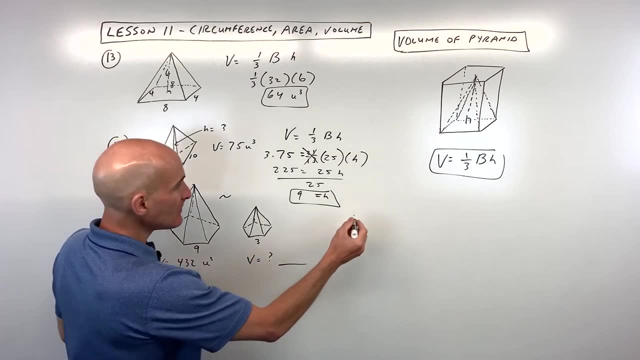 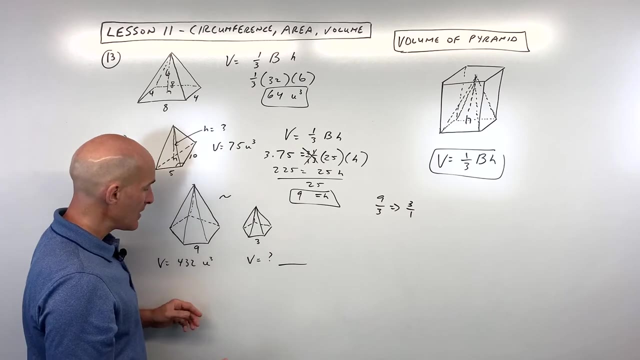 pentagonal pyramids are similar, okay, similar, and we know the scale factor is the ratio of the side length. so nine to three, nine to three, which reduces to three to one. okay, so if you divide the numerator and denominator by three. but when you look at the scale factor, that's the ratio of 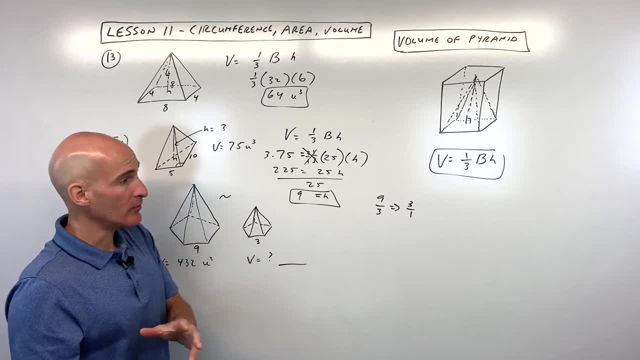 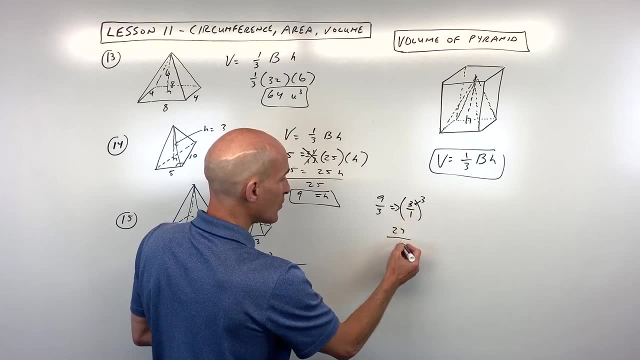 the side lengths or the perimeters. but when you compare the volume volume is the scale factor cubed. so three cubed is three times three times three. one cubed is one times one times one. so the ratio of the volumes is going to be 27 to one. notice: this is the larger volume to the smaller. 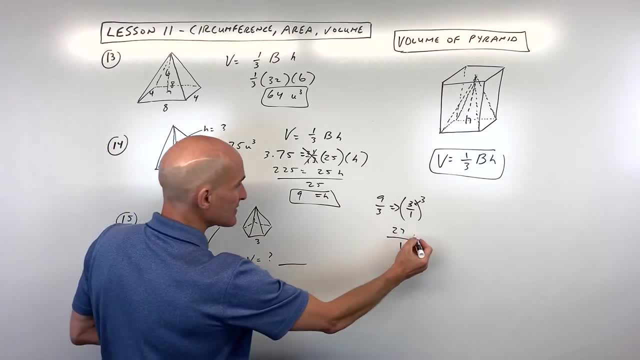 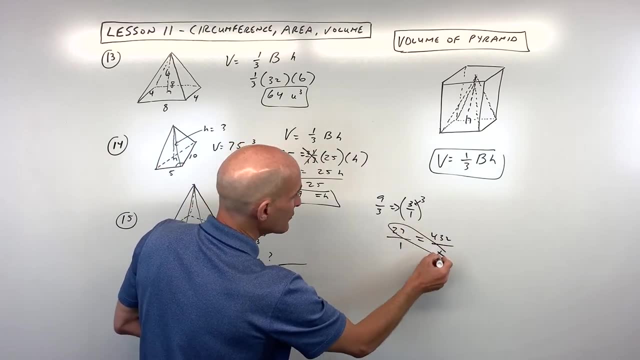 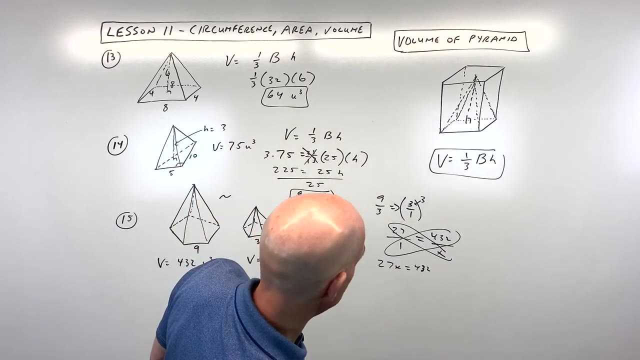 volume, or in this case the left to right. so we want to keep that the same here. larger to smaller, larger to smaller. 32 to x. now all we have to do is cross, multiply and solve. so we have 27 x equals 432 if we divide both sides by 27. 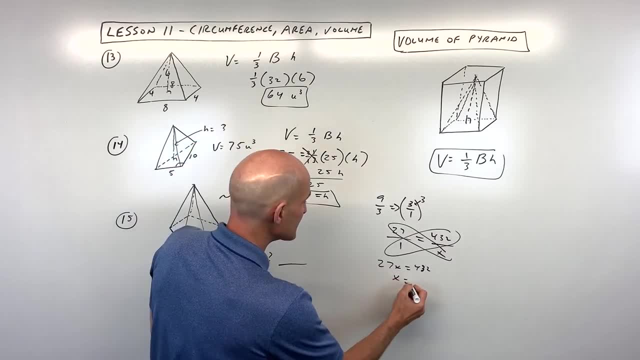 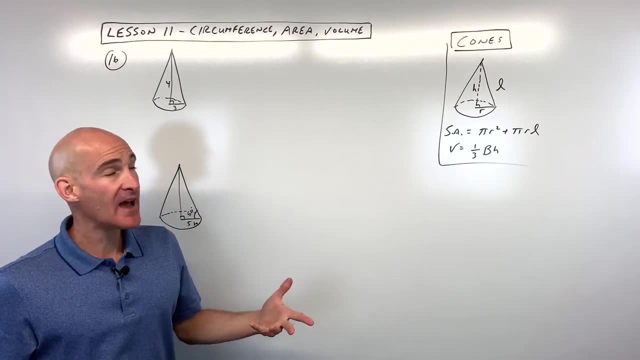 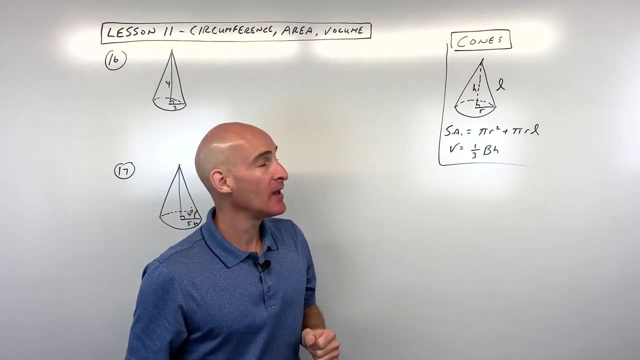 you can see we're getting 16 units cubed for the smaller volume. okay, for cones. now we're going to find the surface area in the volume. so surface area means like the outer surface, like if you're painting the cone you'd have to paint the outer surface of the cone. 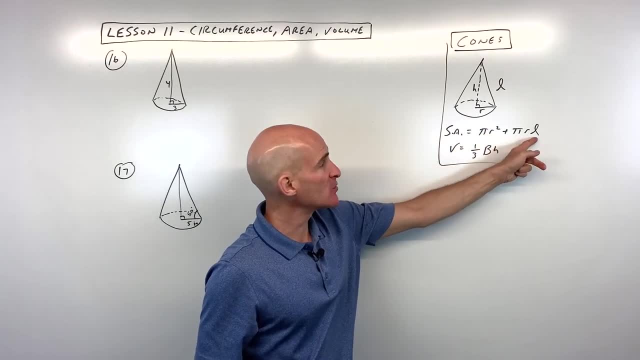 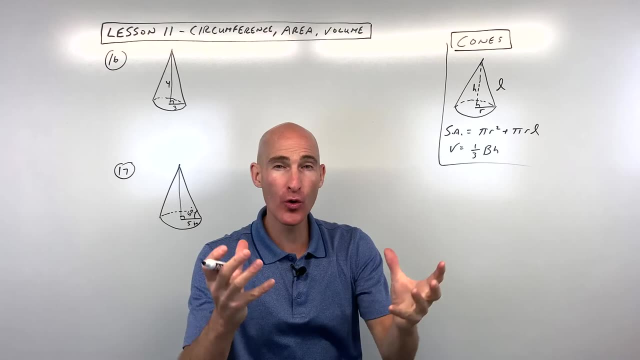 the bottom, which is a circle, pi r squared, and then this is what's referred to as the lateral area. it's the area of the sides, not the base, and that's going to be pi? rl, and if you add those together, you get the total area of the surface. for volume, though, it's just like what we talked. 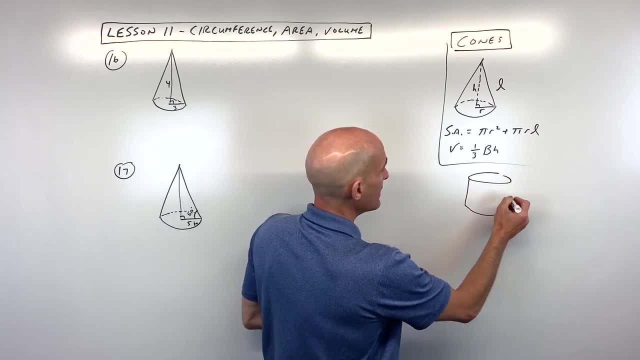 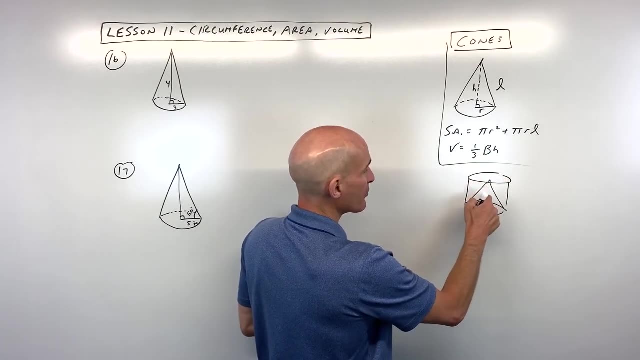 about when we talked about with the pyramids. imagine if you had a cylinder. the volume of a cylinder is, uh, area of the base times the height, but you could actually fit three of these cones in the same in the cylinder with the same base and the same height. 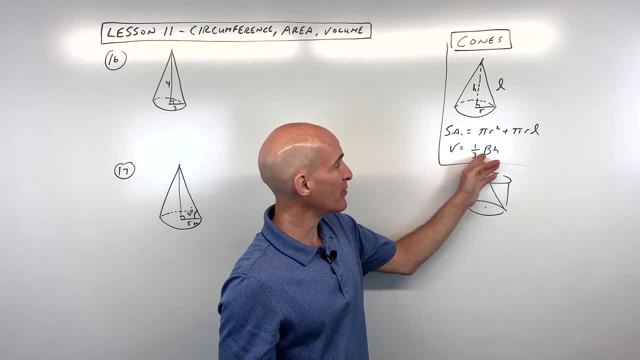 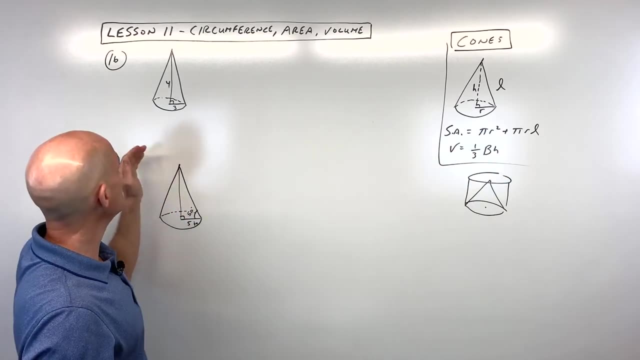 one of the cones is only going to take up one-third of the volume, so it's just one-third of the area of the base times the height. so this formula you're familiar with, this one's a little bit newer. let's do a couple examples: one easy one, one a little bit more challenging. so let's start off. 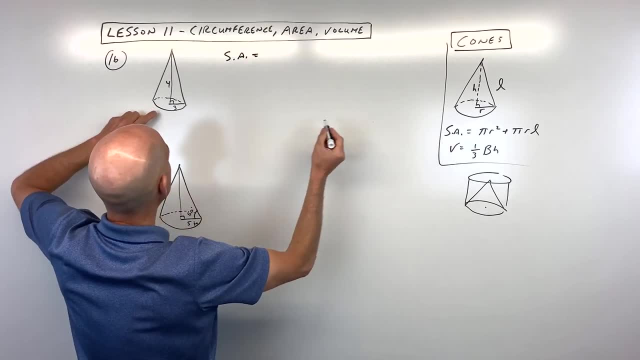 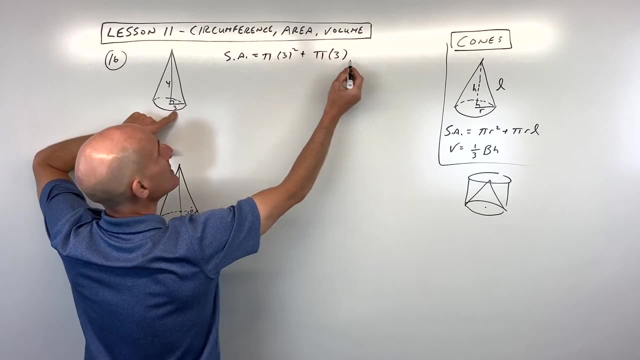 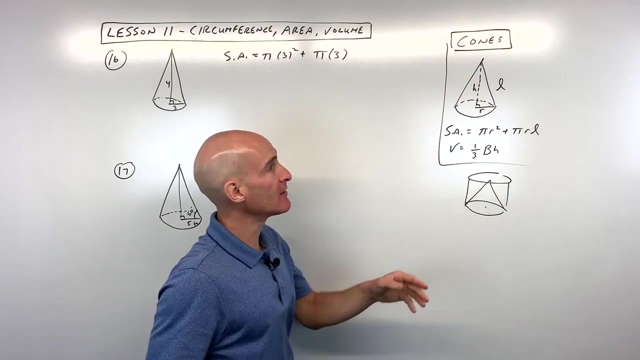 by finding the surface area. so we've got pi r squared. so it's going to be pi times three squared, plus pi times the radius times the l, which is the leaning height. that's our slant height, not h. h is the overall height. that's what we use when we find the volume l for leaning right, or you can think of it as leaning. 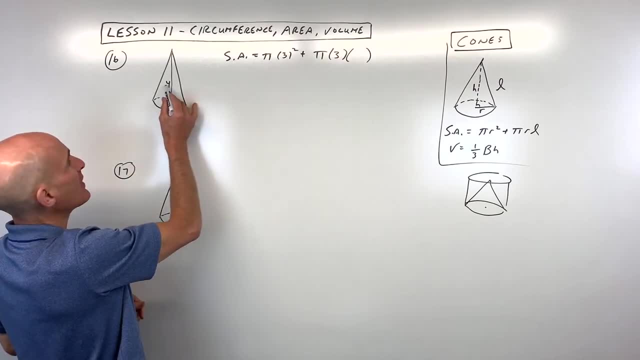 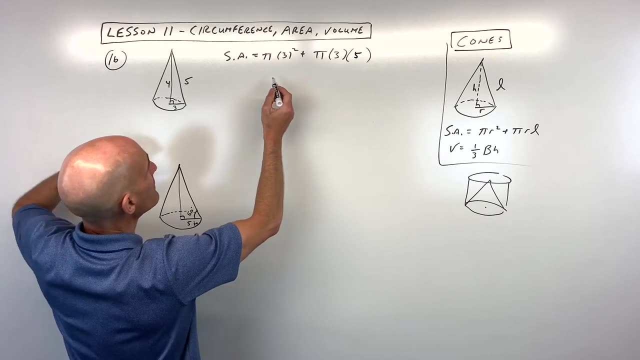 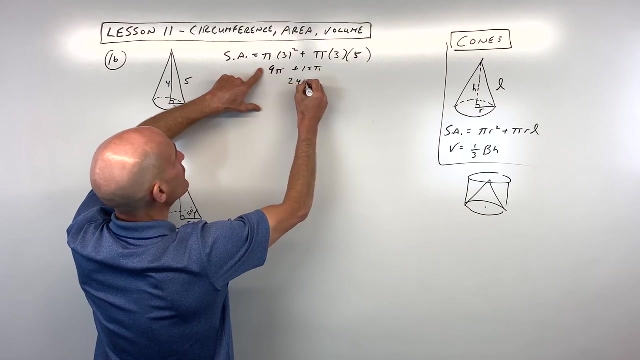 that's the slant height. now notice that this is a right triangle. we could do pythagorean theorem or, if you remember your pythagorean triples, it's a three, four, five pythagorean triple. so three squared is nine. so this is nine pi. this is 15 pi, which equals 24 pi units squared for area for. 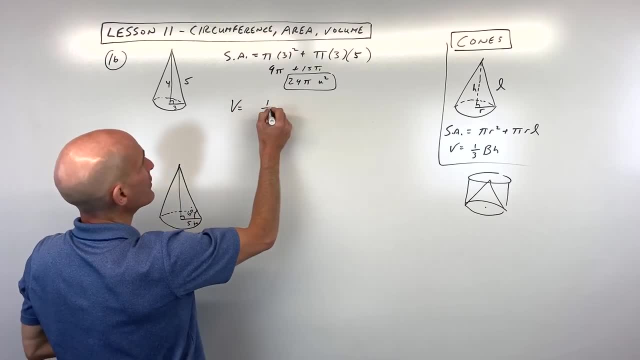 volume, though we want to find the one-third area of the base times the height. so we're going to find the one-third area of the base times the height. but remember the base is a circle, so that's a pi r squared times the height, and here we have the radius is three squared times, not the leaning. 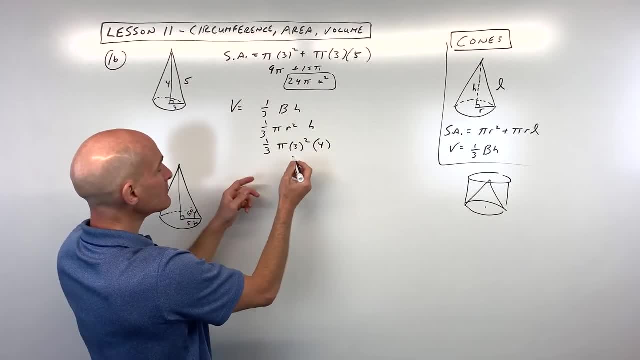 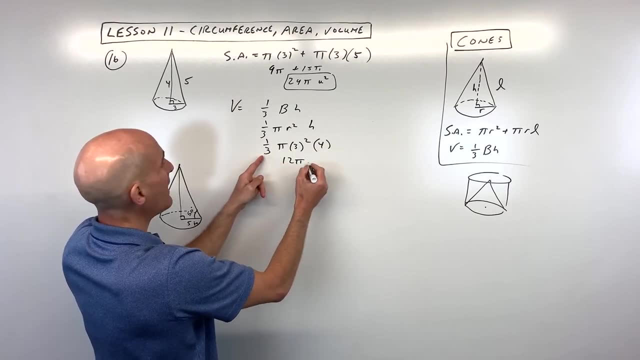 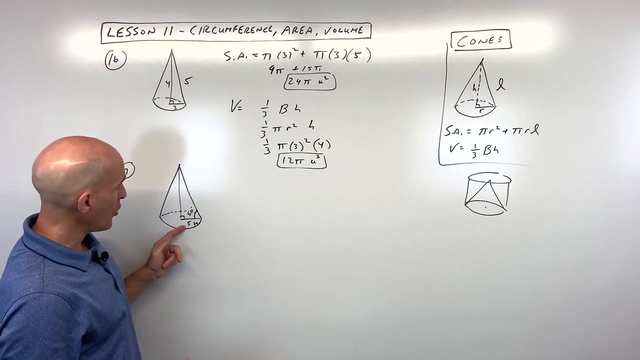 height five, with this perpendicular height which is four. so three squared is nine. nine divided by three is three. three times four is twelve. this comes out to twelve pi units cubed for the volume. now a little bit more challenging one. here we have a cone, the radius is five, and then see this angle, here is 50 degrees. so we don't know the height and we 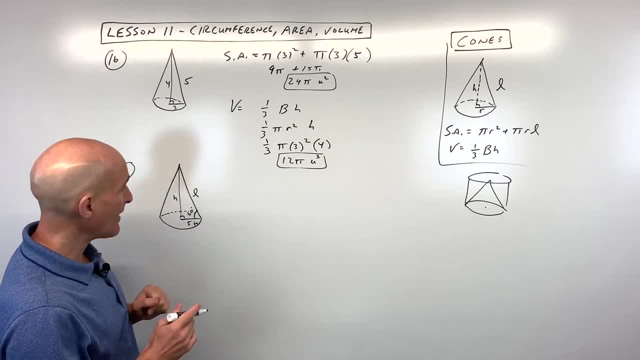 also don't know the slant height, so we have to do some trigonometry. so let's start off by finding the, the slant height and the overall height. so let's let's do the overall height first. so what trig function ties together this angle, this side and this side? well, we have opposite and adjacent. 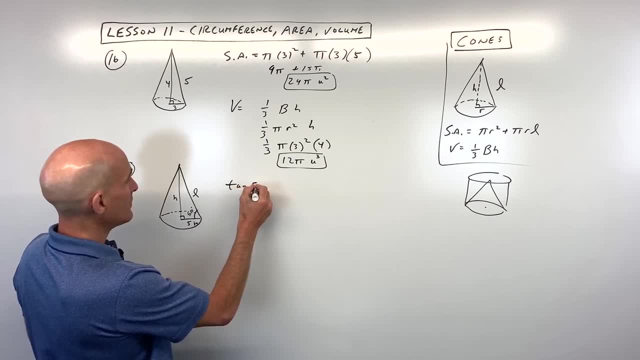 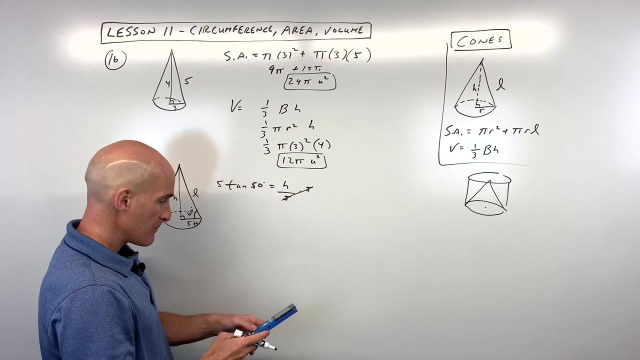 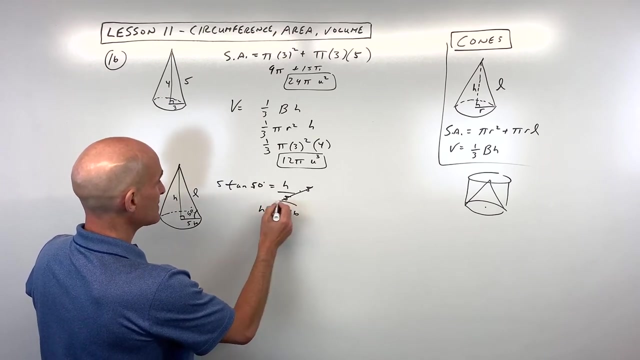 that's tangent. so we can say the tangent of 50 degrees equals opposite over 50 degrees over adjacent. if we multiply both sides by five, you can see that the height equals five times the tangent of 50, which is 5.96. so let's just write that down: 5.96, and then the slant height, which. 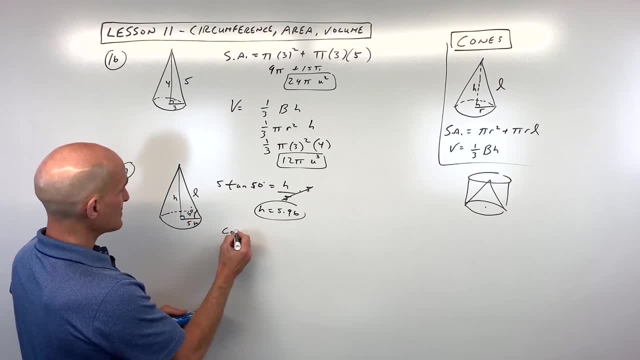 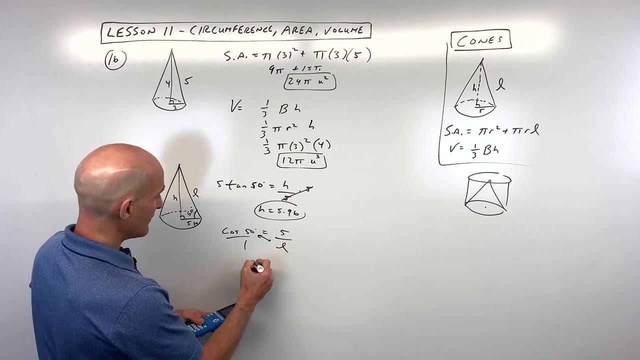 trig function ties together adjacent and hypotenuse, that's cosine. so we have the cosine of 50 equals adjacent over hypotenuse. we can cross, multiply or interchanges on the diagonal. so we have 5 divided by the cosine of 50. that's giving us 7.78 for our slant height. okay, so now let's find the surface area. so surface area is pi. 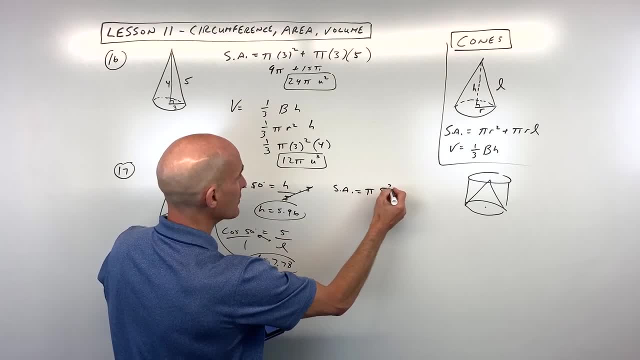 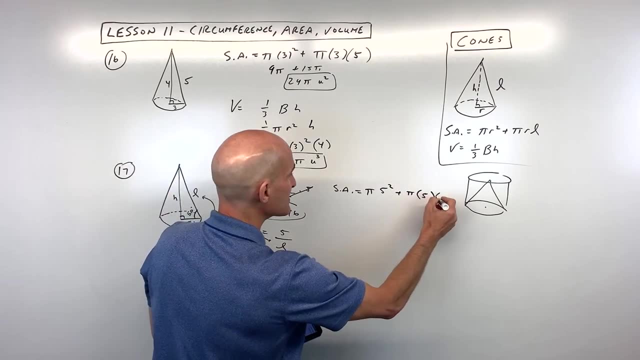 r squared. that's the base. so it's going to be pi times 5 squared, plus pi r l, which is going to be- we figured out- seven point seven, eight, okay, so let's do that. so i'm going to get a decimal approximation. so that's pi squared. that's. 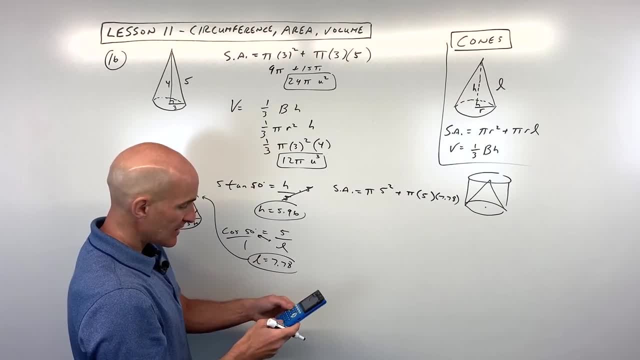 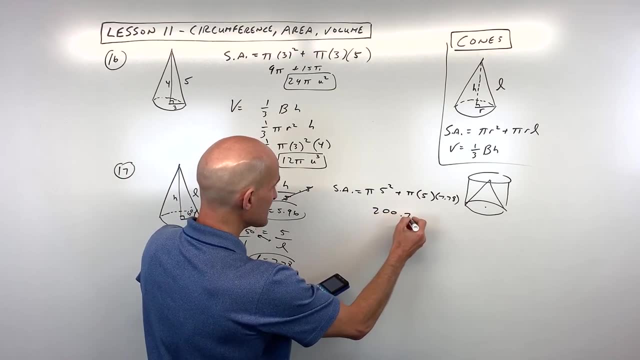 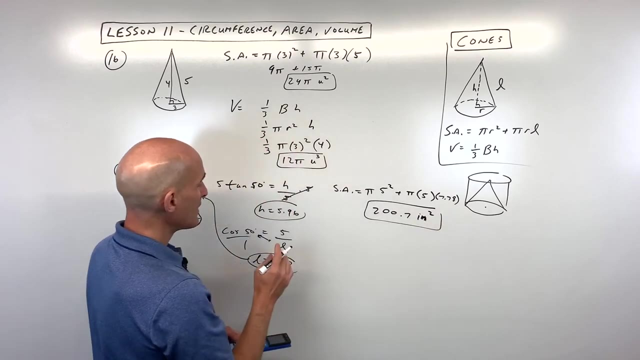 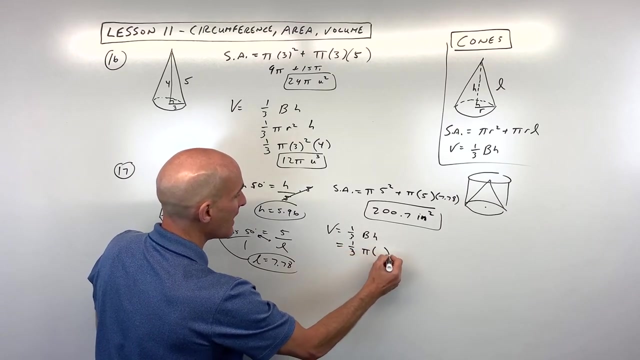 25 pi plus five times pi times 7.78, so it's about 200.7 units squared. in this case it's inches squared. okay, now for the volume. this is a little bit easier. it's just one third area. the base times the height. the base is a circle, so that's pi r squared. 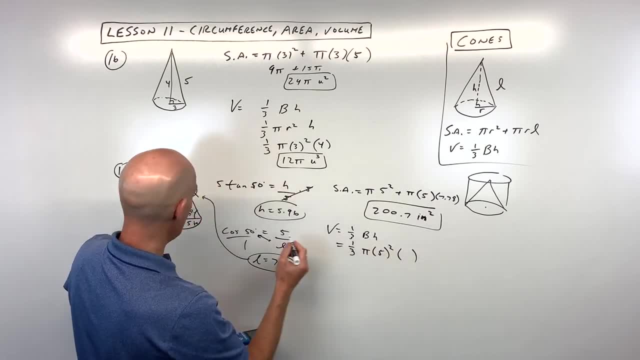 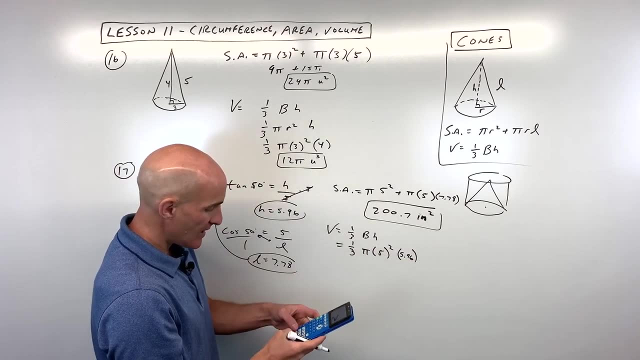 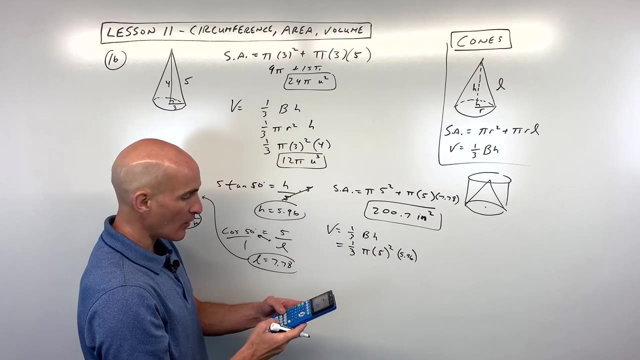 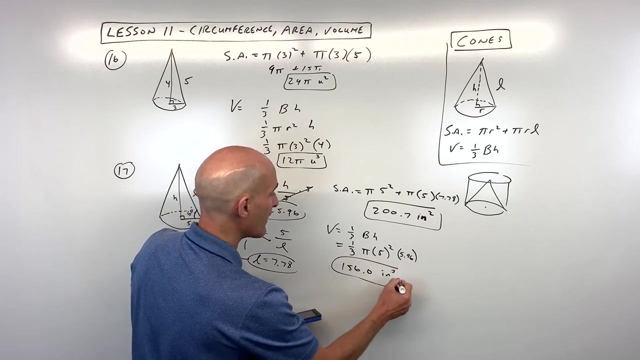 times the height, the radius is five. the height we figured out was 5.96, and if we multiply that together, let's see five squared is 25 times pi, times 5.96, and then all divided by three, or you can multiply by one third. so here i'm getting 156.0 inches cubed for volume. okay, let's talk. 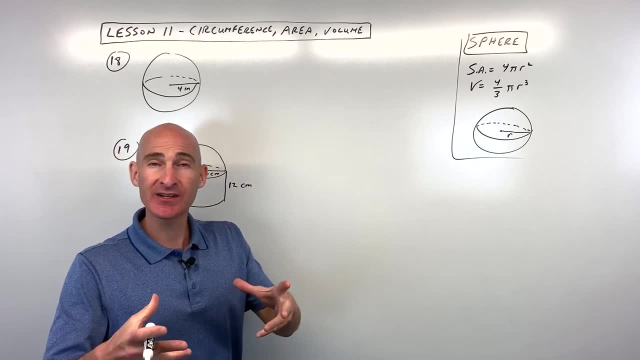 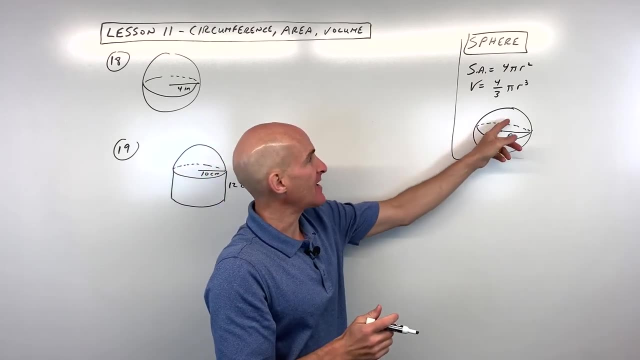 about spheres now. so what exactly is a sphere? well, it's kind of like a sphere. it's kind of like a circle in three dimensions. you know, you're looking at this basically like this ball, and it's a set of points that are equidistant from a given point, which we call the center. 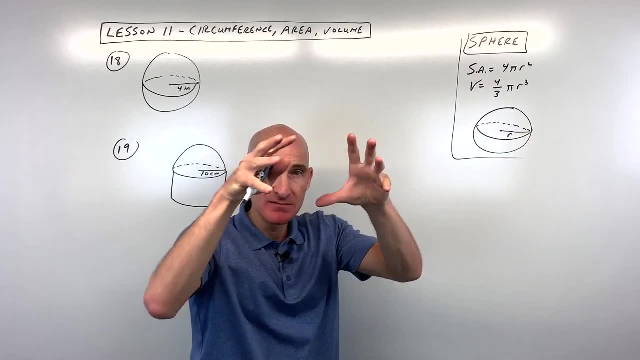 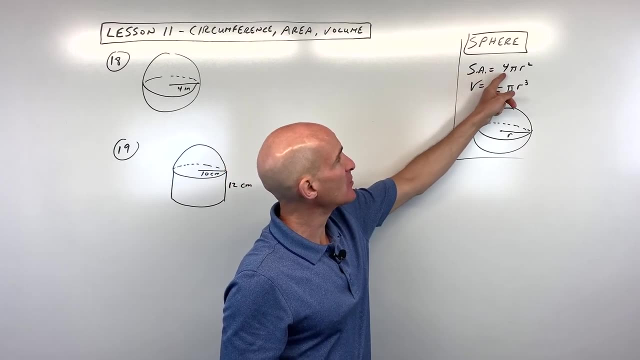 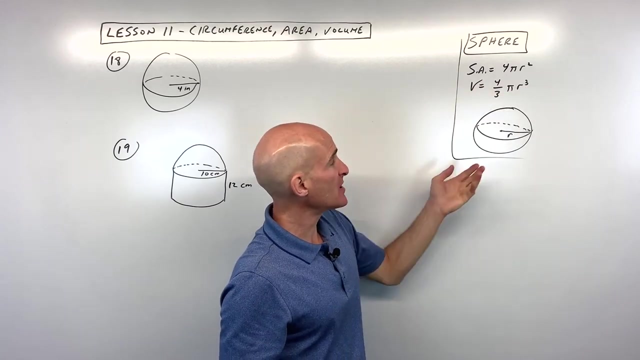 and the distance from the center to any point on that outer edge of the sphere is the radius. so there's two formulas uh: surface area and volume. surface area equals four pi r squared and volume equals four thirds times pi r cubed, and so the only dimension really is the radius that we need. 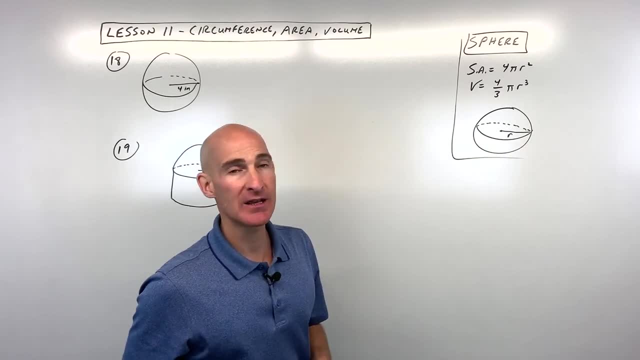 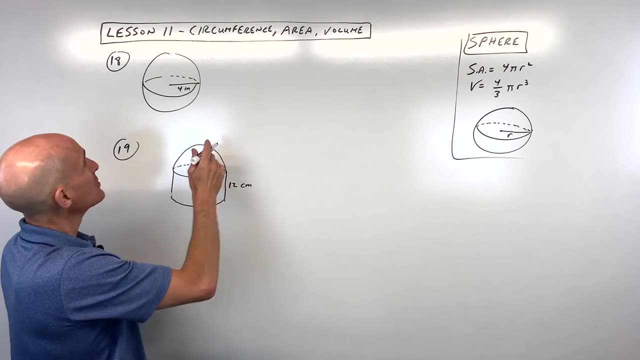 attention to. sometimes they give you the diameter but you can cut it in half to find the radius. so let's look at a couple examples: one where you're just working with the surface area and volume of the sphere and then a composite shape. so here for number 18, the surface area: 4 pi. 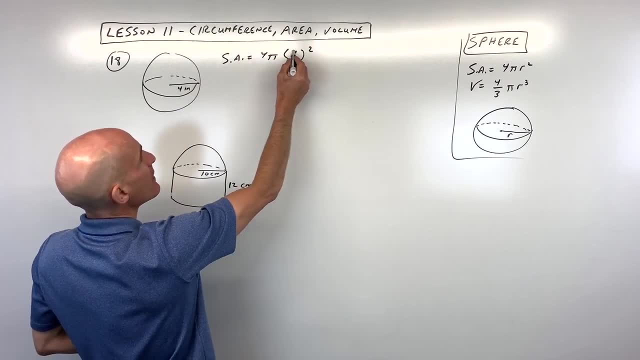 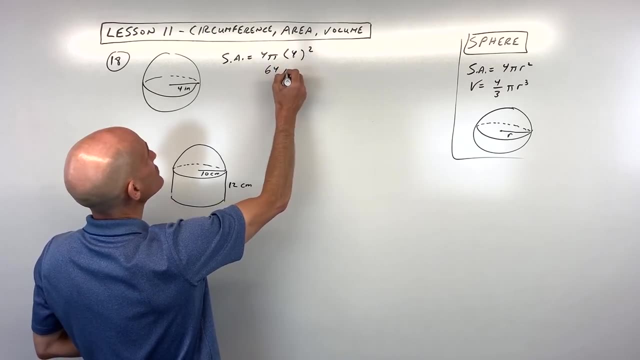 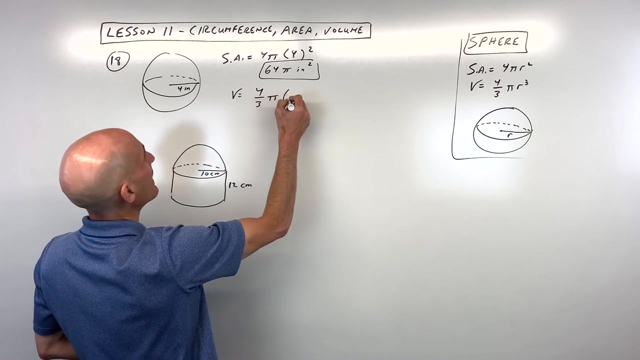 times the radius, which is 4 squared, remember your pemdos. so, parentheses, exponents, multiplication: 4 squared is 16 times 4 is 64, so that's 64 pi inches squared, and then for the volume, we have four thirds pi r cubed. in this case the radius is 4, so 4 cubed is 64. 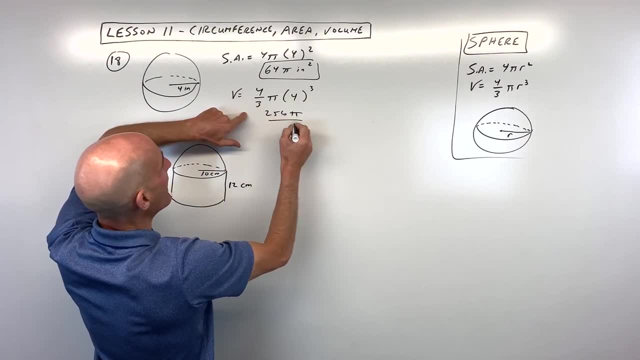 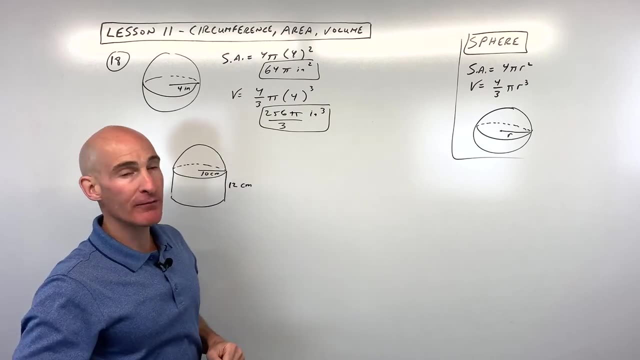 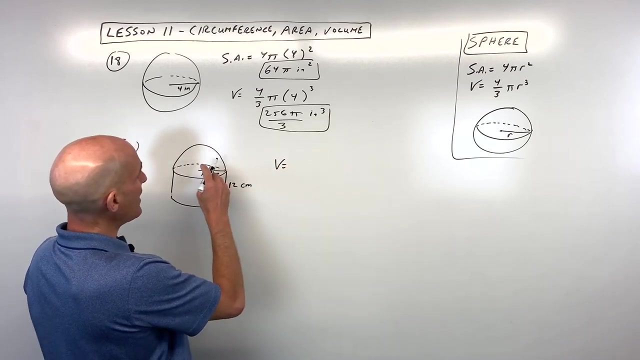 times 4 is 256 pi over 3 inches cubed. so this is an exact answer. you can put 3.14 in for pi to get a decimal approximation. for number 19, though let's look at the, let's look at the volume first. so the volume: we have a cylinder here and then on top the cylinder. 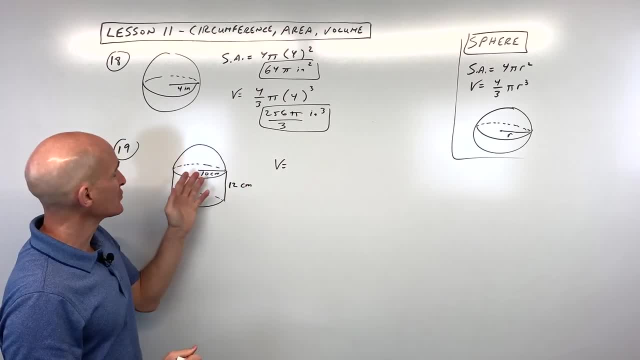 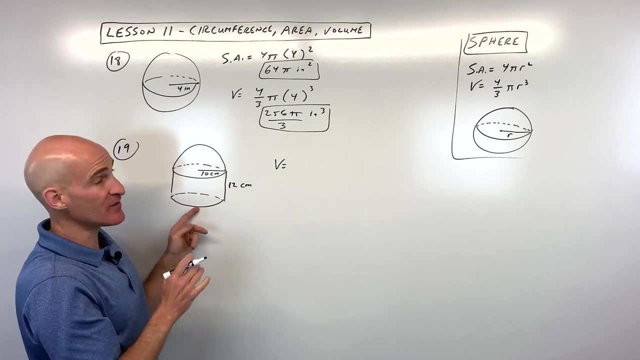 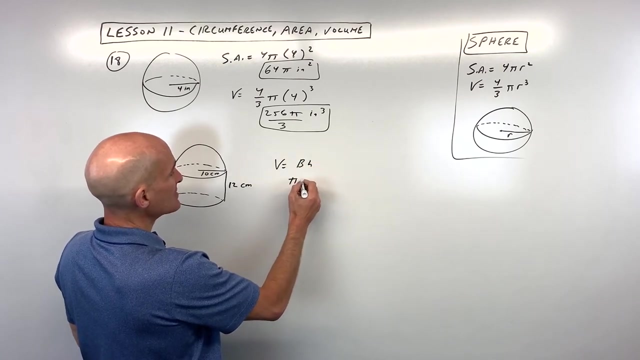 we have like half a sphere right, so it almost looks like kind of like an observatory of some sort. so the volume is the volume of the cylinder plus half of the sphere. so let's see, the volume of the cylinder, we know, is area of the base, times the height, which in this case the base is a circle. so 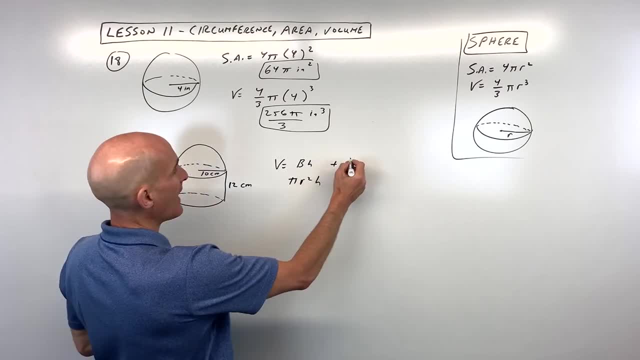 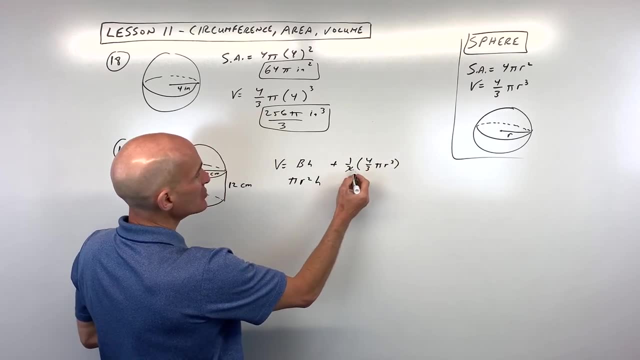 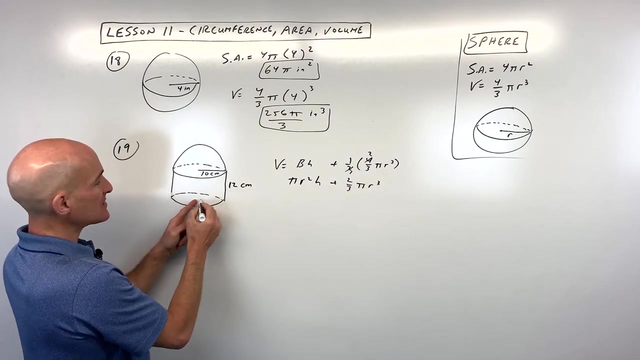 we have pi r squared times the height, plus we have half of a sphere, so it's going to be one half four thirds pi r cubed here, the two and the four you can do. so it's really going to be like plus two-thirds pi r cubed, okay. so in this case the radius is 10. 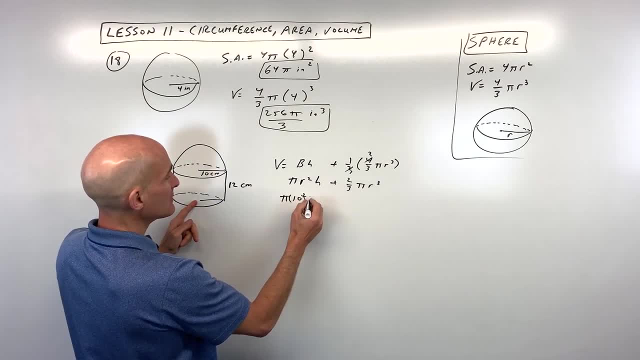 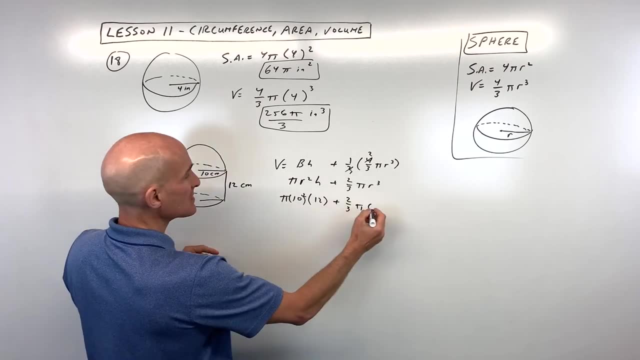 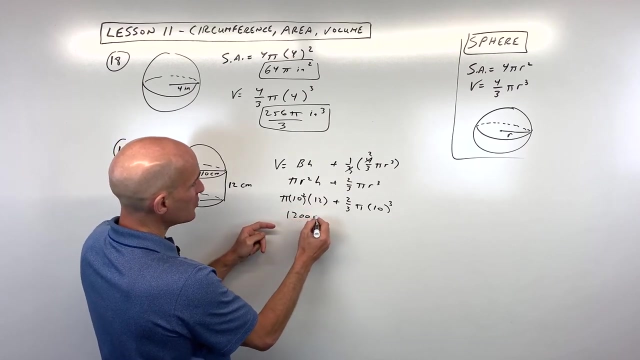 so it's going to be pi times 10 squared, times the height, which is 12, that's for the cylinder, plus two-thirds pi times the radius, 10 cubed. okay, so let's see. so 10 squared is 100 times 12 is 1200. so this is 1200 pi. here, 10 cubed is a thousand. 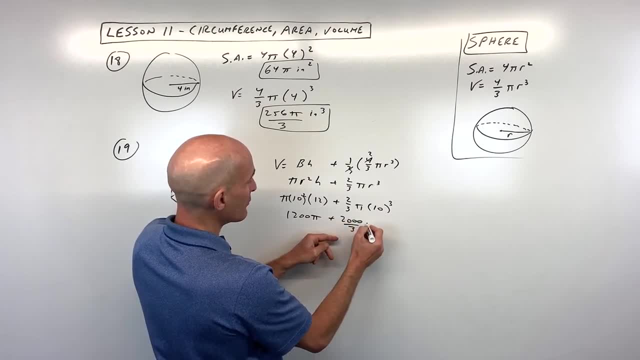 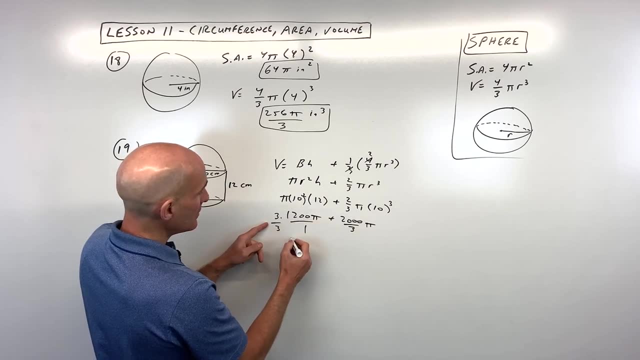 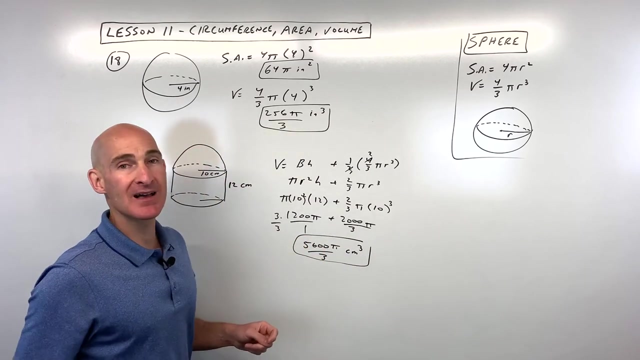 uh times two-thirds, that's going to be 2000 over three pi, and we could get common denominators here. let's multiply the top and bottom by three, that's 3600 uh over three. plus two thousand over three is how much that's uh 5600 pi over three centimeters cubed. so that's the. that's the volume of the composite. 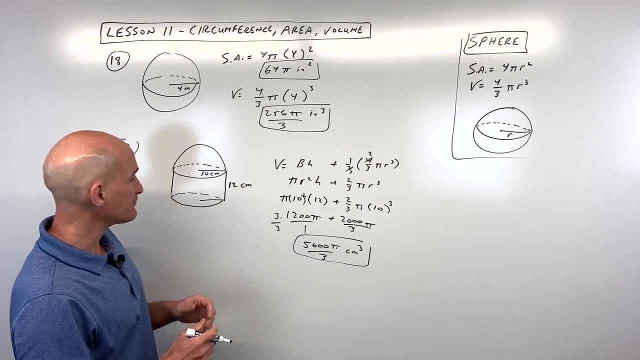 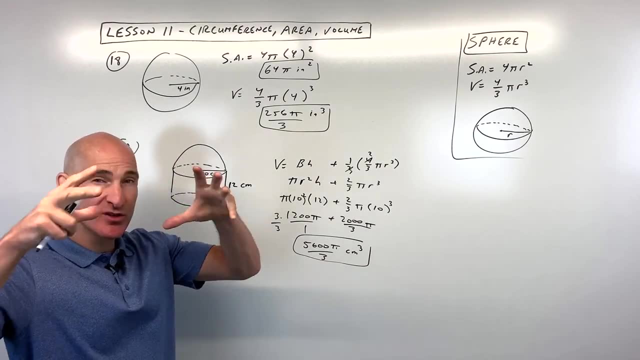 shape. okay, now surface area, a little bit more challenging. we have to find the area of this circle. we don't find the area of this circle because it's on the inside surface area. we're just finding the outer surface. so let's find the area of this circle first. so we've got the area of the circle. 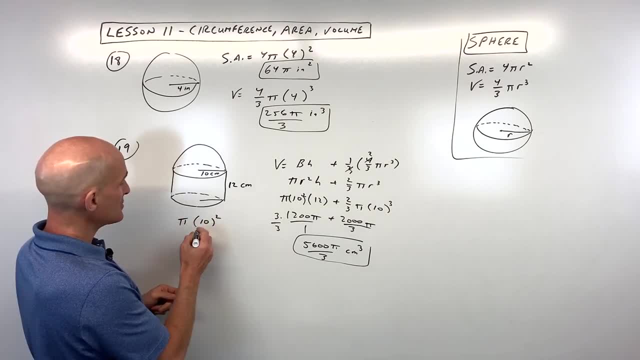 which is going to be pi times 10 squared. so this is 100 pi. okay, now we're going to find the- let's find the surface area of this sphere. but we're going to do, instead of 4 pi r squared, we're going to do 2 pi r squared, because it's half. so that's going to give us 2 pi times 10 squared. 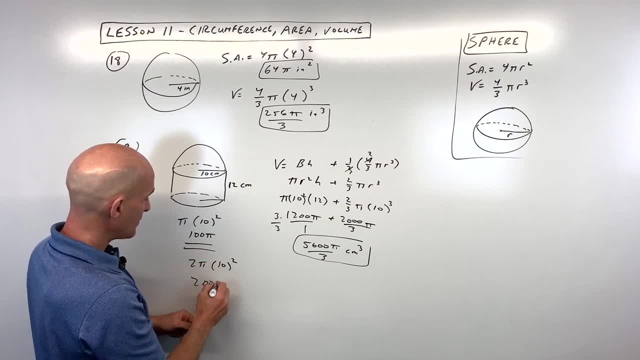 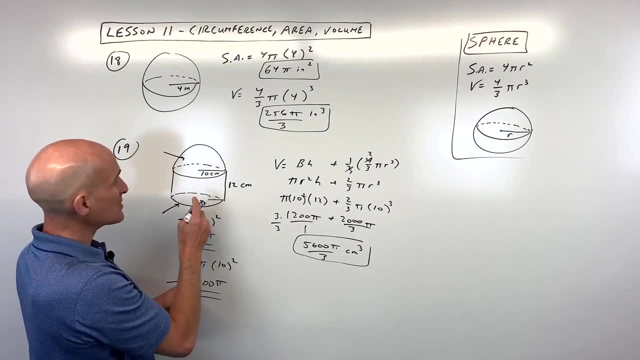 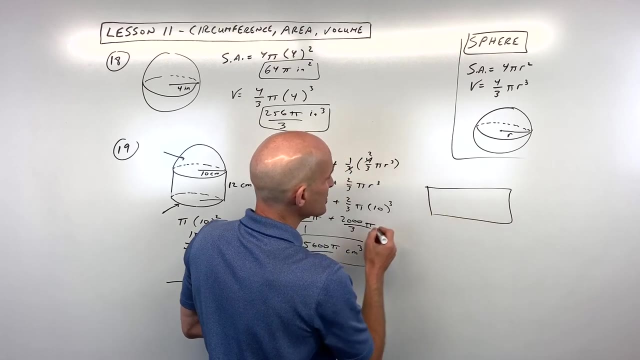 so that's 100, 200 pi. okay, so now we found this. we found that now we just have to find the what's called the lateral area of the cylinder. now, this one we haven't talked about. you probably talked about this in another course when you did like pre-algebra. but if you unroll this, like if you-